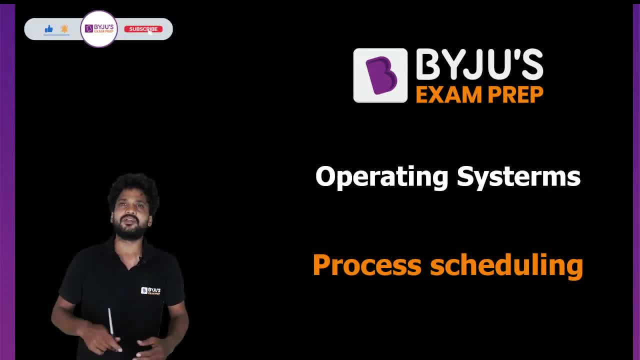 Hi, hello students, Welcome back to India's most comprehensive online learning platform, ByJuice exam trip. This is Anil Prasad Swarampudi and in this session I'm going to take up a few PYQs on inter-process communication. especially when it comes to the inter-process communication, It's a beautiful topic in entire operating system, Operating system. you know, if you ask me which is the most beautiful topic, which is the most interesting topic, that is inter-process communication, because we can actually understand the depth of the operating system. 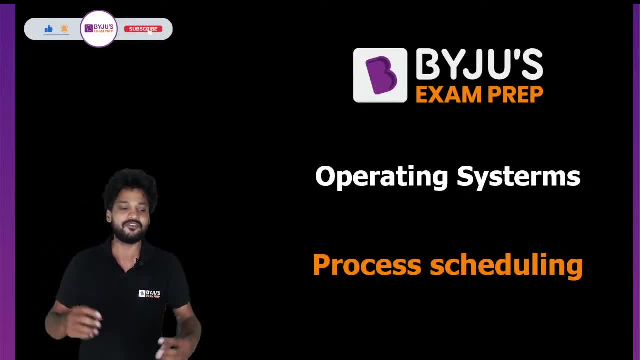 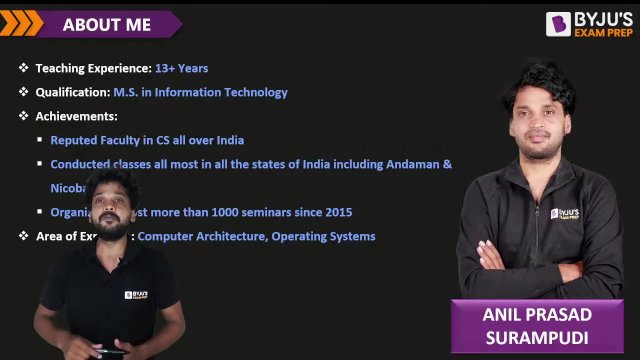 Inter-process communication, which is going to give us a lot of complexities. Okay, so let us start our session on inter-process communication. PYQs- Hi- accelerate inter-concepts. Yeah, very good evening. May I know what's your name so that you know I'll be able to communicate with directly with your name. So let me start the class right away. So this is Anil Prasad Swarampudi. once again, for all of you guys, I don't need my introduction because you know for past. 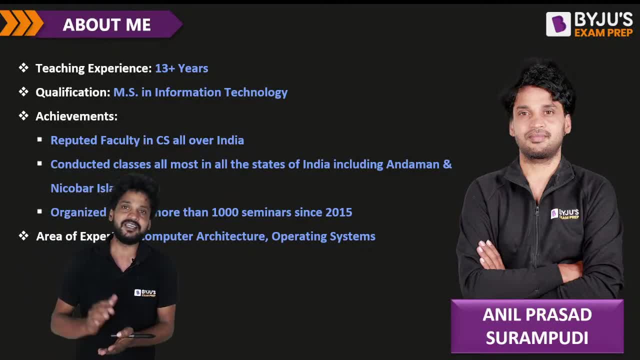 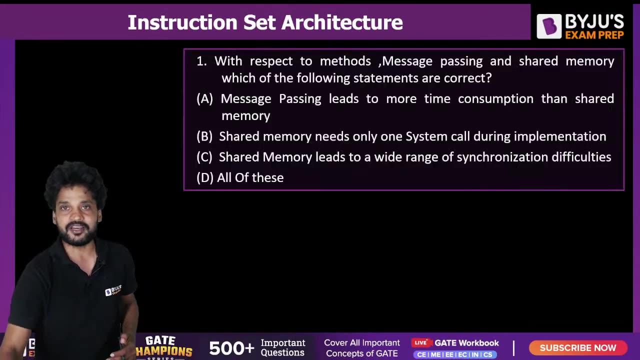 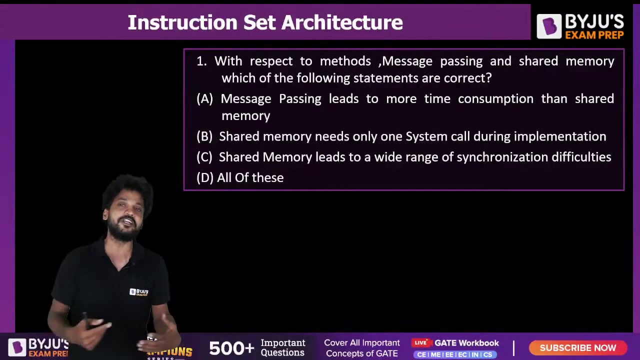 six or seven months you'll be. you are continuously with me. Once again, this is Anil Prasad Swarampudi. I do have 13 plus years of experience and I taught everywhere in India in gate priming, So let us start this session on inter-process communication. The first question is on your screen. First of all, before I take you people into inter-process communication, first of all let us understand something. What is this concept of inter-process communication? Okay, Hi, Abhidhi Villas, Good evening. Yeah, right now. 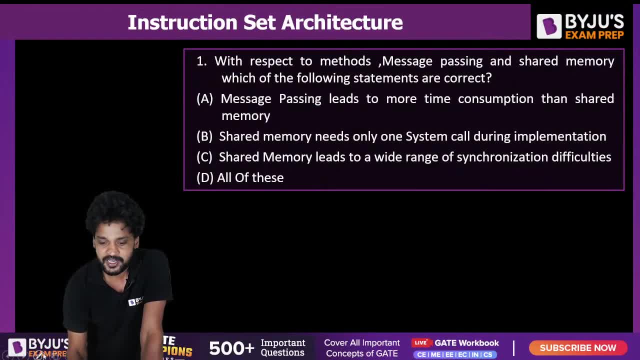 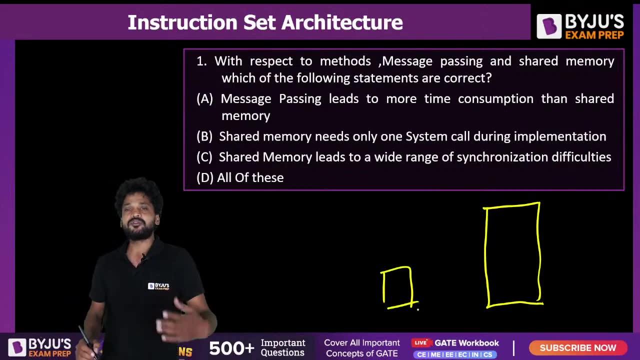 when you talk about inter-process communication, understand something. I will start with a simple note. Okay, I will start with a simple note. Of course I will take an example of main memory and a CPU. Okay, where all the processes will get stored, where all the programs will get stored. all the programs of a computer system will only get stored in the main memory. Is that fine? We'll only get stored in the main memory, All the process, no matter what it is. 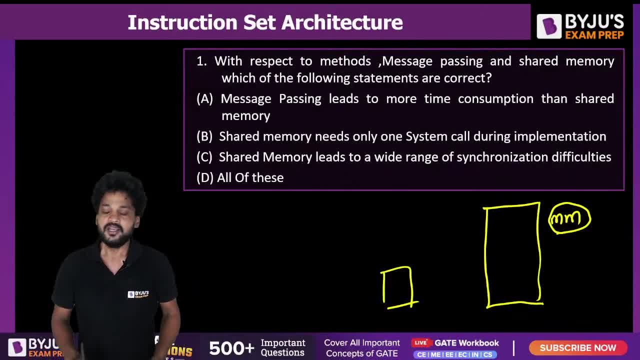 is every process is going to only get stored in the main memory the moment a process comes into the main memory- let us say a process v1 arrives into the main memory. the moment a process arrives into the main memory, operating system will treat that as an independent process. what is an? 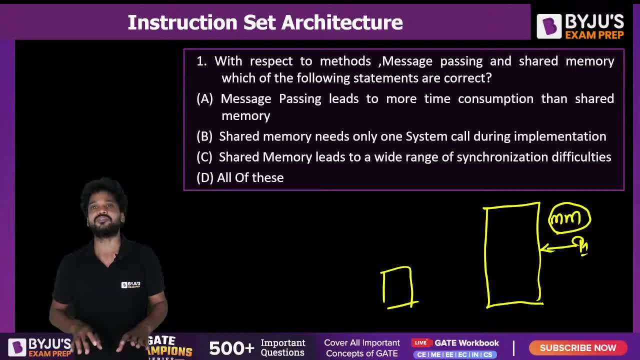 independent process. an independent process is the process to which all the resources are exclusive. that means that, in the simple words, when i am a process, i will be allotted with a few resources. all those resources are exclusively allotted to me, which are not shared to any other process. what are? 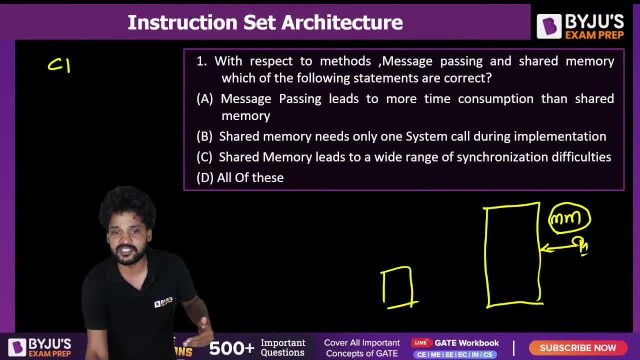 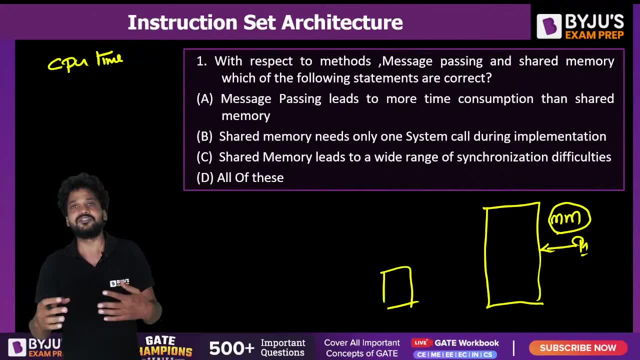 the several resources, resources which started with the. we will start with the cpu time. understand carefully all of you. i will brush up what is in the process. rather, you know what is um. what is it meant by cooperative processes? when you talk about a process, when it arrives into 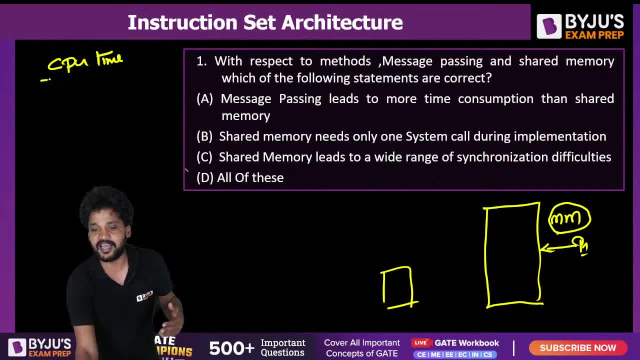 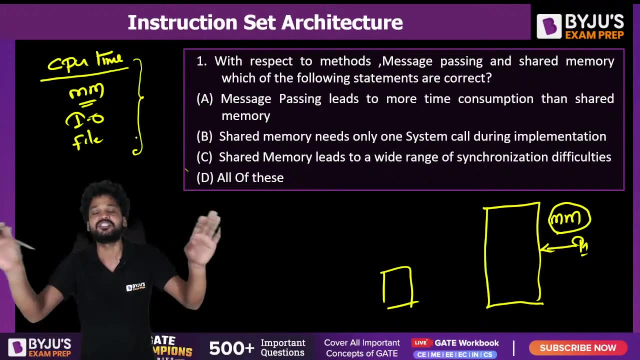 the process. that process will arrive into the moment it arrives. it will be given with several resources, such as cpu, time, memory space and io devices and a file systems. okay, several files will be allotted. understand, all the resources that are allotted to the process are exclusive. these are not shared with any other process at all. okay, the thing is this is only true for a few. 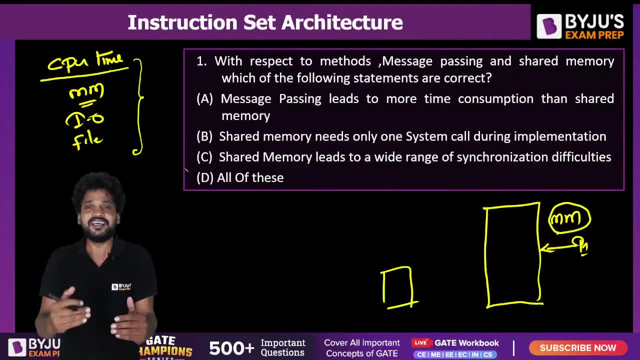 processes, but for some processes it is. there is the need of communication. for an example, i am one process, there is one more process, but we people want to communicate with each other. at that time, operating system will need to allot some shared resources. for an example, i just want to communicate with the other process. i am process a, there is process b. we want to. 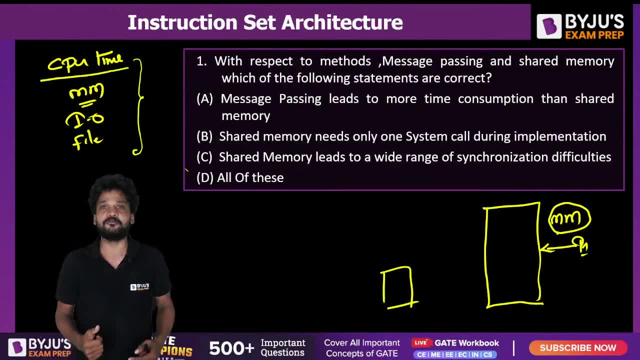 exchange the information. whenever we exchange the information, operating system can make this process communicating with each other by two means. the first one is message passing and the second one is shared memory. i hope i made it myself clear. message passing and shared memory, as you already knew, are the techniques that are going to make two processes rather more than one. 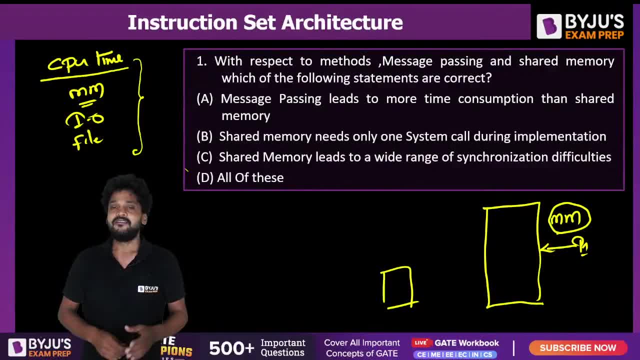 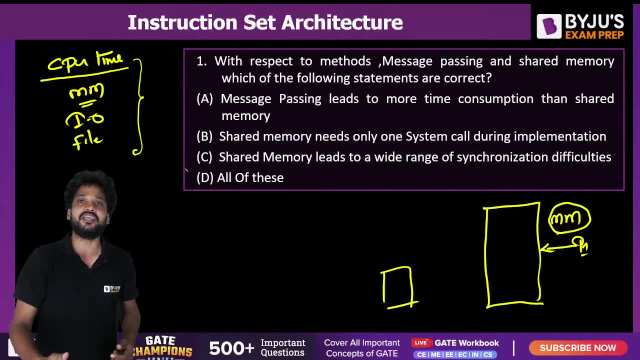 process communicating with each other by the operating system. when it comes to the message passing, it is not that best technique which can be used by the operating system, but when it comes to the shared memory, shared memory is considered to be the best technique that can make more. 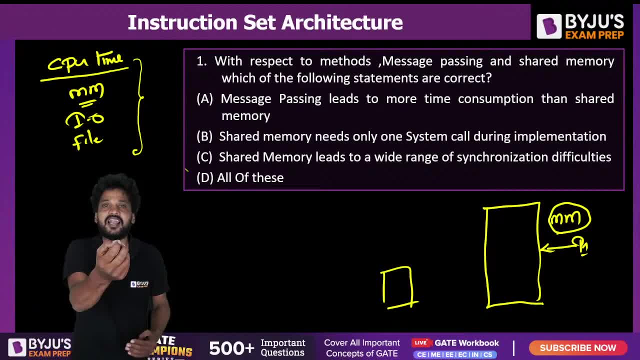 process communicating with each other, because shared memory will allow the processes communicating with each other with more data. i just want to exchange tons of data at that time. shared memory is the only way that i can come that i can um use to communicate with the other process. 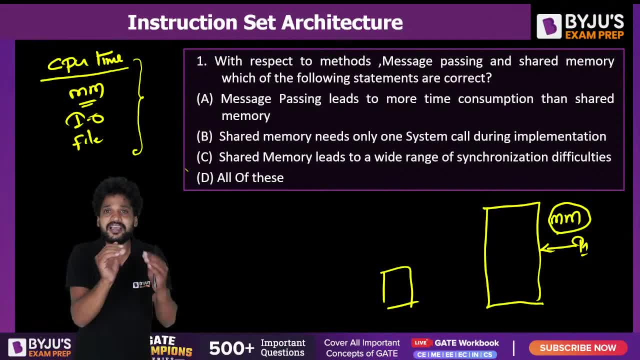 message passing will be used in between the processes to exchange the smaller information, smaller what you call the amounts of the data. now in this life, let us solve our first question. i hope all of you guys are with me. accelerate inter concepts are ability values. are you with me? 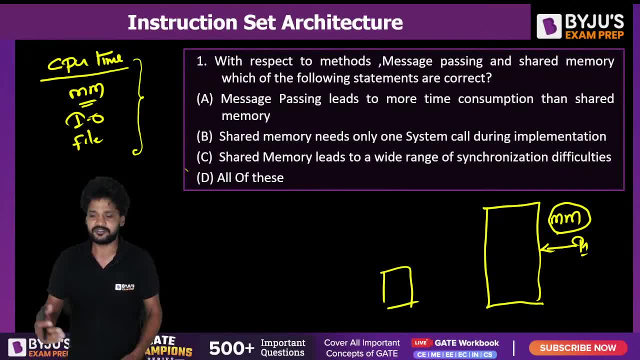 shall we discuss about our first question? say yes, i am going to give you one dimension to the inter process communication in this very um session. shall we start with respect to the methods: message passing in the shared memory? which of the following statements are correct? let us understand: there are. 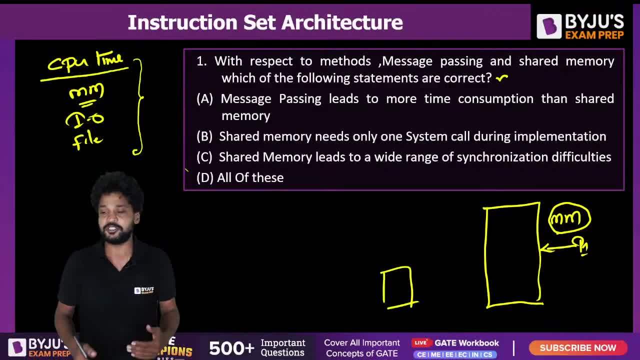 two techniques which makes the process communicating with each other. the first one is message passing and the second one is shared memory. in this same light, when you talk about a shared memory and message passing, which of the following are actually true? message passing leads to more time consumption than shared memory. this is the first statement we need to find, we need to say. 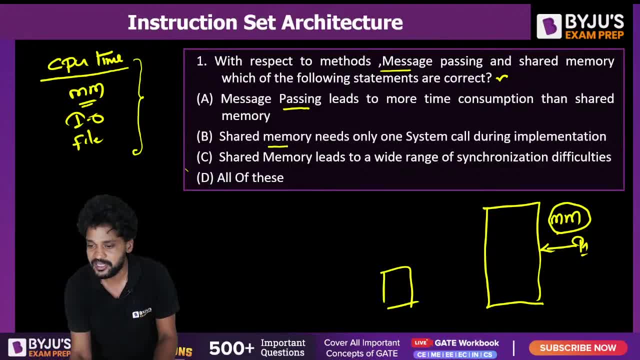 if it is true or not. second one is: shared memory needs only one system called during implementation. this is the second statement and the third statement: shared memory leads to more time consumption than shared memory. which of the following are true? message passing leads to a wide range of synchronization difficulties, ability, values. what is your pick? your pick is: 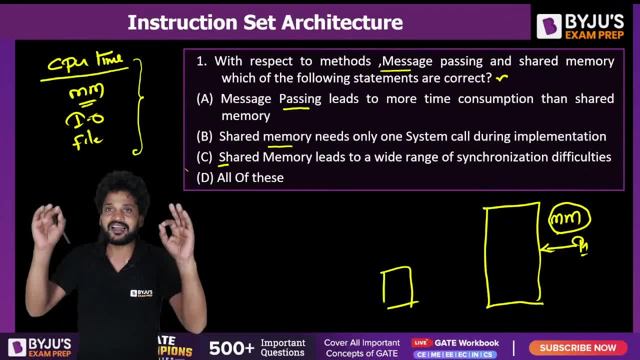 already. i think. i think you made your choice, that is, d ability values. you are perfectly spot on and you are correct. in this life, all these three options are correct. all these three statements are actually said to be correct. i will tell you. write it down somewhere when you talk about message. 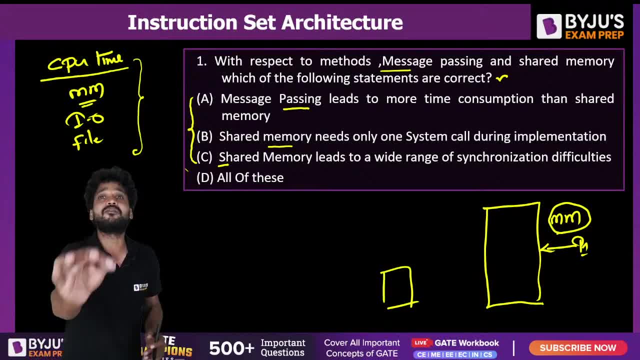 passing. two processes will be able to communicate with each other, but the second one is shared memory. which of the following are true? message passing leads to more time consumption than shared memory by means of system calls. let us say i am a process and there is one more process. i want to send a. 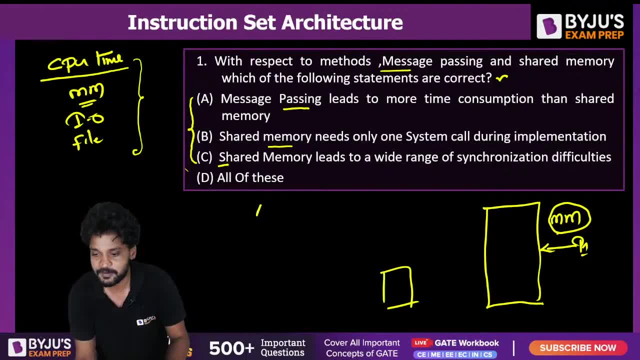 message to the another process. i would put it this here: there is a process a, there is a process b. whenever process a wants to communicate with process b, it can only be done through the system calls. hi, neil mado. sahoo, very good evening. now let us say process a wants to communicate with 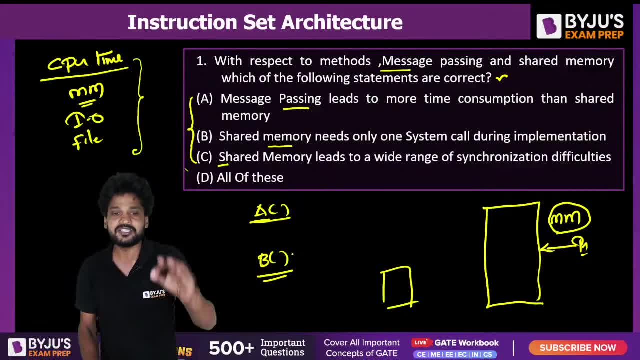 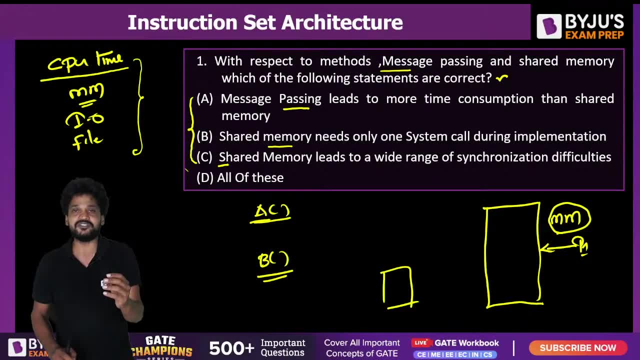 process b. it can only be achieved by means of a system call. you know what is the system call? system call is a service which is going to be provided to the process by the operating system in a kernel mode. so when process a wants to send a message to process, 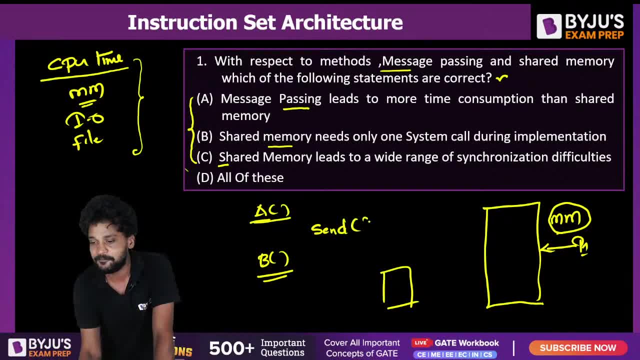 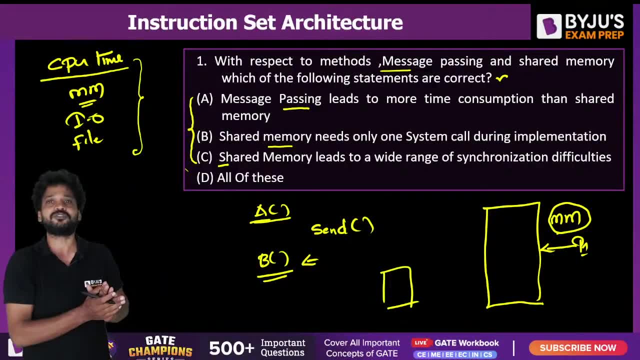 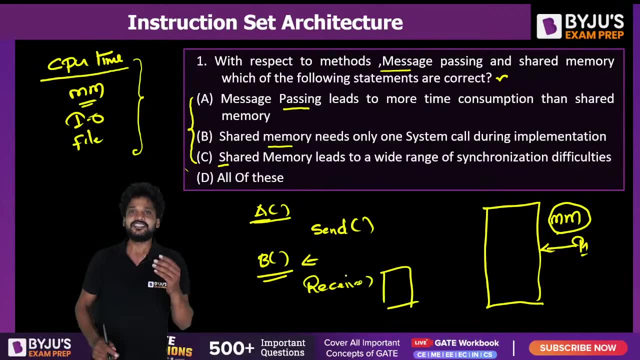 b by using a system call called send, a message will be sent to process b. at the same time process b, when it has to receive a message from past process a, it needs to execute one more system call called receive. not only the send and receive. send and receive are only the examples through which the 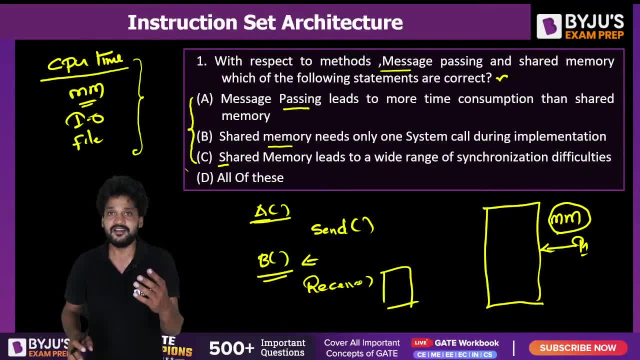 process can communicate with each other, but understand there will be numerous system calls are utilized, such as send and receive, which can make two processes rather more than one process communicating with each other. but system call can only be executed in the kernel mode. system call can only be executed in the kernel mode. 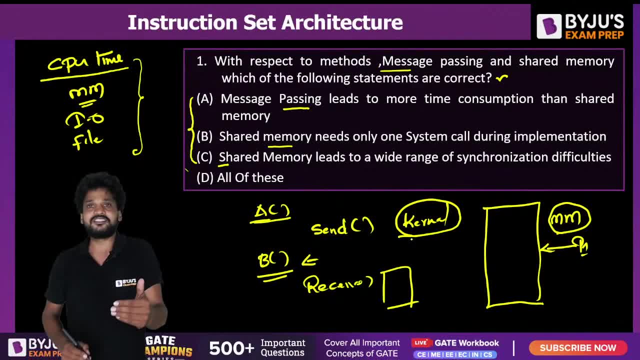 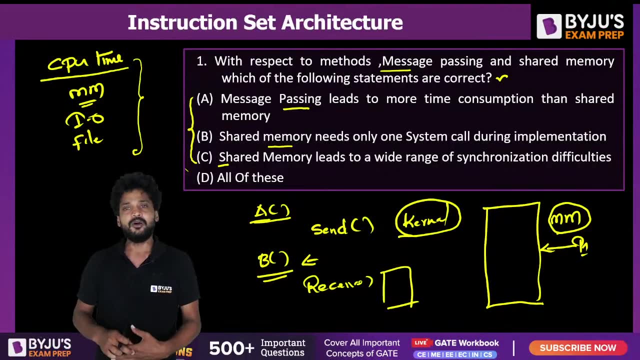 what is kernel mode? when a system call is executed, a mode will need to be switched from the user mode to the kernel mode, which will take a lot of time again, right after the system call is executed, again, mode must be switched back from the kernel mode to user mode. okay, so obviously this is going. 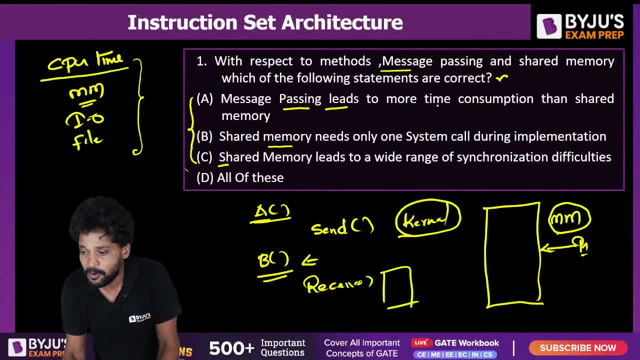 to consume a lot of time. message passing leads to more time consumption because message passing- write it down somewhere- can be achieved, can be implemented, by system calls. when a system call has to get executed, we require to execute the system call only in the kernel mode. so there will be frequent mode switches. use the mode to the kernel mode. 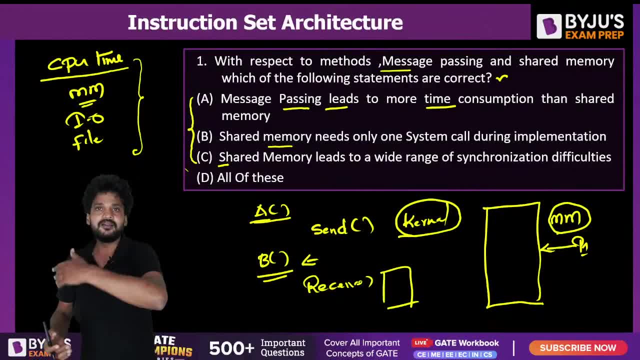 right after the message pass happens. kernel mode to the user mode. this can this. this mode switching itself is going to take a lot of time. so for this, this. this of course leads to a lot of time consumption. second thing is: shared memory needs only one time consumption. 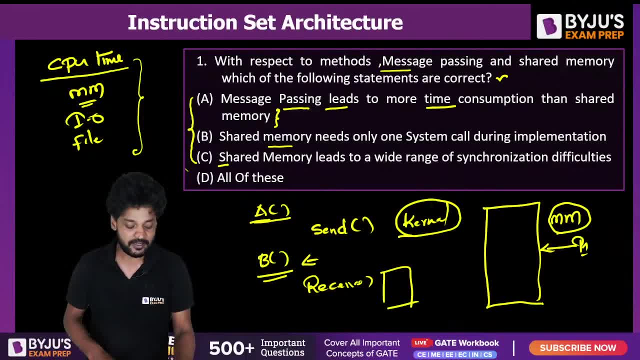 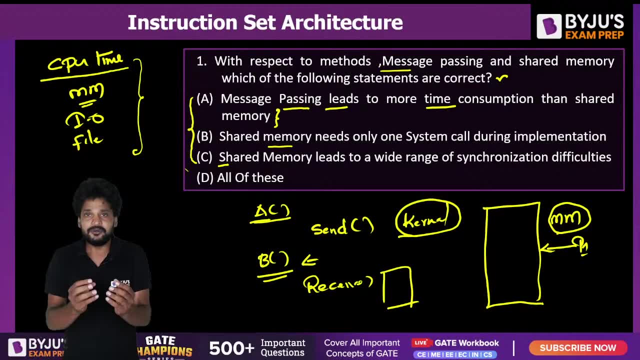 system call during implementation. this is also correct now when you talk about shared memory, understand clearly. shared memory will be used by the operating system to establish a communication in between several processes. shared memory has a lot of advantages over the- you know- message pass. what are the advantages by using the message passing? 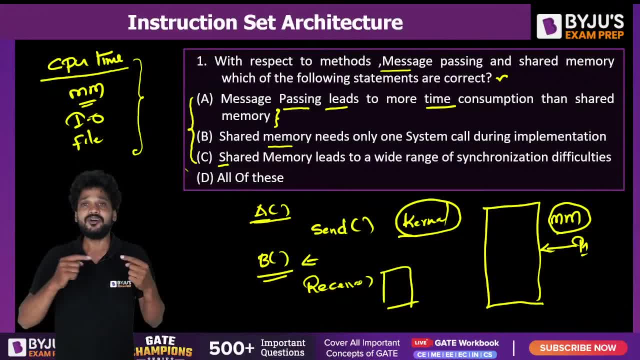 the process will be able to communicate with each other whenever do have only a simple- uh, you know what you call limited data to share. let us say i want to share 2 mb of data with another process. this is not possible by the message passing. 2 mb is a huge. 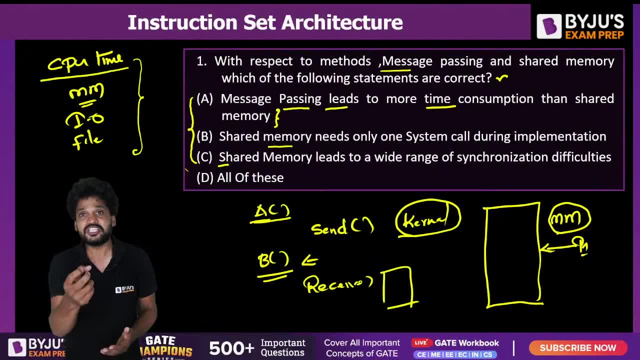 data. at that time, what we can do is we will use a shared memory where, in the shared memory which is being used by more than one process, the- the person the process wants to send the data to the other process- will write the data, will load the data within the shared memory, the other process which 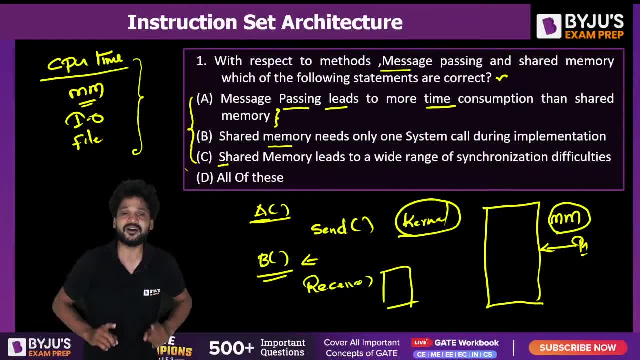 wants to read the data, will read it. so this is what all about shared memory technique. in the shared memory technique, we don't use extensive system quads. okay, we'll use only one system call, just only to create the shared memory in between several processes. operating system during the 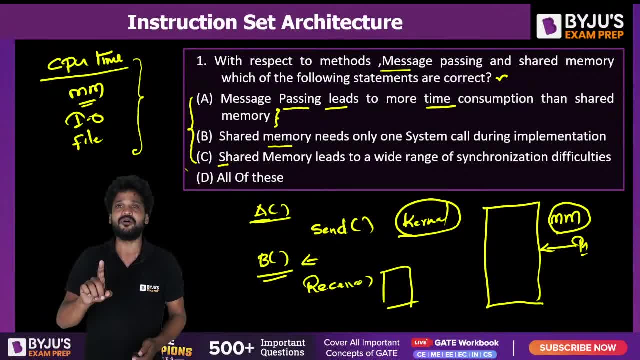 creation of the shared memory, we'll use one system call called create memory memory. okay, for that only we will use the system calls. so option b also is correct. the third one is: shared memory leads to wide range of synchronization difficulties. let me tell you, inter-process communication is all about the problem that we are going to face, such as race. 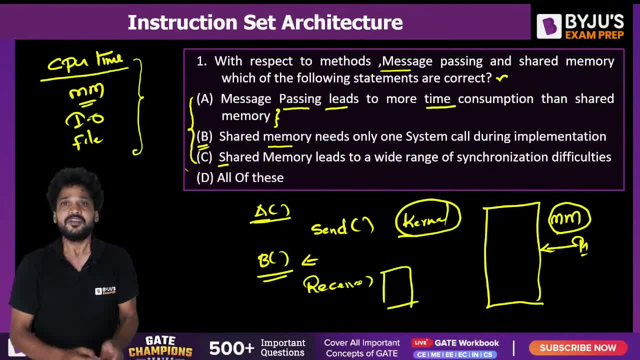 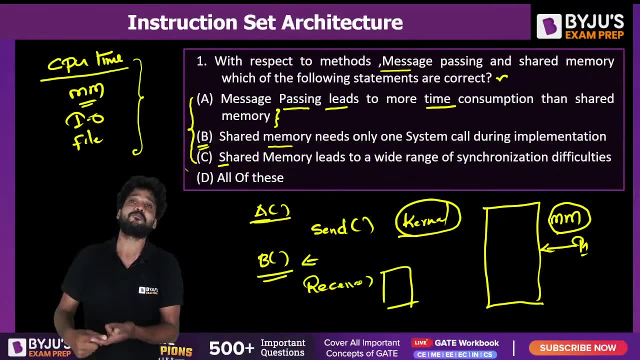 condition, such as critical section problem. you know what is. what is critical section problem? what is race condition? right? all the total inter-process communication is just all about providing the solution to the critical section problem. why the critical section problem we are discussing right now? critical section problem origin is our shared memory. if there is no shared memory, there are no. 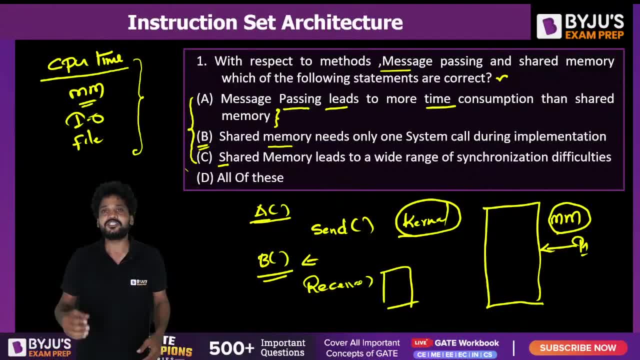 difficulties. there are no problems at all. operating system will hold its head whenever two processes want to communicate with each other, because a shared memory needs to be established. right after i establish the shared memory, then there may be a lot of chaos, there will be a lot of disturbances, there are there are a lot of. 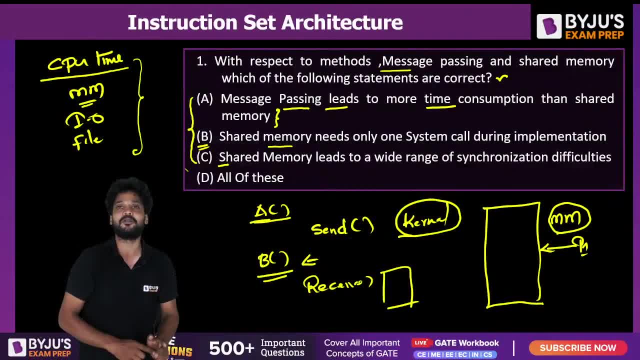 complexities such as race condition and a critical section problem. okay, so we need to find out the solutions for all those problems and see option c in that light. option c also is correct. shared memory leads to a lot of difficulties, right, so option d is correct in this regard. can i go to the? 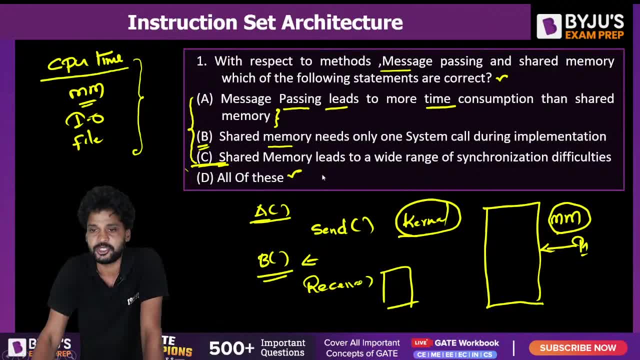 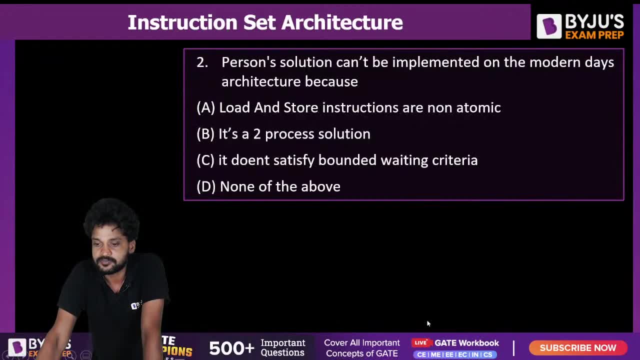 next question. it's a simple question. can i go to the next question? a bit of less and um and and can i go to the next question here? next question is on your screen: sri hita, um peter's solution can't be implemented on the modern disk architecture because understand that, see, write it down somewhere if there is a critical. 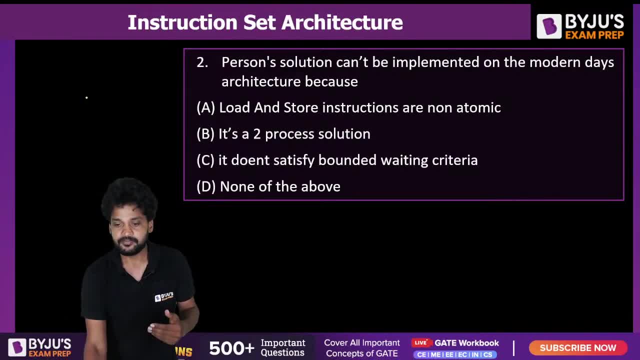 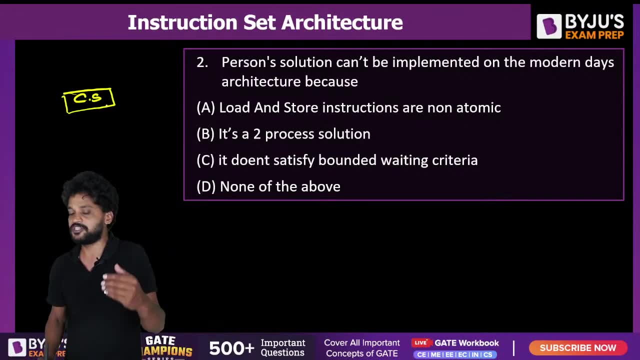 section problem. if there is a critical section problem, we need to protect the critical section. see, hita, understand. i know, uh, the operating system for you is not yet done, but understand clearly: critical section is the piece of code which can be executed by only one process. there is process one and there is process two. understand carefully these process 1 and 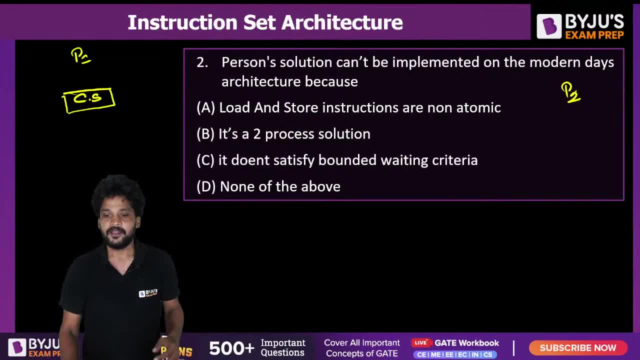 process 2 are actually cooperative processors. so in process one there is something called a critical section. in process 2 also, there is something called a critical section. what is this critical section when process p1 and process p2 executing in their respective critical sections? they are. 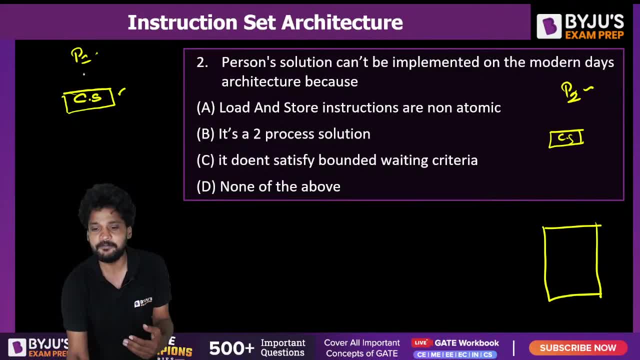 to access a memory region which is shared in between process p1 and p2. right ability will correct me if i'm wrong. yes, i know this is what our critical section problem. right, let us say myself: i am one process. mr abed will is. he is one more process. we both are cooperative process. 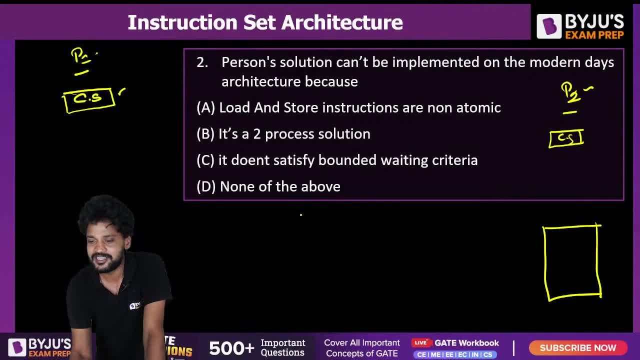 i will example this one. what is this? let us say there is a compiler, i am compiler, mr abed will is loader. got my point here: compiler and loader will have to get executed one after another. that to compiler and loader need to use a shared memory region. okay, let us say when, when, when. compiler. 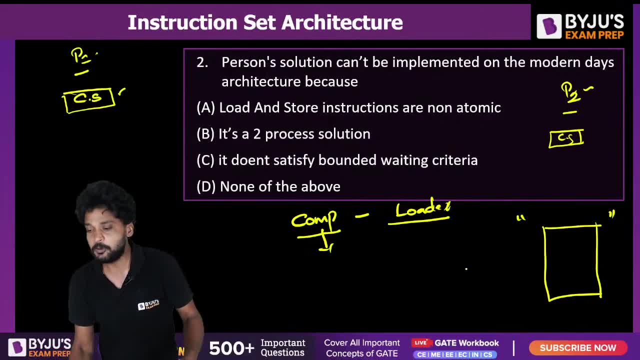 gets executed. this compiler is going to put some data in the shared region. the output of the compiler will be used by the loader sr. no, so when loader gets executed it is going to use the code that is being produced by. that's being produced by the compiler. so first compiler should execute. 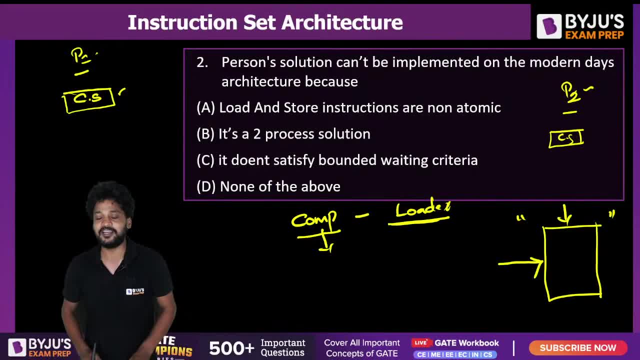 followed by the loader. right. so understand carefully. this compiler will write load. loader will read: okay, so process p1, such as compiler, process p2, such as loader. when they are executing, there is a section of code which acts as a critical section. understand carefully. only guy can access this critical. sorry, can access the shared memory at once, am i clear? can can access? 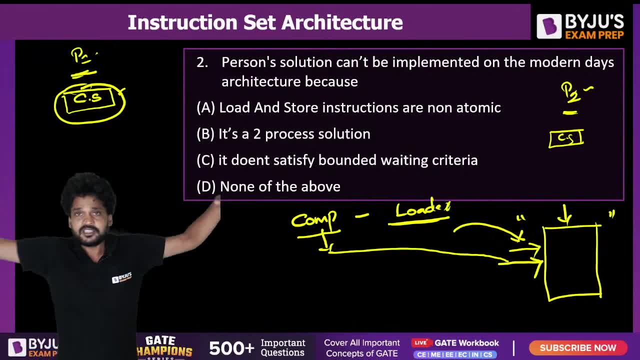 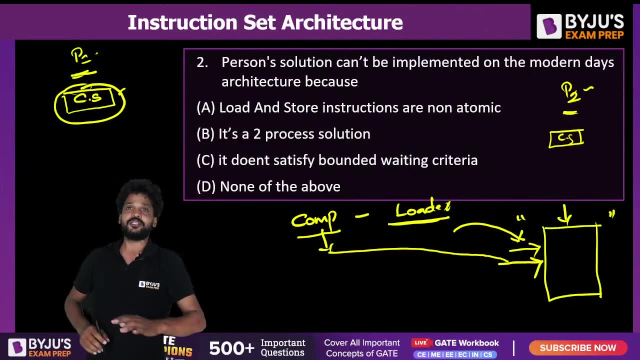 the shared memory at once. if both of you guys enter into our respective critical section, the shared region will be accessed at the same time, simultaneously, which leads to a lot of complications. did i make it myself clear? see, hita, whenever there is a shared memory region, which is 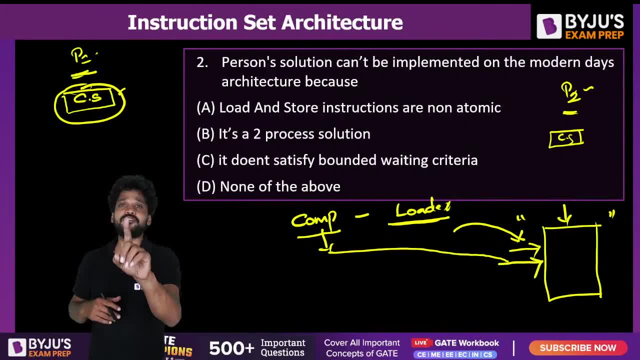 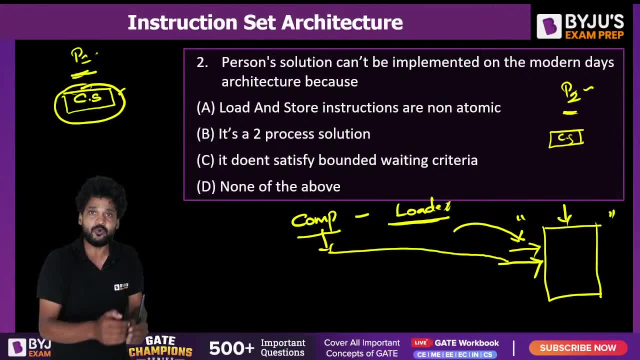 being used by more than one process. only one process should be able to use that shared region at once. if any process wants to share region again, he needs to wait for the other process to finish. okay, so for that, for that, uh re. for that reason, these critical sections must be protected by some. 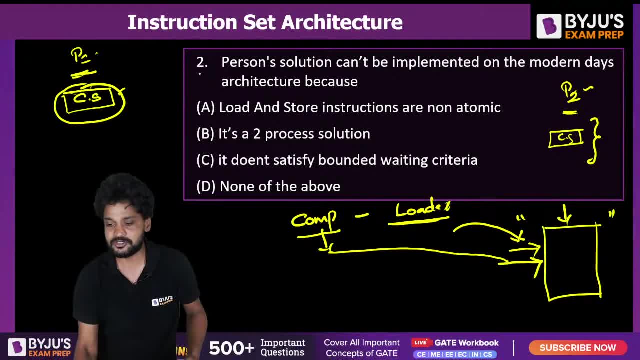 are the other solutions? there is one solution called peterson solution as, as these guys know, is used to protect the critical section. so p1, before enters into the critical section, it will use a peterson solution. this peterson solution is actually the best method, if it is implementable, to protect the critical section. 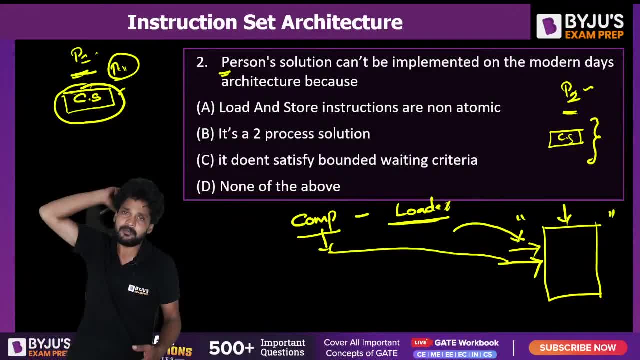 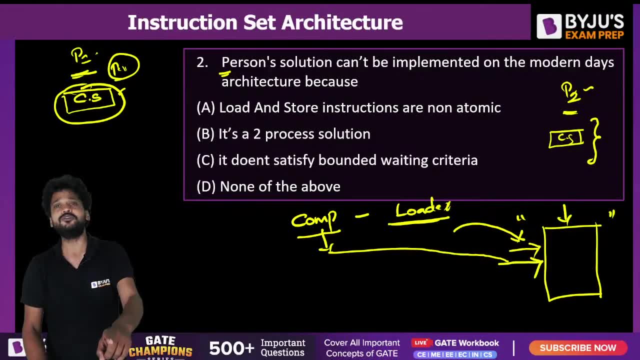 but actually the problem is peterson solution was developed way back in 1970s or 1960s which cannot be utilized in the modern-day architecture. if you want to use the peterson solution to protect your critical section within your application, it is not possible at all because 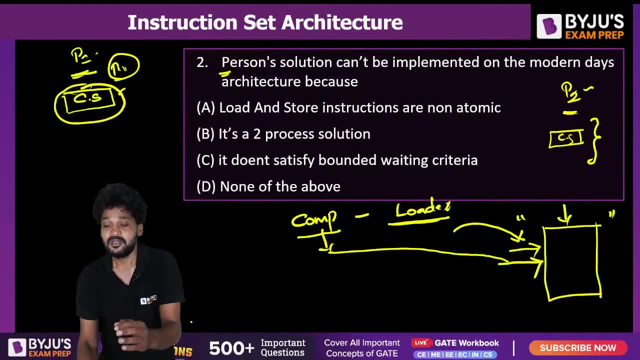 peterson solution uses to act. rather, you know patent solution uses normal load and store instructions. yes, i know peterson solution. actually, when access the main memory, it just uses regular instructions such as load and store. load and store are non-atomic. load and store can be printed right. 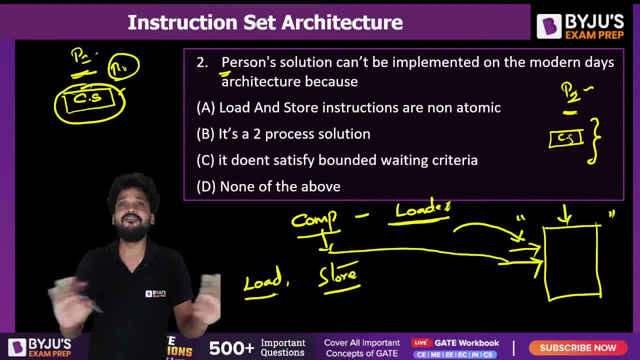 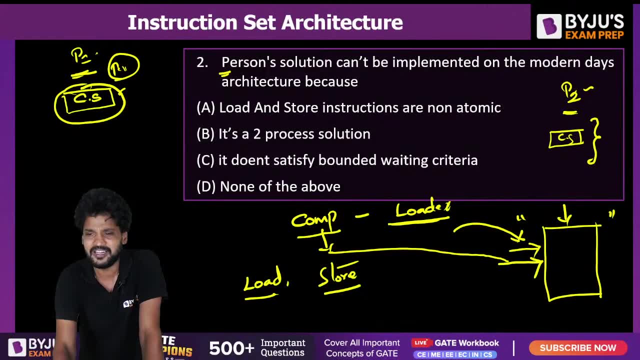 so this is the very reason why peterson solution will not work on the modern-day architecture. so i'm out of time. p4- let's talk a little bit about p2. go back a bit more. p3 from the wait. p4 and consumer problem: right now, in 2022, even for two processes, you won't be able. 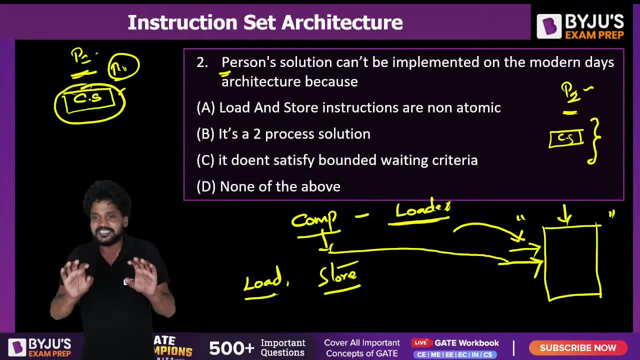 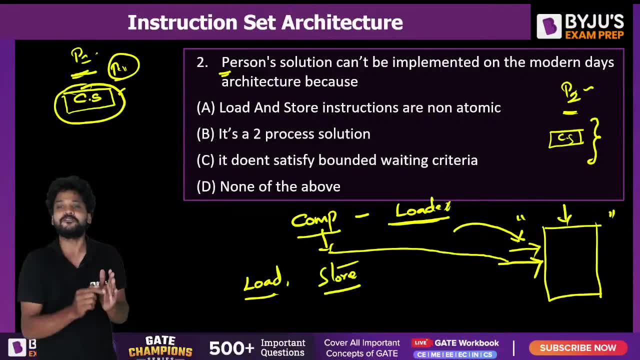 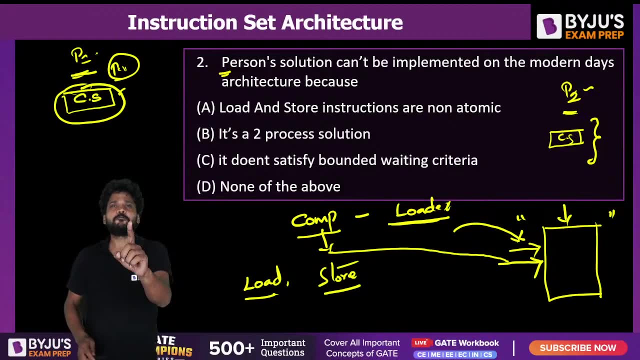 to Peterson solution. even to protect the critical section of the producer and consumer, you won't be able to use Peterson solution. it is simply because Peterson solution uses normal load and store instructions. I hope I made my point clear. even for a two process critical section, Peterson solution. 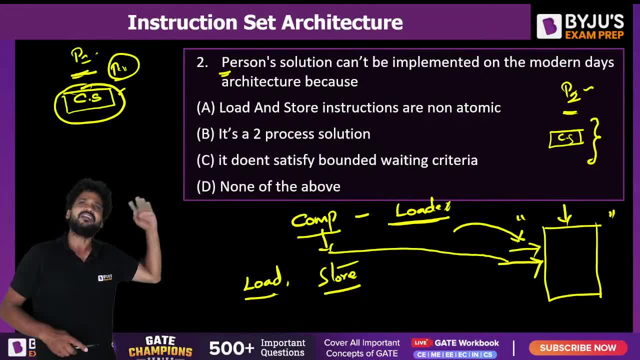 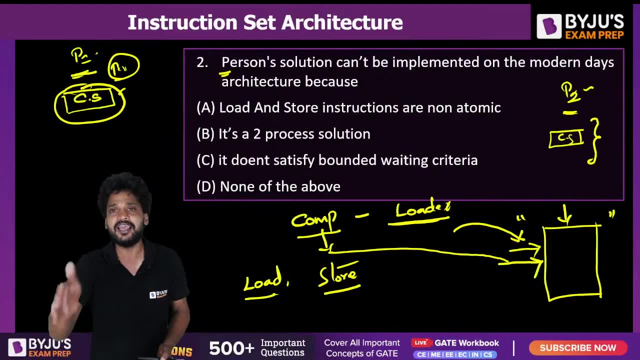 cannot be used in 2022 because it was the older arm. you know the method to predict critical section: older solution. it cannot be implementable in 2022 in the modern-day architecture at all. load and store instructions are non atomic, simple Peterson's. the solution uses general, normal load and store. 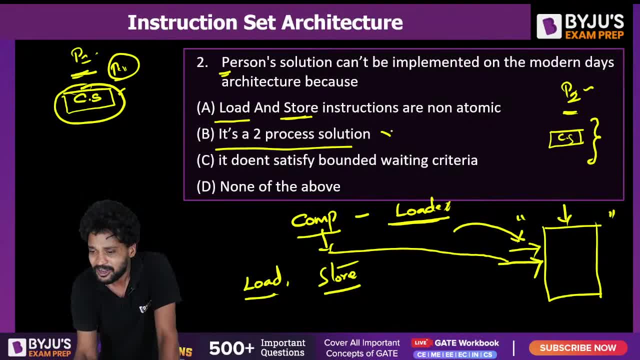 instructions. it's a two process solution. it is a wrong option. of course. Peterson solution works only for two process. even in 1960s, Peterson's solution cannot be used for 10 processes. Pay-to-send solution can only be used for 2 processes. But now, 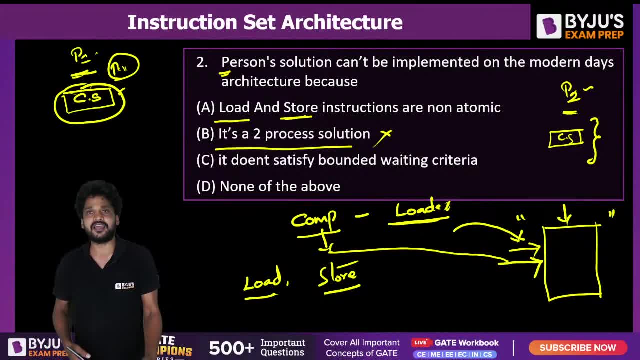 let us in 2022. let us example that there is a producer-consumer problem. Even for a producer-consumer problem, although it's the 2 process problem, pay-to-send solution cannot be used because of the simple reason that option A load and store instructions. 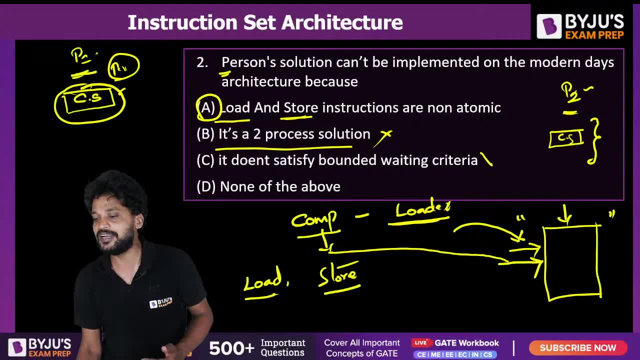 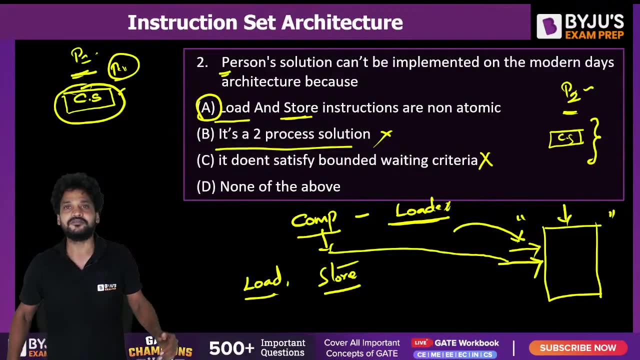 and third one is it does not satisfy. bounded weighting criteria should also be ruled out When you talk about the pay-to-send solution. although we accept that it cannot work, pay-to-send solution will give you the best algorithmic description in such a way that it will satisfy all. 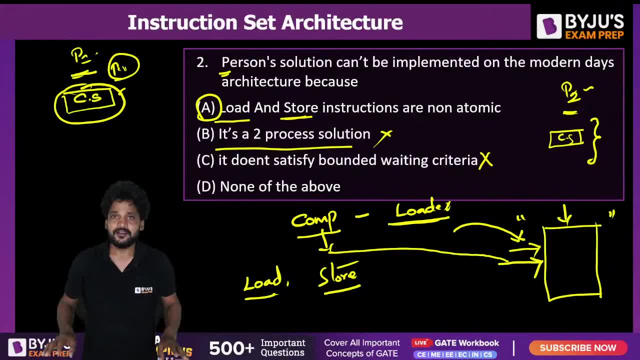 the criteria Srihita understand. whenever we want to define our solution, let us say critical section must be protected. when the critical section has to be protected, you can use any solution that are already available or you can design your own solution, Being a. 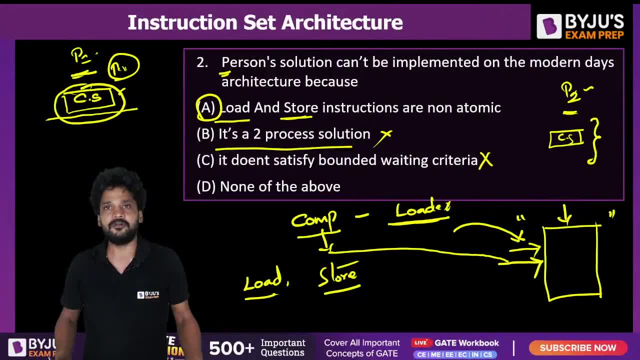 programmer. it is possible. You are a good application program developer. It is still possible that you can develop your own solution. But if you want to develop your own solution, there must be 3 criterions must be followed. What are those abitabulous? tell me. One is: 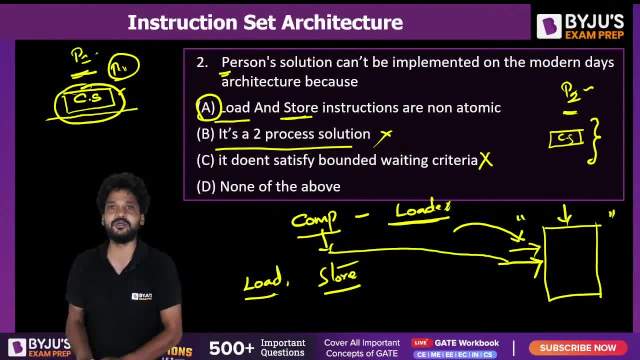 progress. one more is bounded weighting. one more is mutual exclusion. For this I request you to watch my classes on operating systems in inter-process communication. I explain a lot, but if there is a solution, that solution should satisfy 3 criterions. First one: 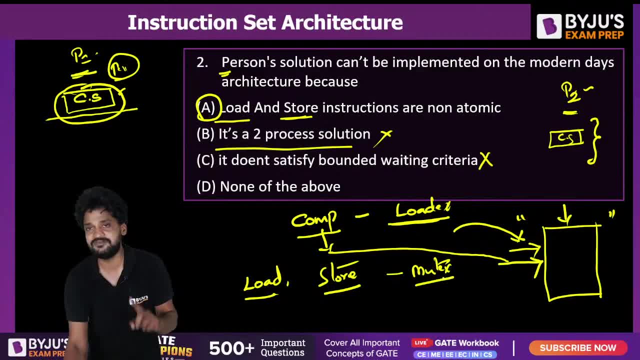 is mutual exclusion. Mutual exclusion will allow only one process to be in the critical section. Second one is bounded weighting. Bounded weighting will avoid starvation. A process should not enter into the critical section again and again and again as long as one more process is waiting. 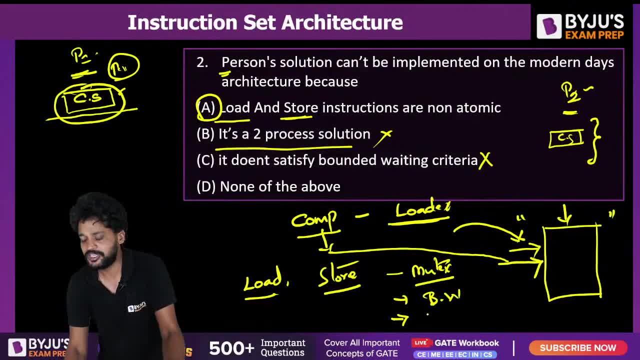 And the third one is: what do you call the progress? These 3 must be satisfied. Peterson's solution straightaway will satisfy all these 3 criterions. This is a very good solution, but only the thing is it is not practical in 2022. 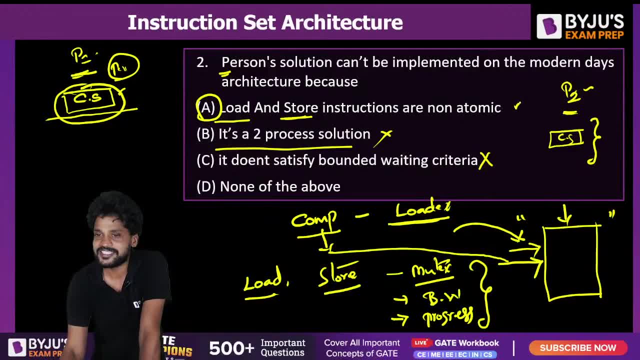 So what is our pick right now? Option A is correct. Am I right? abitabulous, Am I right? Option A is correct. right, It is simple, It is sensible. Option A looks very sensible. at this point Did I make myself clear. 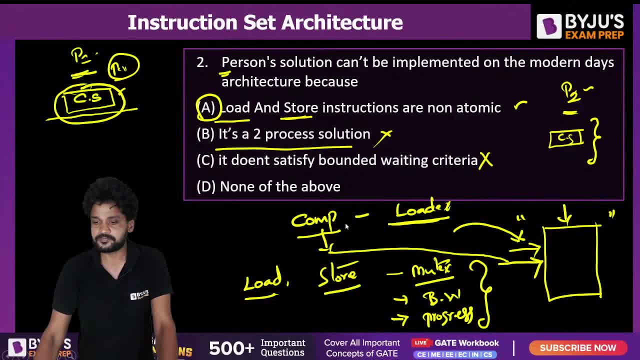 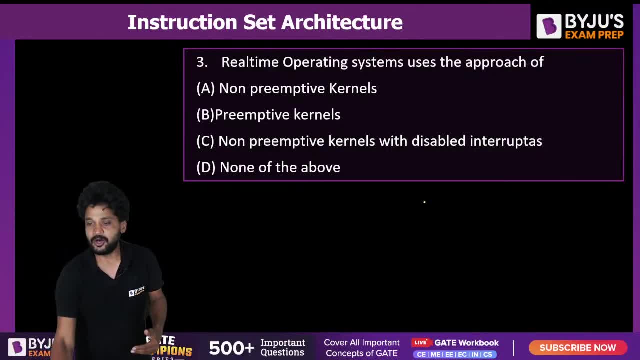 Yes, Shall we go to the next question? Yeah, A real-time operating system uses the approach of non-preemptive kernels. preemptive kernels, non-preemptive kernels with the disabled intrex. none of the above. What is the correct option here? 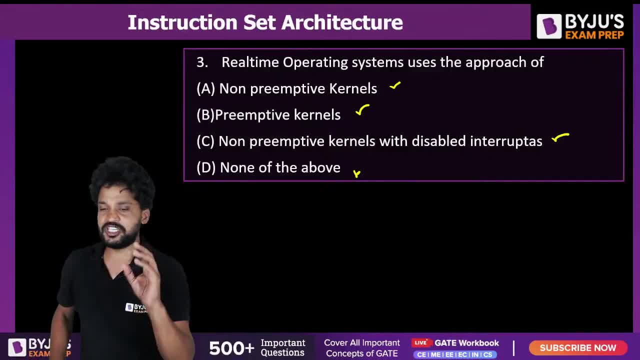 Nilmadhav abitabulous. of course Shihita is the first class. I can't ask her because she is just watching it. You just take your time to get into this topic. Meanwhile, I don't disturb you with my questions. 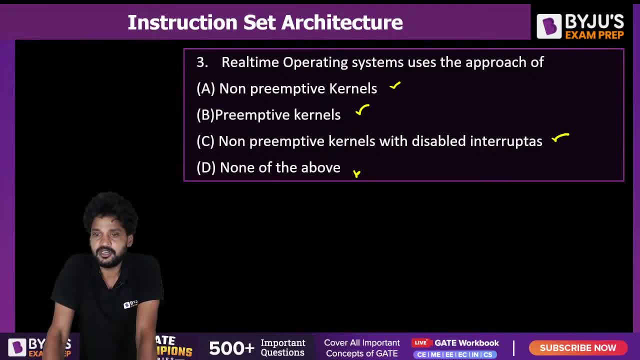 Okay, Yep, Pranjal, tell me what is your pick. Real-time operating system uses the approach of what? Preemptive kernels or non-preemptive kernels? Okay, For this I will tell you a story. in order to answer this, I will tell you a story. 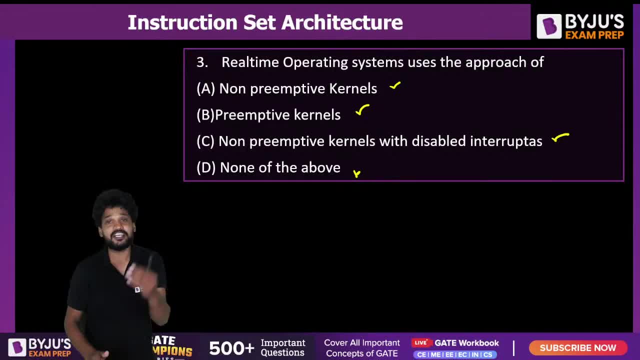 Okay, This story is the same example that I will explain to demonstrate what is the real-time operating system. Okay, And understand and stay with me. I will make it clear. Mr Nilmadhav Sahu is correct. Preemptive kernels. 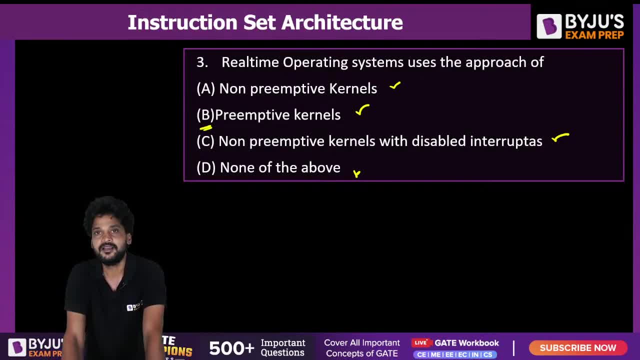 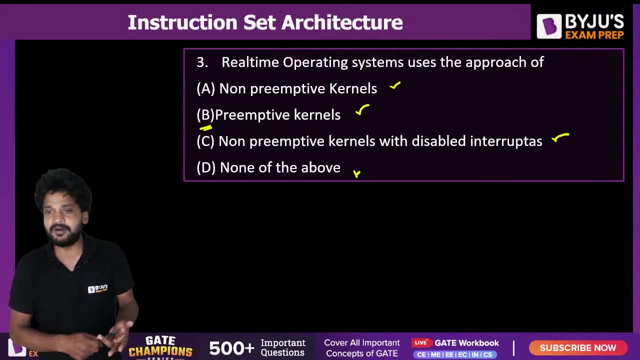 is perfectly right. Understand carefully. There are two things. If you want to develop an operating system, no matter who you really are- you could be Nilmadhav, you could be Pranjal, you could be Shihita or abitabulous. When you want to, 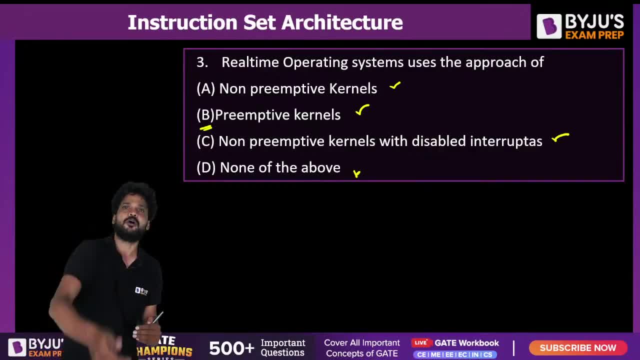 develop your own operating system, your custom operating system. you have two ways to develop your operating system. One is preemptive kernels, One more is non-preemptive kernels. You already know kernel mode and user mode, right Preemptive kernel meaning. 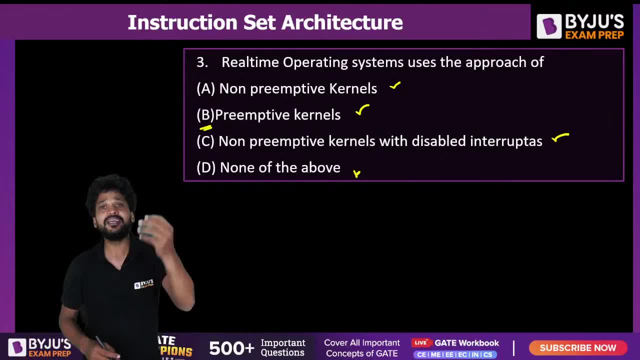 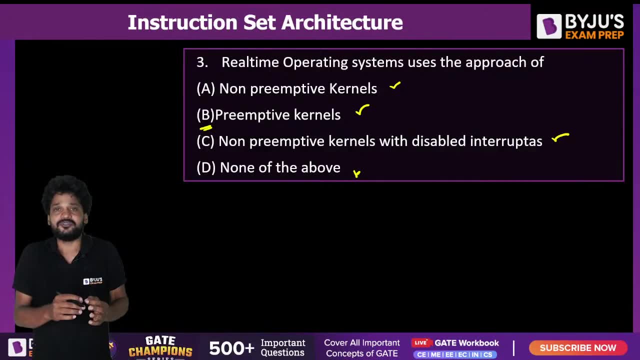 when a process is executing in the kernel mode, it can be preempted. Non-preemptive kernel meaning when a process is executing in the kernel mode, it cannot be preempted at all. In these two ways, you can design your custom operating system. 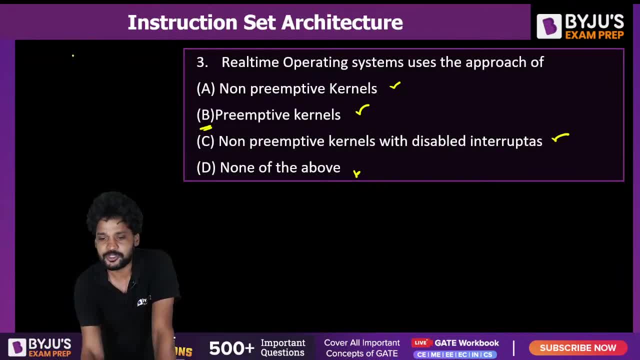 Now understand what is a real-time operating system. Okay, In the real-time operating system, the process should be executed within a stipulated time. For that I will give you an example of ABS, The same example that I used in my previous class. 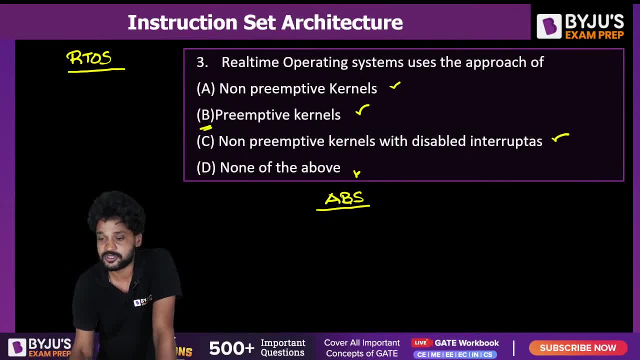 while I was taking, while I was discussing about real-time operating system, What is ABS, Anti-lock breaking system? I think you heard about a car. right In the cars we use anti-lock breaking system. Okay, Anti-lock breaking system. 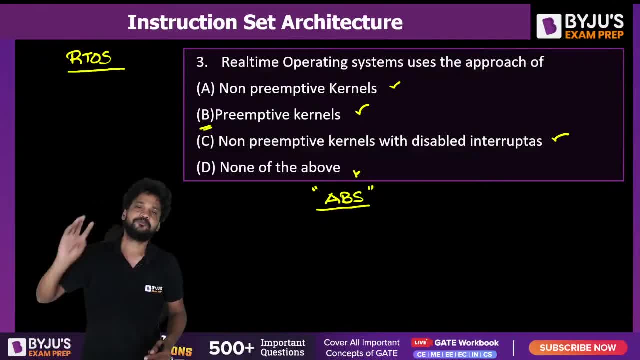 if we do not get into the details. is a process? Is a process? Anti-lock breaking system, when executed, will avoid the accidents- Okay, But anti-lock breaking system will only work when the sudden breaks are applied. Am I clear? 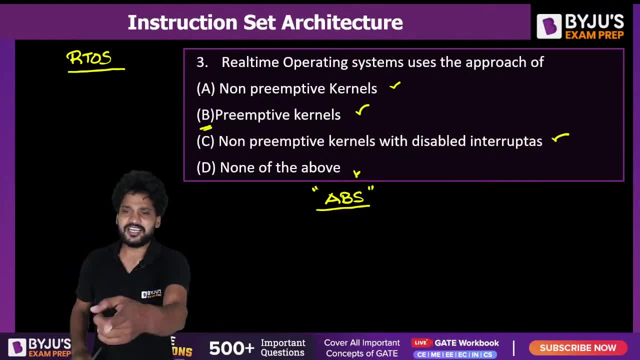 Yes or no? Anti-lock breaking. Have you heard about anti-lock breaking system? Prangel, Neil, Madhav, ABWs Sri Hitha. Have you ever heard about anti-lock breaking system or not, Yes or no? You there. 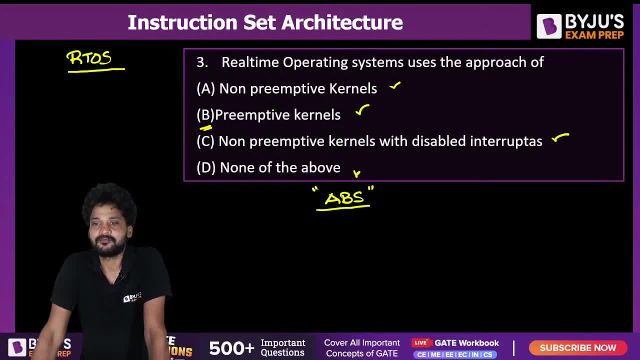 Or slept already. Yeah, When. anti-lock breaking system? Yeah, understand, Sri Hitha. What is anti-lock breaking system? See, when the sudden break is applied, the problem is: tyre will start sliding, The wheel will get jammed and it will slide. 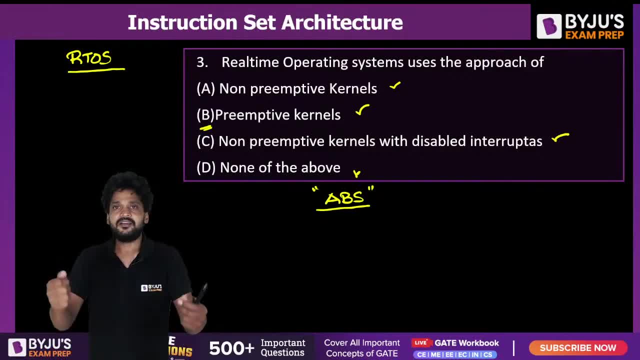 When wheel starts sliding, I mean your steering will not be under your control. Your steering will be completely under your control as long as wheels are rotating, But when you apply sudden break, wheels will not be under your control. Wheels will start sliding. So, according to the Newton's, 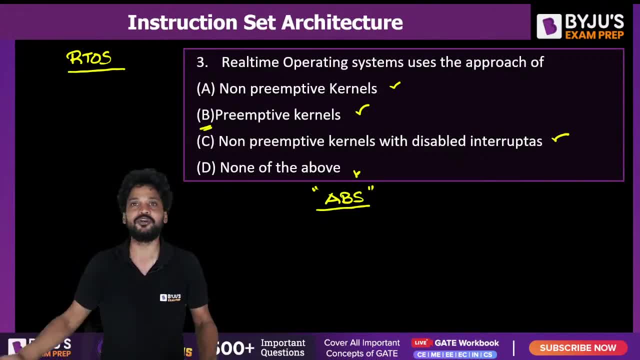 law of motion, inertia of rest, inertia of motion. your car will fly away somewhere to mid accident. Sudden break is the problem. Anti-lock breaking system when executing will avoid the wheels from being jammed, even when you apply the sudden break. 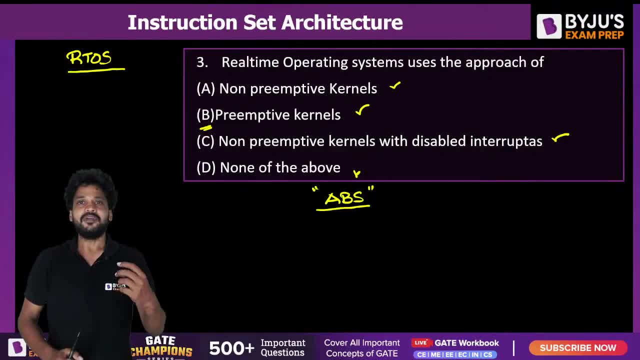 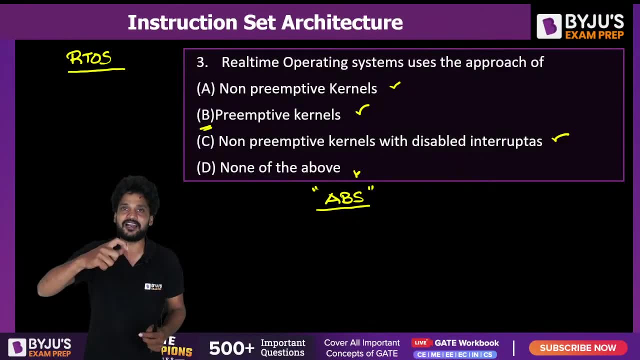 The car which is equipped with anti-lock breaking system will allow the wheel to still rotate and get jammed Again. rotate, get jammed During the anti-lock breaking system. wheel will run and break, Will run again, will get locked, Will run. 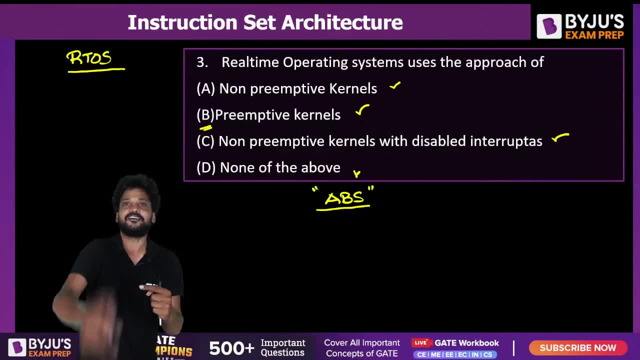 again will get locked, So periodically, wheel will still run, So the wheel will sorry. the steering will still be under your control, So you will be able to drive your car to the safer place. Why did I take this example? 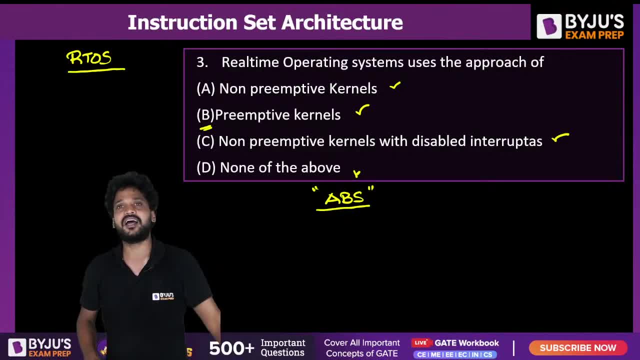 Anti-lock breaking system can be used in any car as a process. If you want to equip your car with the anti-lock breaking system, it can only be done by an embedded processor. The car must be supported by a processor. Okay, this processor. 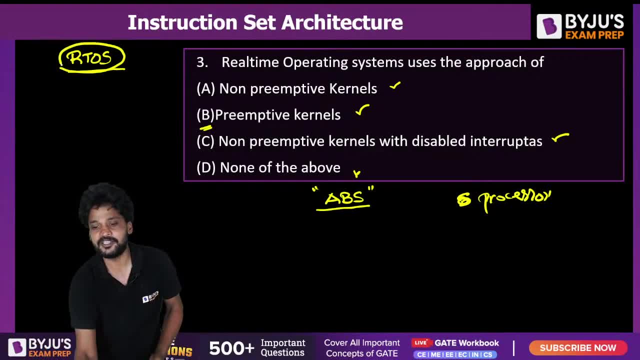 should be supported with the real-time operating system. What is the real-time operating system? In the real-time operating system, there are some process called critical processes. What is the critical process? ABS is the critical process When this process arrives into the main memory. 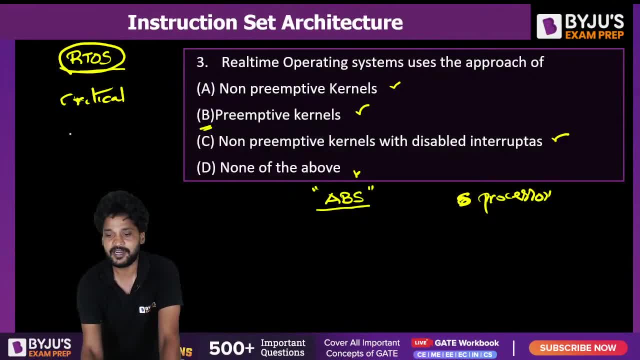 within no time it should be executed. Okay, for that, what we need to do is we should implement. we should only follow the approach of primitive kernels. What is the primitive kernel? Primitive kernel will allow a process to be primted. 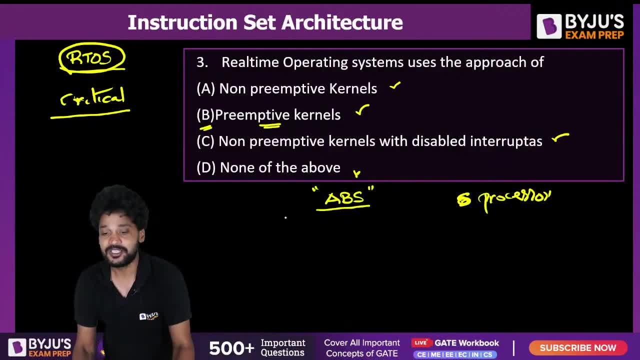 even though, when it is executed in the kernel mode Such, let us say you applied a sudden break- ABS immediately will get triggered. ABS will immediately come into the main memory. The moment ABS comes into the main memory, within no time our CPU 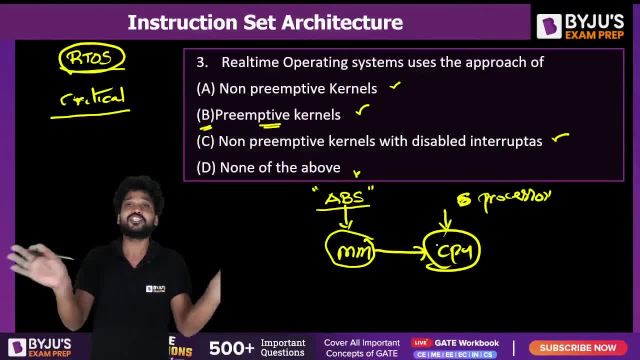 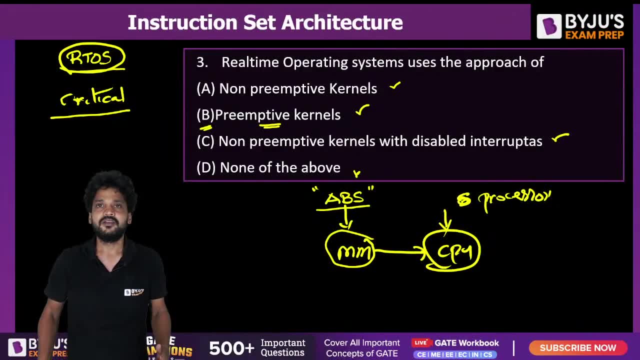 should execute. Unless the CPU executes, this, ABS doesn't work. But is the CPU free? If you do have a CPU, obviously that CPU will do some or the other job. Okay, let us say that job is in the kernel mode. 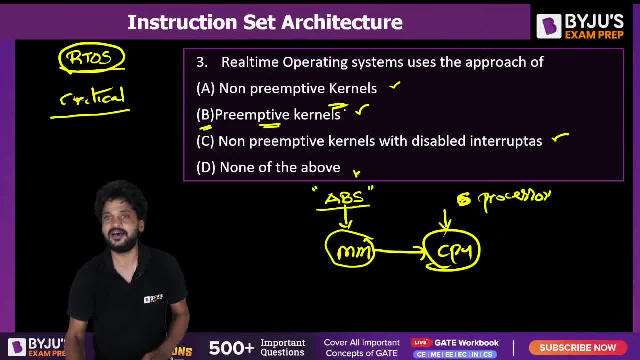 It cannot be primted. in the non-primted kernels, Your car will not be able to execute ABS within time. Yes or no? You will not have much time. The moment you apply the break, you have the milliseconds to have the ABS triggered Within that. 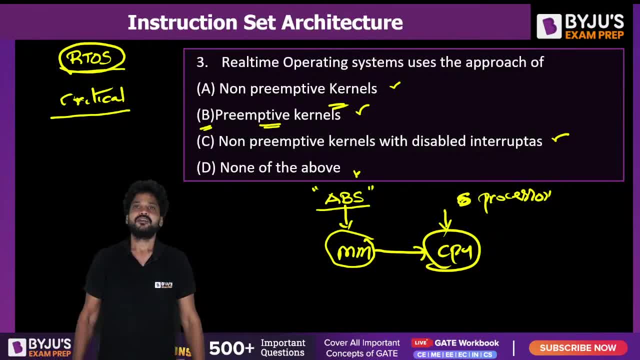 milliseconds. if ABS doesn't get executed, simple, You will find yourself sitting next to your grandparents in heaven or hell Pulling your legs. Fine, I hope I made my point clear. So we use only primted kernels In the primted kernels. 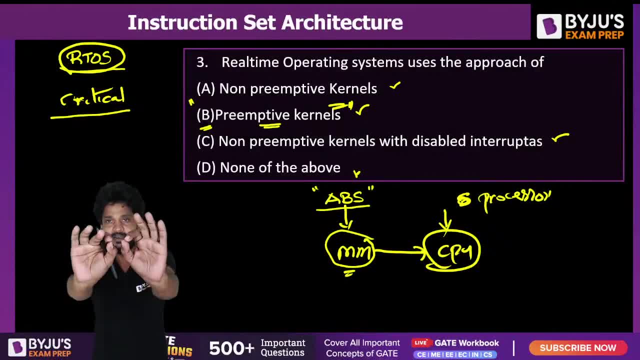 even though a process is executing in the kernel mode, it will be primted back to the main memory and the real-time process, such as ABS, will immediately be sent to the CPU for execution. Okay, So real-time operating system will always use primted. 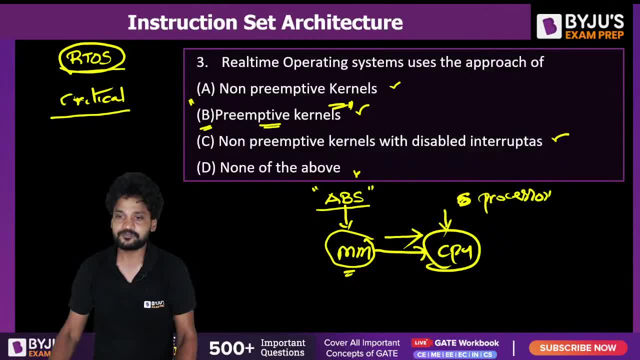 kernels. Did I make myself clear? Can I go to the next question? Are we done? Non-primted kernels is straight away to be ruled out. Non-primted kernel meaning I won't be able to primt one process at all. 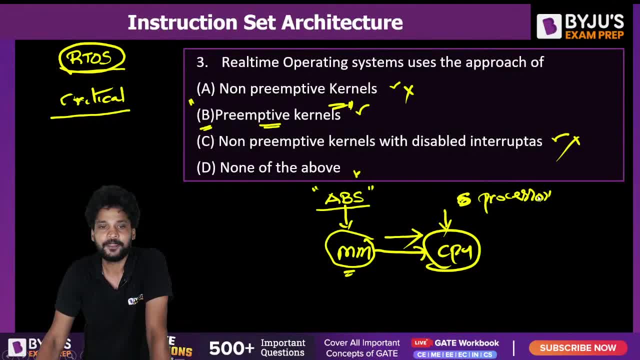 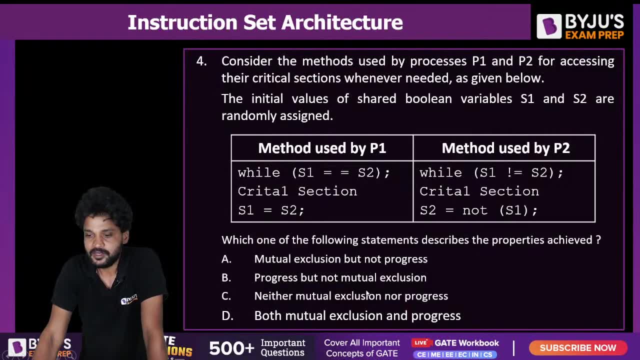 Can I go to the next question? Yeah, A bit of a list. Are we done with this, Srihita? are we done with this? Okay then Next question is on your screen For change. I will give you one minute. 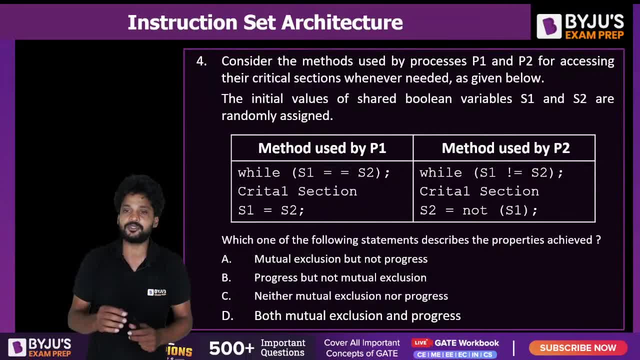 to solve this question. I will give one minute to solve this question, Srihita. what you do is just go through this. You just go through this, You will get to the topic directly. You don't need any introduction to solve this question, Okay. 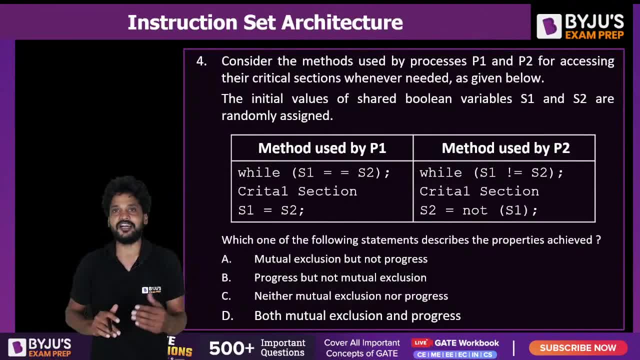 Because we just what we need to in order to understand, in order to get to the answer, we just need to understand the basic programming Already. I know that you people are well equipped with this basic programming techniques. Just I don't. 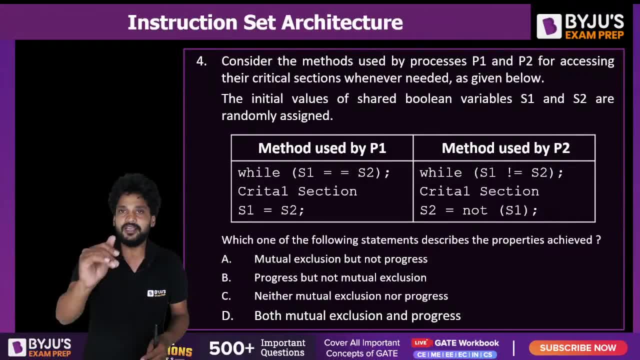 want you to answer. Watch that, Meanwhile, the remaining people. I just want you people to give me the answers right away. Neel Madhav, what is the answer for this? The question: what is on your screen has got what answer? 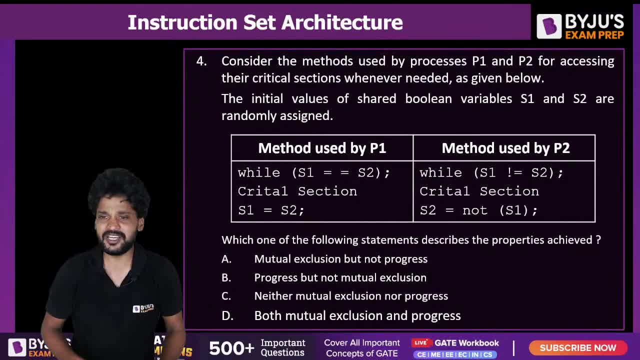 And Prangal Abhidevil is with other guys. Neel Madhav, Prangal, only few people are here. Why Lot of people is showing here, But why only few people? Let me see, Fine, Anyhow. what is answer? 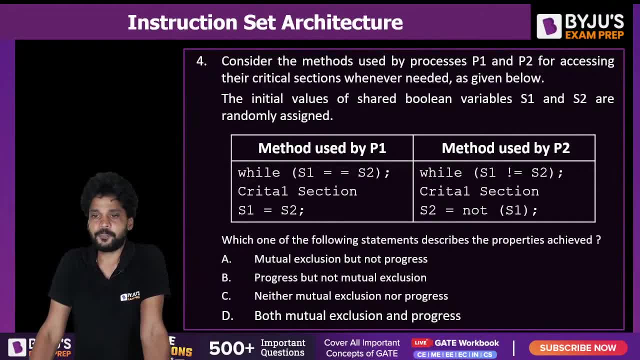 for this. What is answer for this Abhidevil is, May I know? May I ask you? You have one minute. Consider the methods used by process P1 and P2 by accessing the critical section whenever needed, as given below The initial. 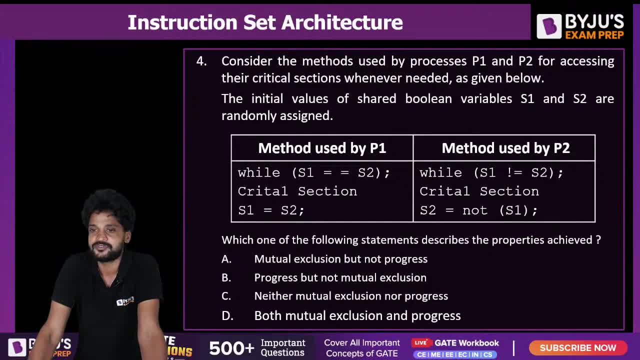 values of the shared billion variables S1 and S2 are randomly assigned Both mutual exclusion and progress. Is there? D Abhidevil is: Is Neel Madhav correct? Is Neel Madhav correct or not? Are you there? 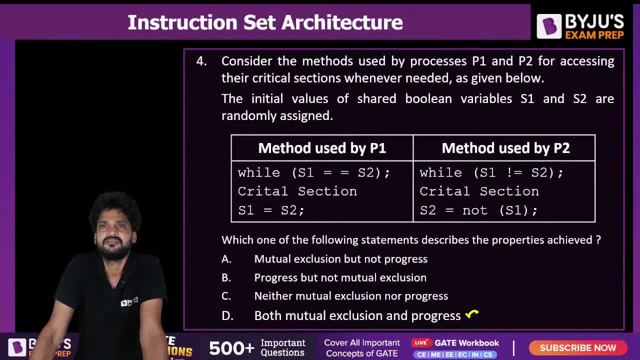 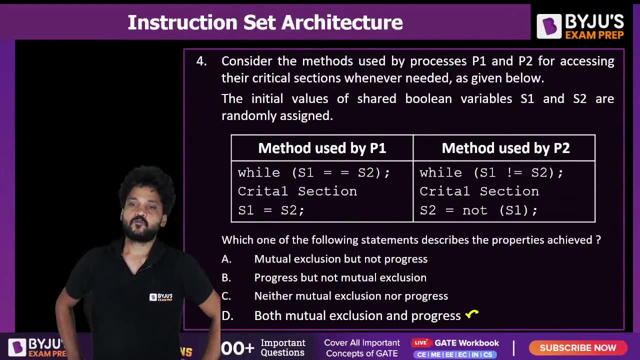 Are you there? Are you there or you slept? Abhidevil is Prangal. what is your pick, Sridhar, can you give me random answer? Some random answer? Fine, Let us understand. Let us understand this. 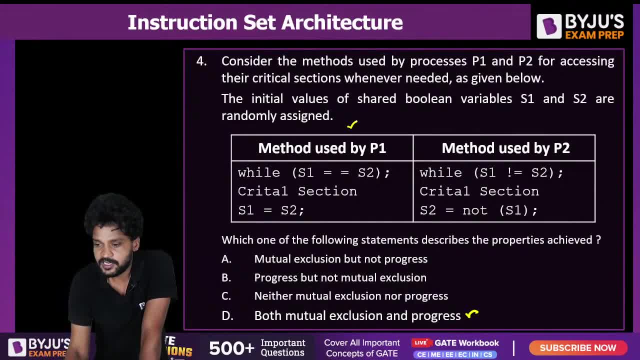 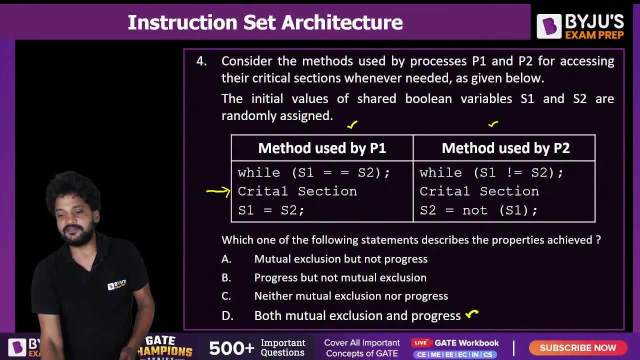 See, There is process P1 and there is process P2.. It is understood that only one process should be allowed to enter into the critical section. Now you just have a look at this. There is a while loop which prevents a process from entering. 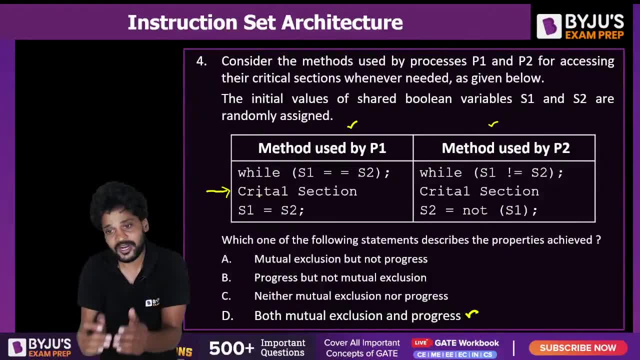 into the critical section or allows a process to enter into the critical section. For that, let us take the values of S1 and S2.. As these are randomly assigned, we will imagine the values of S1 and S2.. Let us say S1. 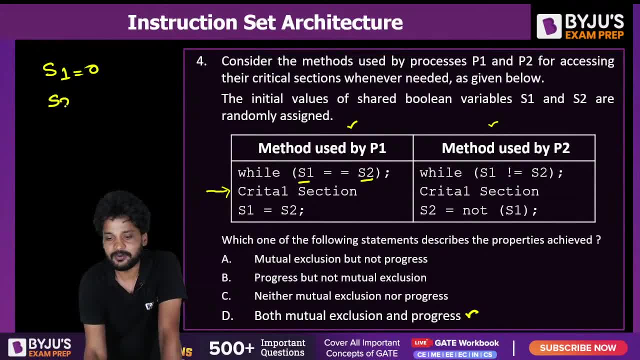 is equal to 0. S2 also is equal to 0. Both are equal to 0. Now, when both are equal to 0, obviously this process will get locked here. This process will not be able to enter into the critical section. 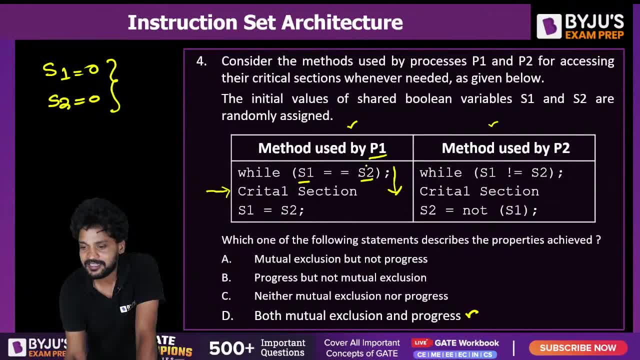 That means that process P1 will be caught in the while loop. Am I correct, Srihita? Will I be able to enter into my critical section next to the while loop? No, Because, as the condition gets satisfied, the first process will be. 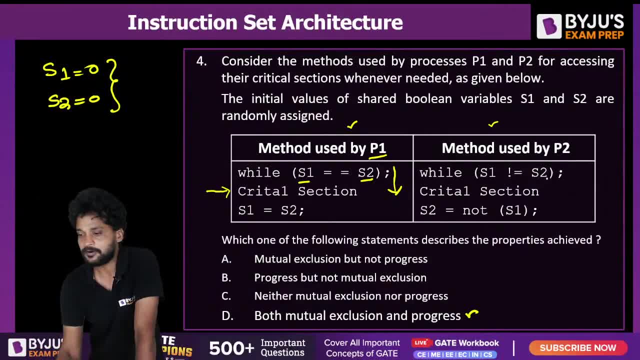 caught in the while loop At the same time, second process as second process, as S1 is equal to S2- will be able to come out of the while loop and starts executing in its critical section. Okay, Is that clear, Yes or no? So? 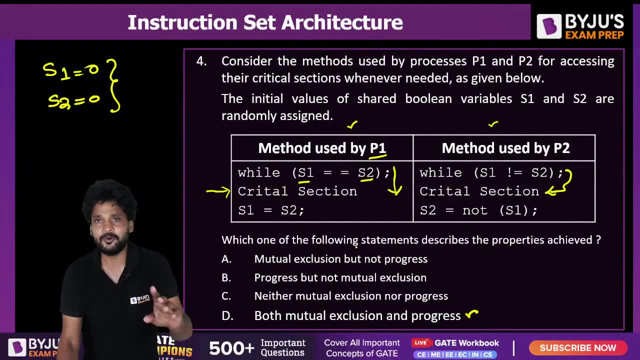 mutual exclusion is guaranteed. Only one process will be able to be allowed into the critical section. Okay, If it is: S1 is 1, S2 is equal to 0. In this case, P1 will be allowed into the critical section. P2 will be locked in the 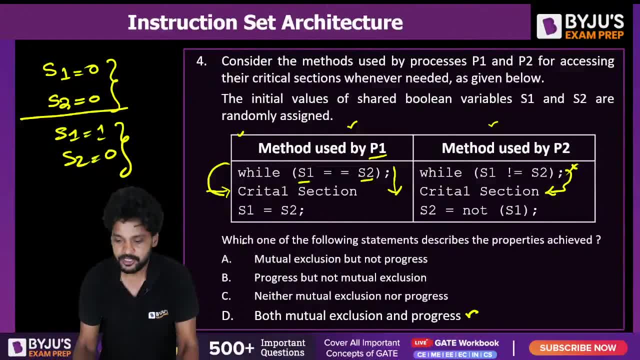 while loop. I hope till then we are clear. So the example, what we are taking here is: S1 is equal to 0, S2 is equal to 0. Both are equal. Okay, Now understand K2.. According. 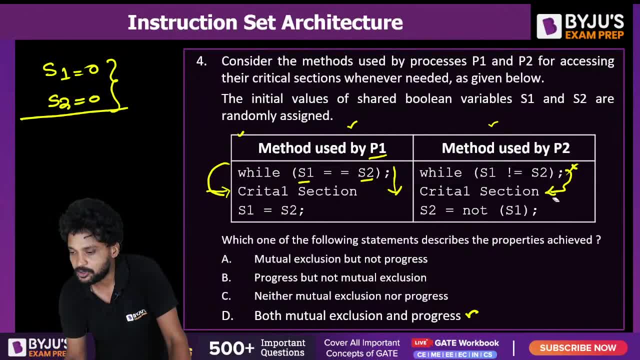 to this condition, P2 will be able to enter into the critical section. But the moment the P2 comes out, what will be set by the P2?? S1 is not equal to S2. So S1 is equal to 1,. 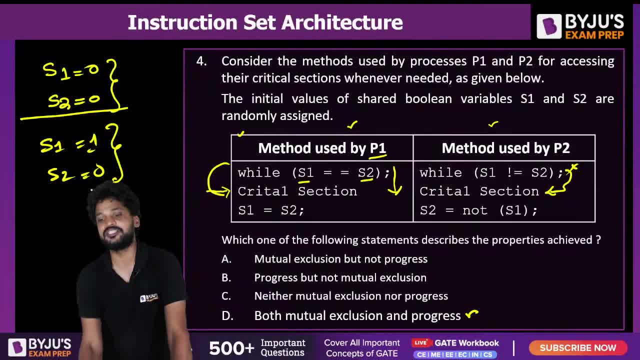 S2 is equal to 0. It will make: S1 is equal to 1, S2 is equal to 0. Or any other thing which makes S1 is not equal to S2. Because that is the code that has been written here in the P2.. 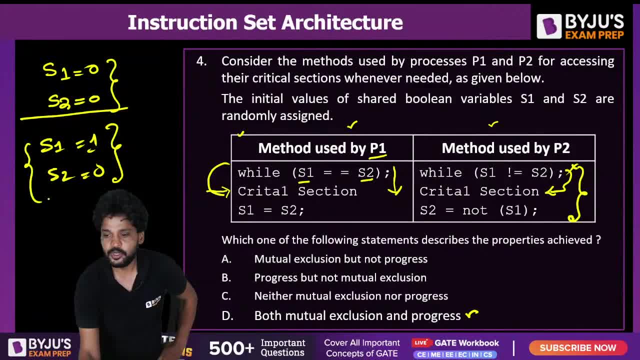 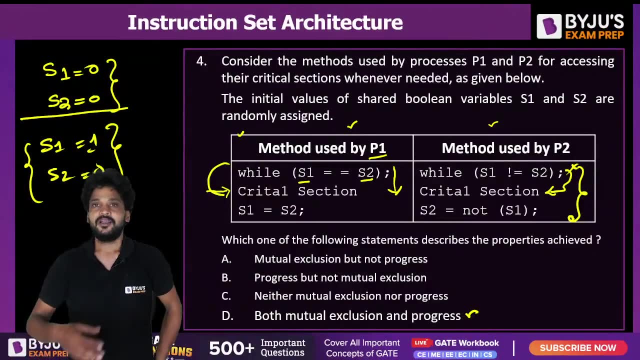 SR: no, If S1 is not equal to S2, then P1 is allowed into the critical section. Understand carefully Here the thing is: stay focused. What if P1 doesn't want to enter into the critical section? I am P1.. There is one more process. 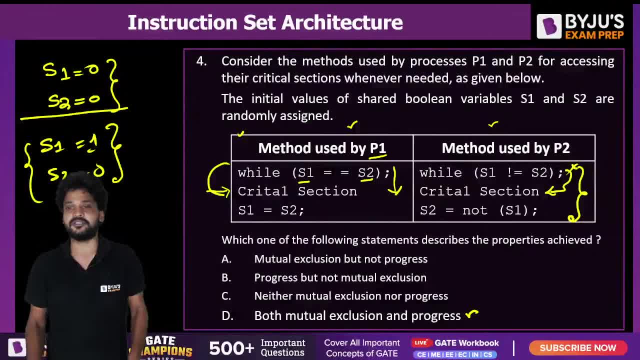 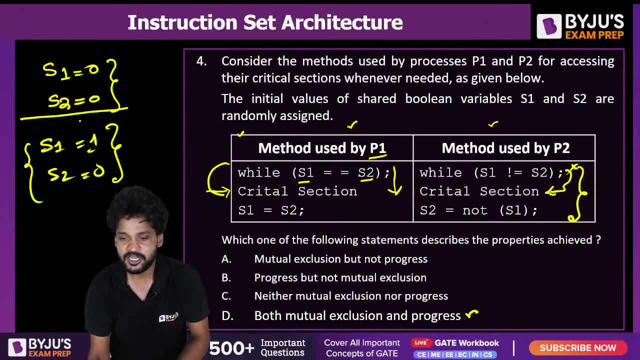 P2.. I don't want to enter into the critical section. Let us say Neel Madhav want to enter into the critical section. He went in because the moment, straight away when he checked this, S1 is equal to 0, S2 is equal. 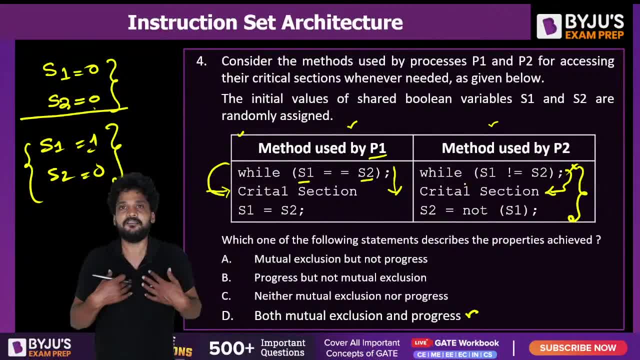 to 0. Immediately he will enter into the critical section At the same time. P1,, I don't want to enter into the critical section. I am executing in my Samadhar code. I do not want to enter into the critical section, But. 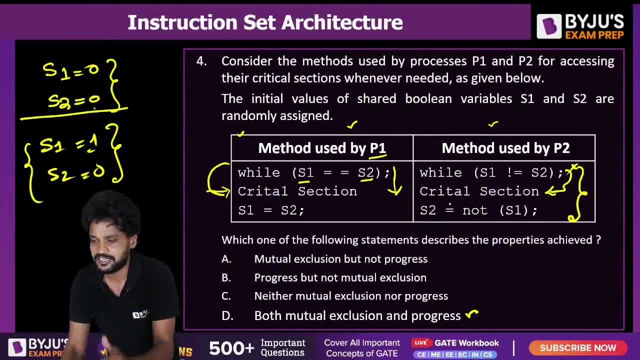 the Sahoo will be Neel Madhav Sahoo. he entered into the critical section. By the time he comes out, he has to execute one more instruction which makes S1 and S2 are not equal. Then he leaves Here. 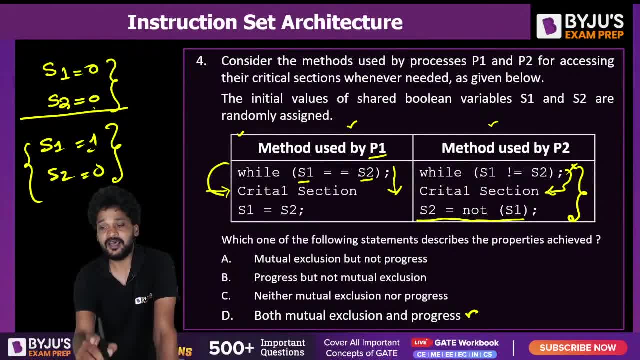 as long as S1 is not equal to S2, it will allow only P1, but not P2, to enter into its critical section. At this time, as S1 is not equal to S2, P1 cannot enter. P1 can enter P2. 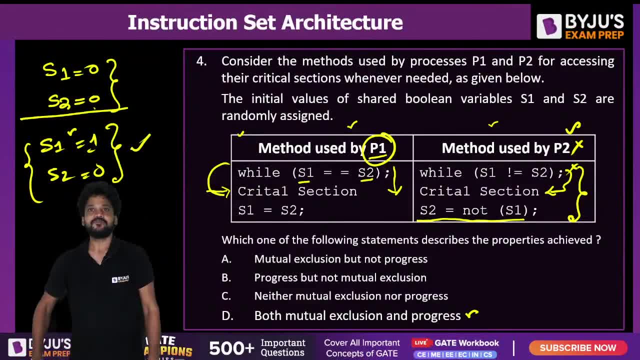 can never enter into the critical section at this point. Now understand what if P1 doesn't want to enter into the critical section? I don't want to enter. I am executing in some other code, But at the same time Sahoo wants. 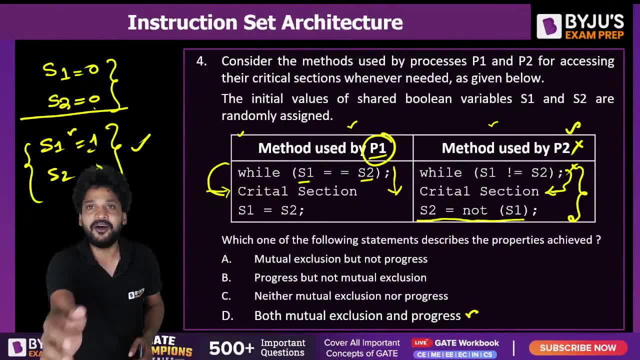 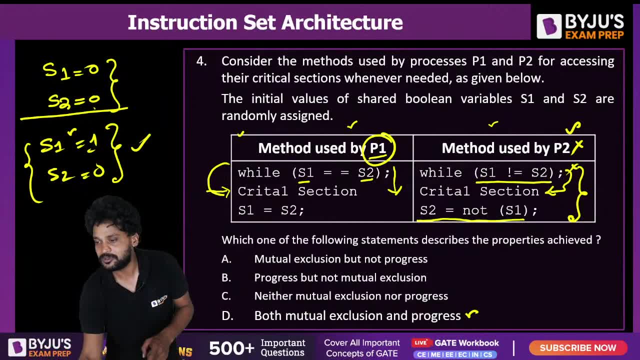 to re-enter into the critical section. No, he cannot re-enter into the critical section because S1 is not equal to S2.. As long as S1 is not equal to S2, he will be caught up in the while loop. Did I make? 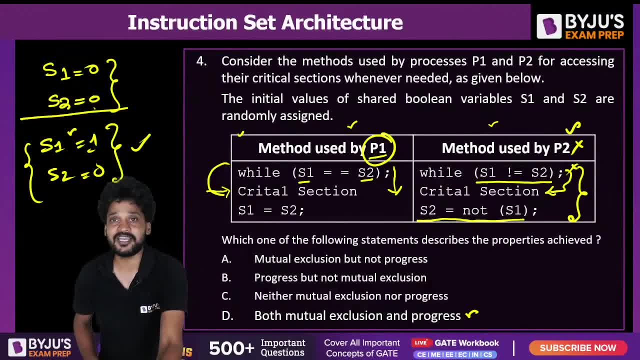 it myself clear, Sahoo, Here progress is not satisfied, Mutual exclusion is satisfied. Progress is not being satisfied. What is progress? Whenever a process wants to enter into the critical section. if there is no other process wants to enter into the critical section, the current, 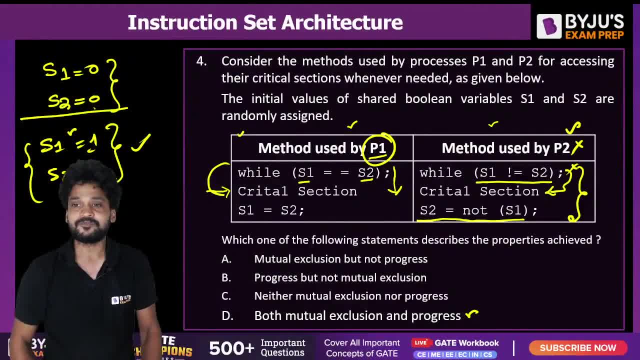 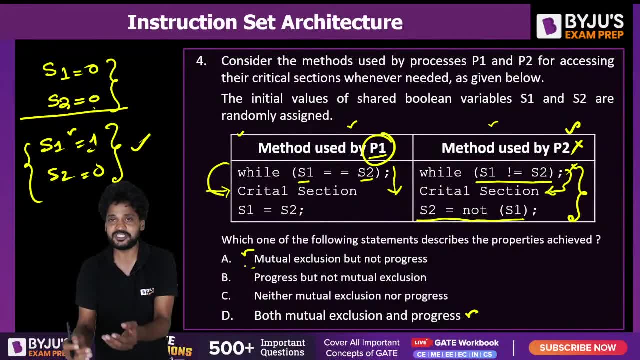 process which wants to enter should be able to enter. Got my point clear, or not? So mutual exclusion is possible. Only one process is able to enter into the critical section, according to the condition, But progress is not being satisfied at all. 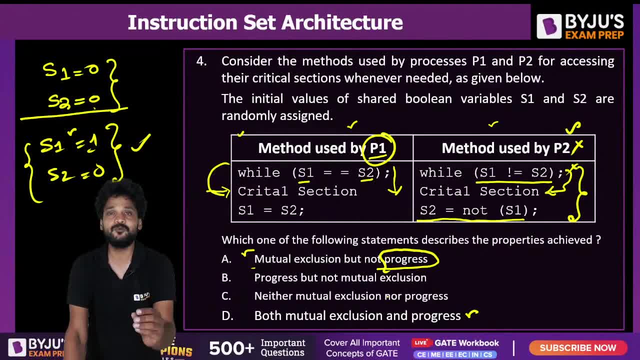 I hope I made my point clear Once again. what is a progress? What do you mean by progress? Progress means if there is only one process waiting to enter into the critical section, it should be allowed to do so Because there is no other process in the system. 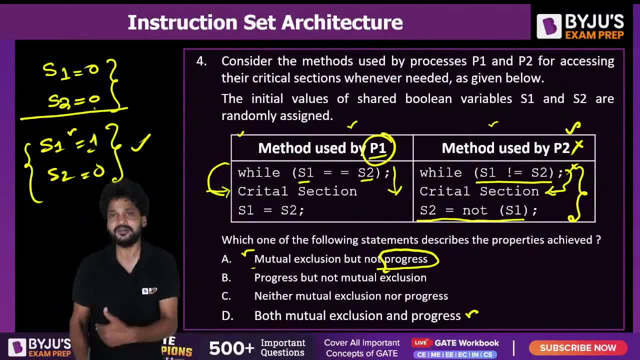 at this point wants to enter into the critical section. But here the condition has been violated: The moment process P2 comes out, it needs to wait for the P1 to enter. Unless P1 enters and sets the condition that will allow the process to enter into the critical section, 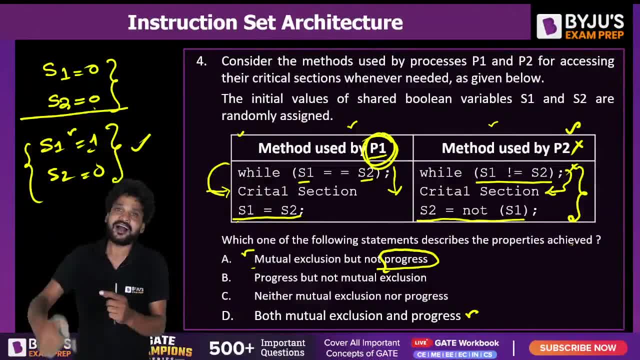 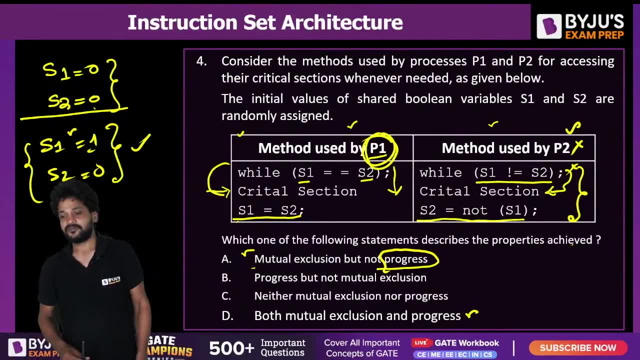 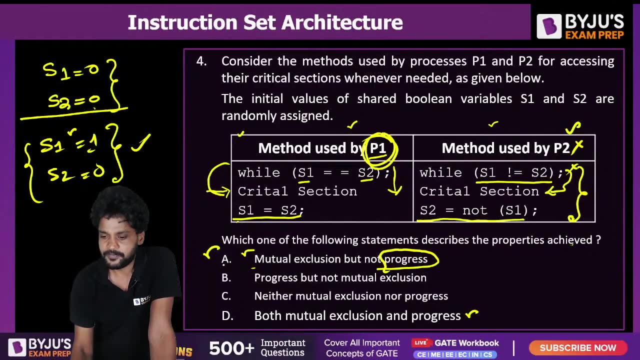 there is no other way for process P2 to again to enter into the critical section. I hope I made my point very clear, Sushant. yes, Can we go to the next question? Option A is correct. Progress is not being. 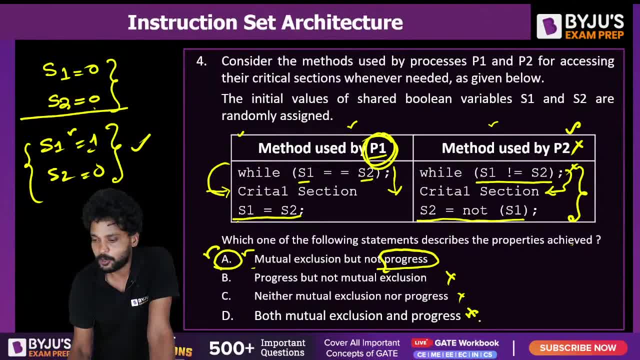 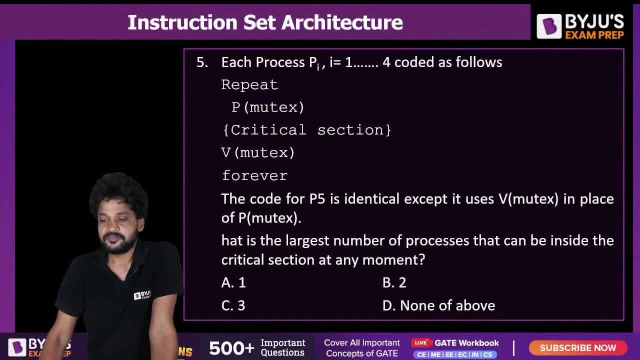 Obviously, option A will rule out all the other options. Can we go to the next question? We will take it as yes. There are several processes here. Each process- P1, P1 I- is equal to 1 to 4, coded as follows: 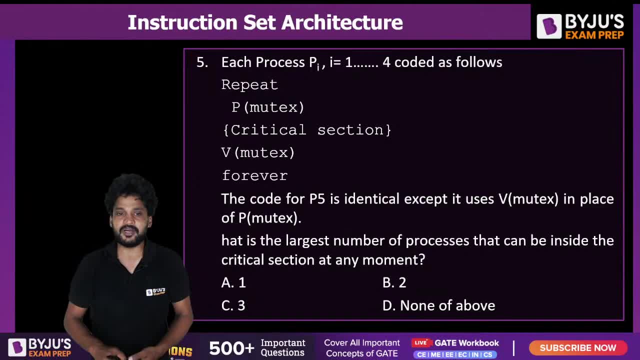 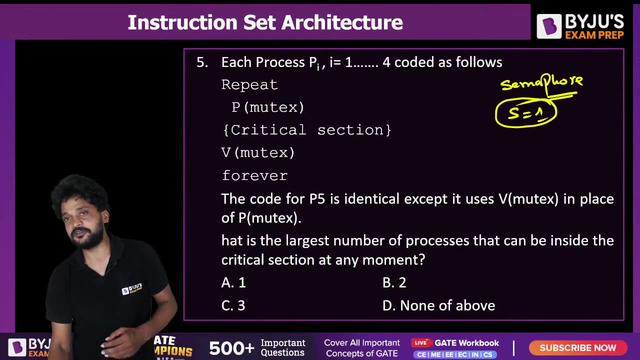 P mutex, P mutex. We are talking about semaphores here, How a semaphore to be accessed. A semaphore value S will be initialized to 1.. Right after the initialization you will be able to access the value of the semaphore or update the value of the. 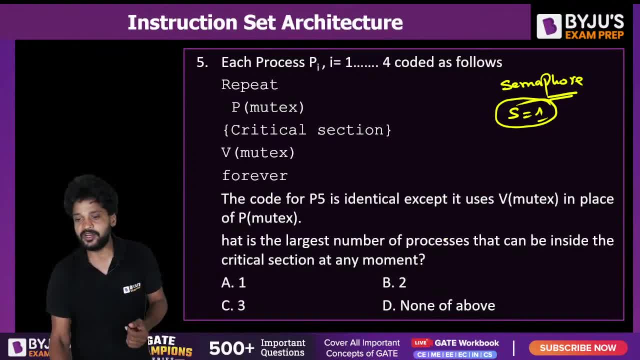 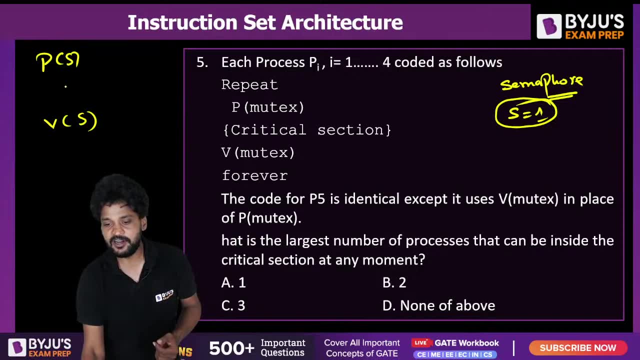 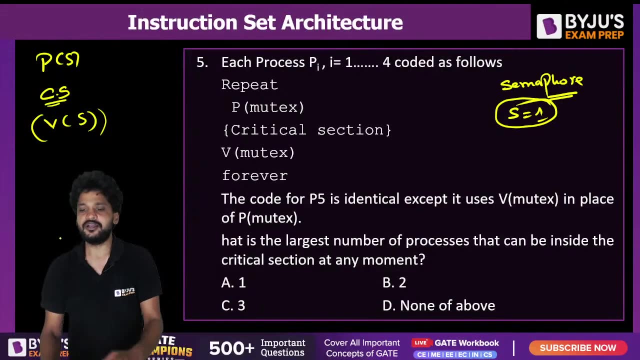 semaphore by using two methods. One is P of S, followed by V of S. If P of S is successful, you will be able to enter into the critical section. Then you need to perform V of S, Okay, So here's look at this. If the semaphores are, 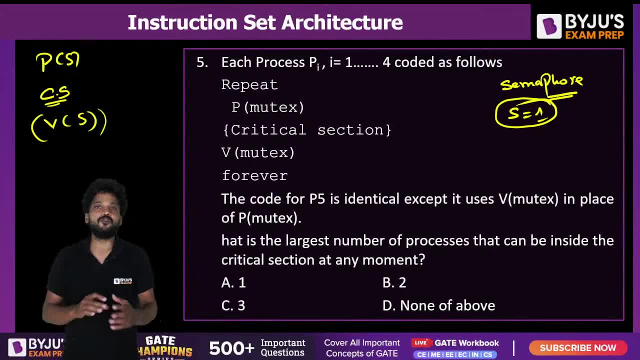 used correctly and properly, there won't be any trouble whatsoever. But if the semaphores are not used properly by the programmer, those will lead to the worst outcomes. Only the thing is, you should be able to use the semaphores properly in the same order of P of S. 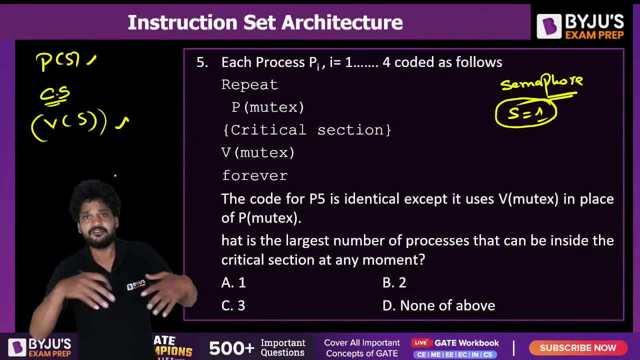 followed by V of S. If you do reverse it, there will be a lot of chaos Here. the thing is. the question is: I mean there are several processes Here within this application. there are five processes. Okay, There is an application. Let me explain. 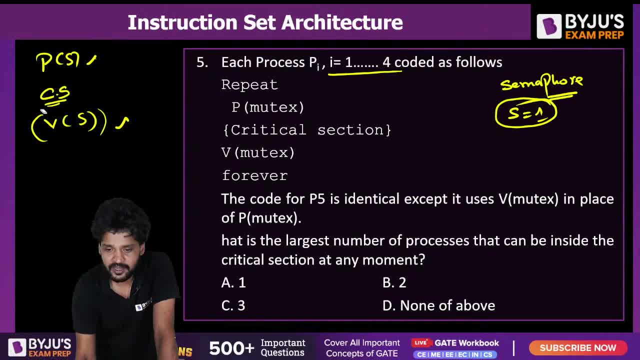 There is this: All of you stay focused. I don't want you to do anything. Please do not even try for this. I will explain. Stay focused. There is an application According to the question. there is an application. That application. 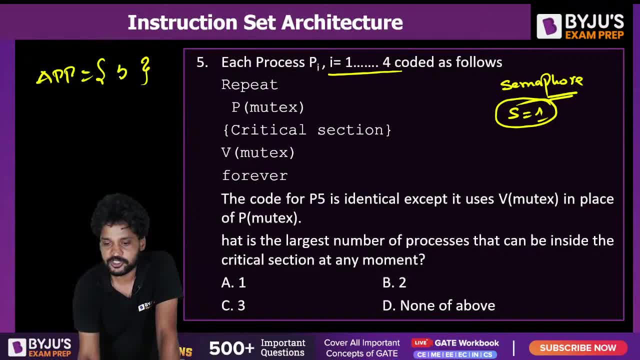 has altogether five processes. Okay, All these five processes are cooperative processes. I mean linked with each other, Connected to each other, Meaning all these five processes has a shared memory region. When this is set to be shared memory region for all the five processes, 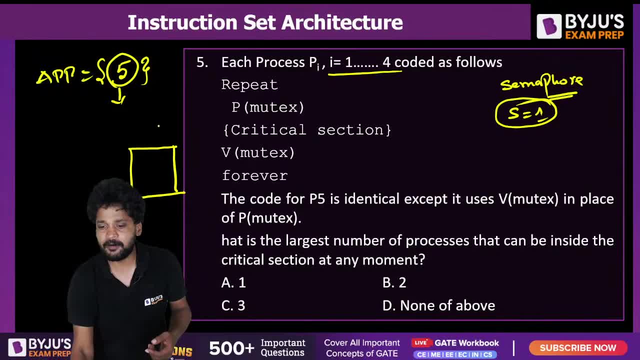 obviously any of these processes will update, can update this shared memory region, But shared memory region should be updated by only one process at a time. It can allow any process can update the shared memory, shared memory region from these five processes, But only one process should be. 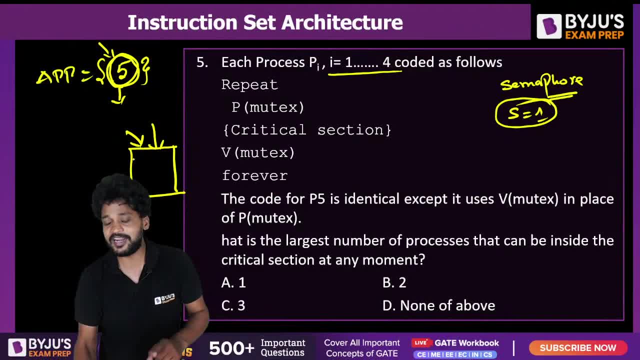 allowed to access the shared memory and update it at once. Okay, So for this, let us understand. All the other processes from 1 to 4. critical section has been protected with P of S, followed by V of S. P of S is just mutex, It's a. 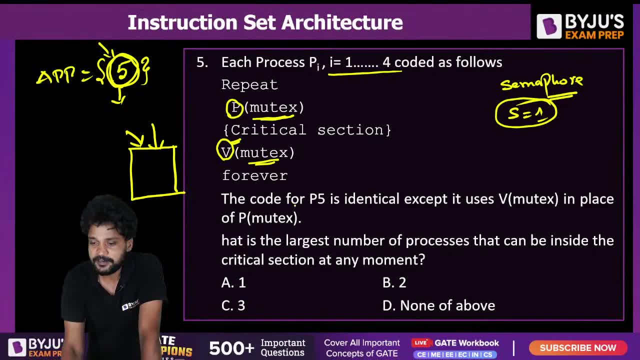 semaphore: mutex. Okay, But for the code P5, identical, except it uses V of S in the place of P of S. So let us understand. There is a small mistake done by the programmer. He did not use the semaphores in a right way When he did not. 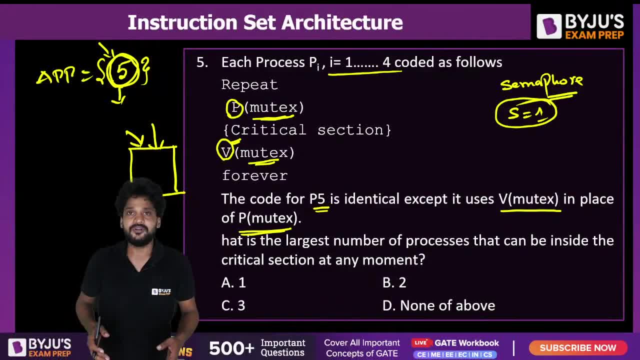 use the semaphores in a right way, in the correct order, there will be a chaos. What is the option? A, B, D, C is correct. None of the above is correct option, But let me explain why. Okay, I will. 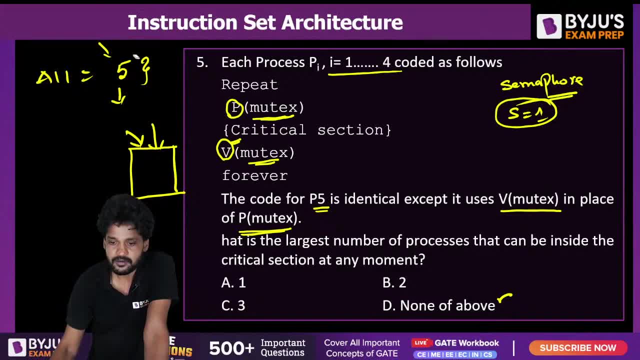 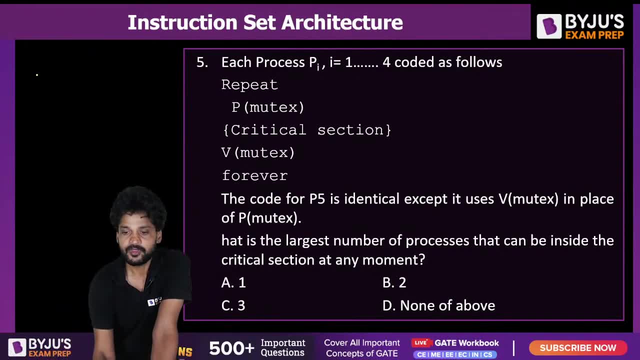 demonstrate with. I will demonstrate with the complete scenario. Let us say there is process P1. A process P1, initially we will put the semaphore mutex value. I would say mutex, Mutex value is equal to 1, right Initially, semaphores values. 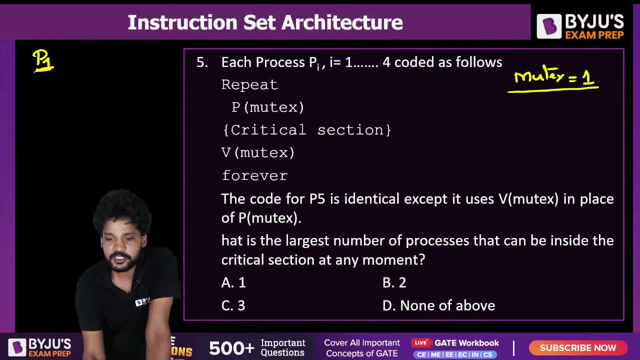 are initialized to 1.. Got me When, let us say, process P1 wants to enter into the critical section. So what it does? It performs P of mutex. When P of S is being performed, mutex will be equal to 0.. 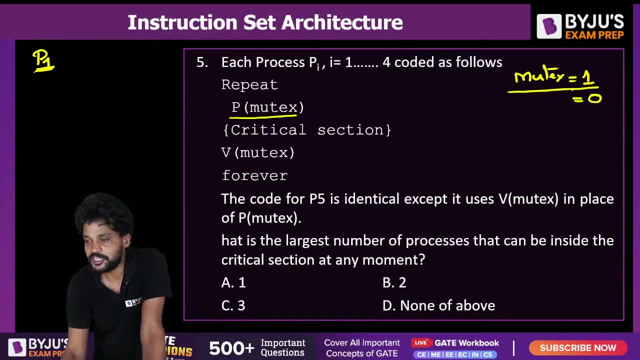 S minus minus will be performed right. So mutex minus minus is equal to 0. So after setting it to 0, process P1 can be able to enter into the critical section. Okay, This is my critical section. Now, after performing P mutex, the process. 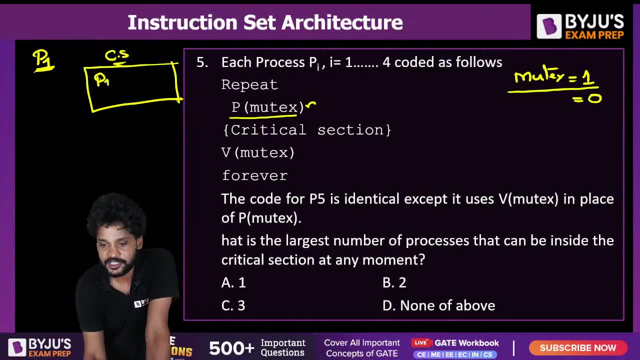 P1 enters into the critical section. Now critical section has one process, that is P1.. Now understand carefully When you talk about process file, Process file using V of mutex, followed by the critical section, followed by V of mutex. That is what I have given in the question For the process. 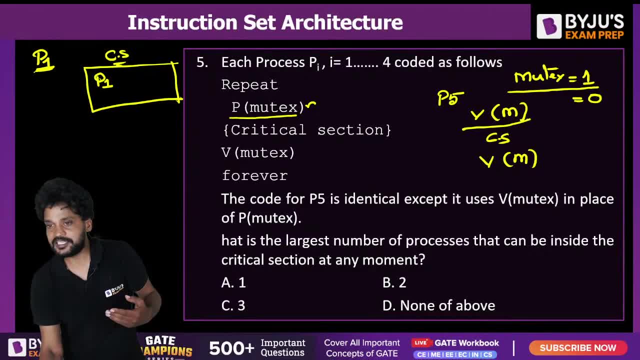 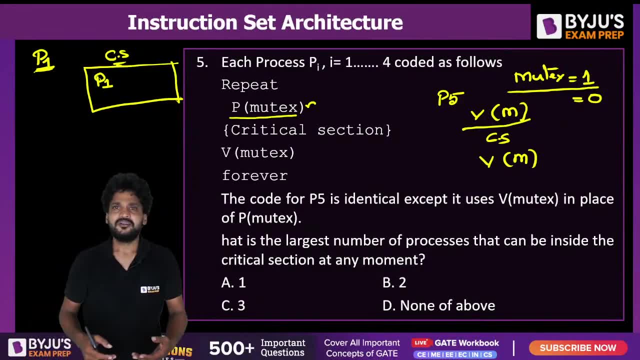 P, file V is critical section is being protected with, of course, semaphore value is always equal to 1, right, It is understood What is the semaphore? initialized initialized value, initial value. Semaphore initial value will always be equal to 1.. 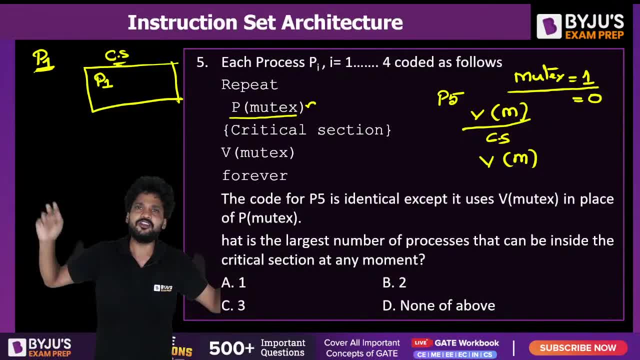 Am I right, Or do we have any other value for semaphores? A binary semaphore value will always be equal to 1.. Yes or no? Yeah, So let us say process P5.. Before enter, let us say: right after P1, process P5. 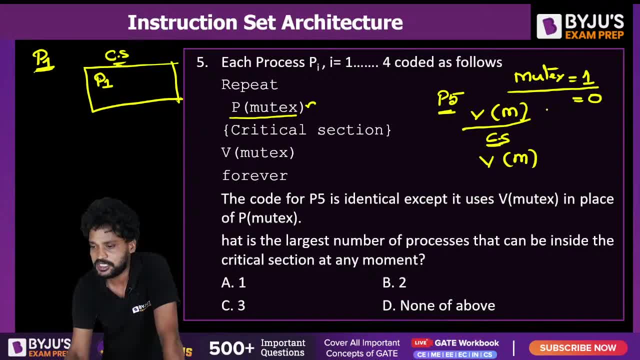 comes into the CPU. So before it enters into the critical section, it will execute V of M. When V of M is performed, what will happen? Mutex plus plus will get performed. So by making mutex value 1, process P5 will be able to enter. 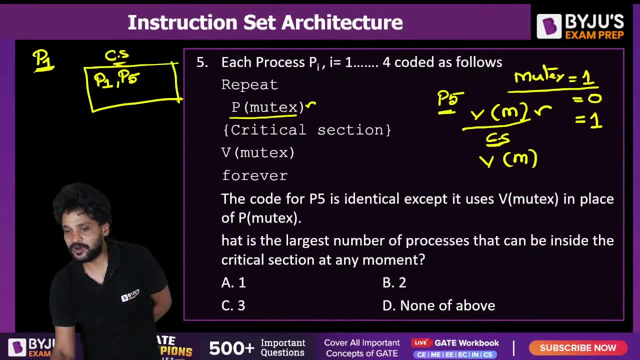 into the critical section Now, as the mutex value is equal to 1,. let us say, now there is one more process: P2.. If it wants to enter into the critical section, it will be able to do so, because when the mutex value is equal to 1,, 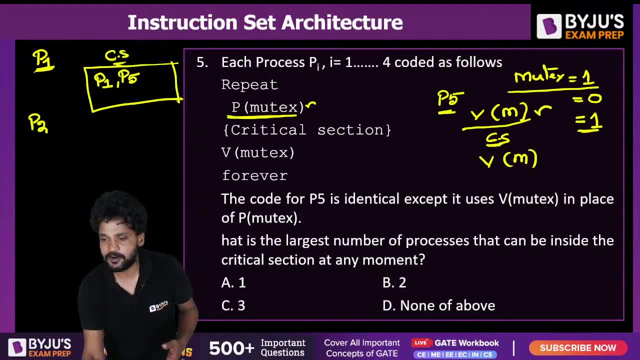 you know, P of S, all the other process performing the right operations on the semaphore, that is P of mutex. P of mutex is S minus minus. When S minus minus is being performed, obviously semaphore value will get decremented. Then P2 will be able to enter. 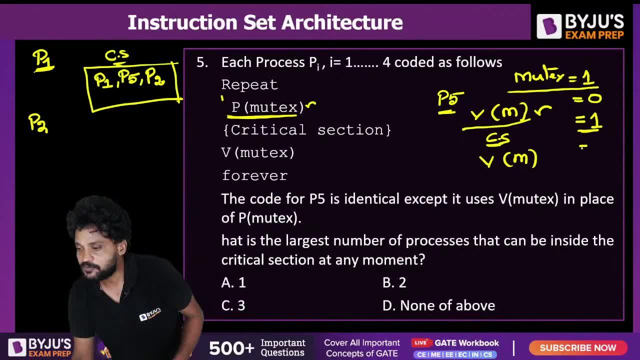 into the critical section, which will make the mutex value again equal to 0.. When it is equal to 0, let us say my P5 wants to come out of the critical section. Obviously it will execute V of M, making mutex value equal to 1.. P5. 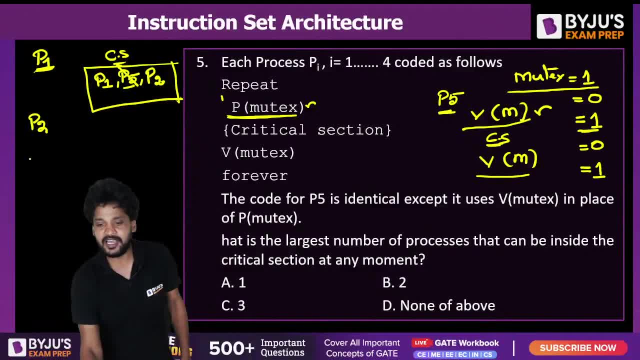 came out of the critical section. It will allow one more process, P3, to enter into the critical section by performing P of mutex, by making 1 to 0. Again, when P5 comes, P5 can come in. So that means that if it iterates any, 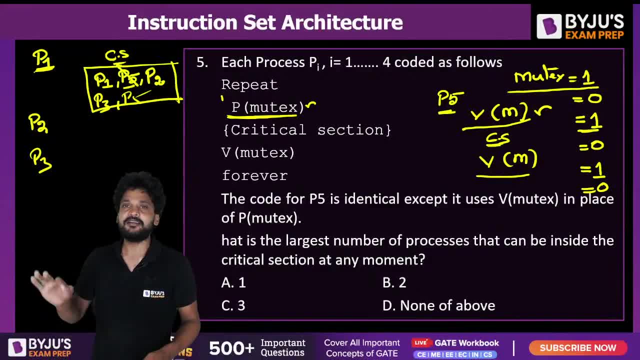 number of processes can be in the critical section. Did I make it myself clear or just It will be followed Again: P5 will come. When P5 will come, it will be equal to 1.. When it is equal to 1, one more process, say P4,. 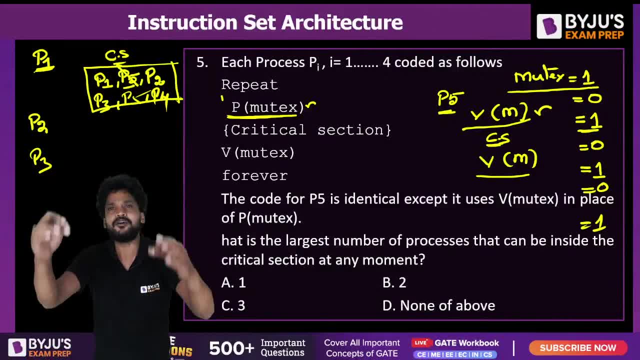 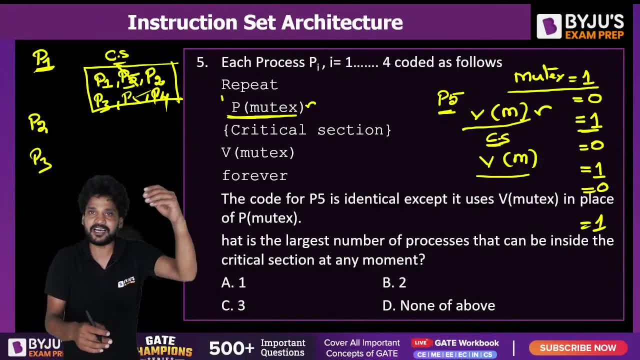 can be in the critical section, Yes or no. All the processes will be able to enter into the critical section because a small mistake has been committed by the application developer, because in the five processes, in protecting the critical section, actually he reversed the operations on the semaphores. 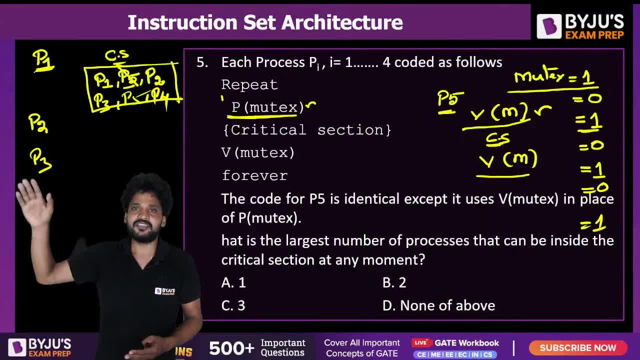 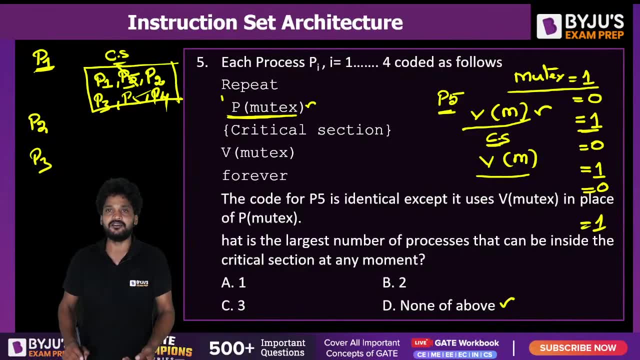 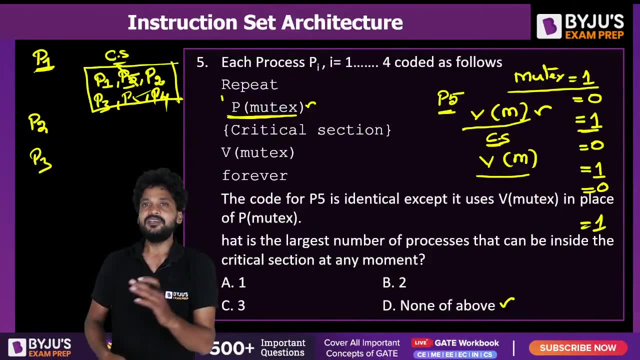 V of M, followed by the V of M. he stitched with the fifth processor, critical section. So what is the option? None of the above, as interpreted by the ABWs, is correct, because total five processes can be in the critical section at the same time. Is it making? 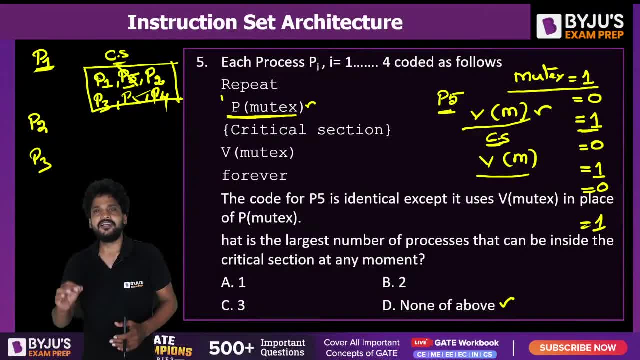 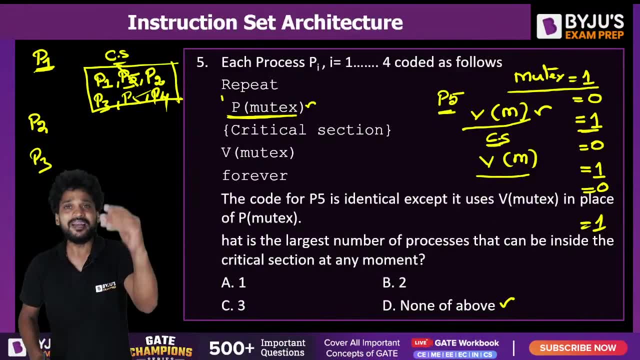 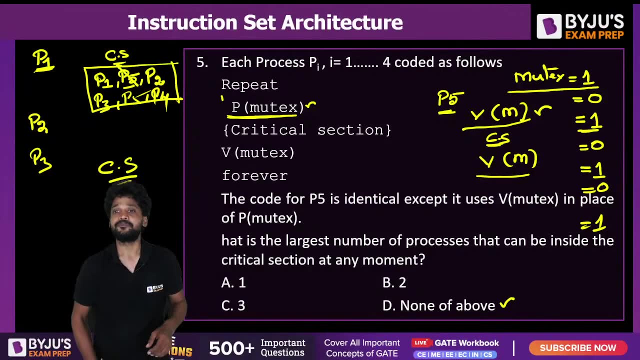 any sense. Yes or no, It makes a perfect sense. You cannot use the semaphores differently. Semaphores are to be used only in the order of the operations. When you have a critical section, use the semaphores, no problem. 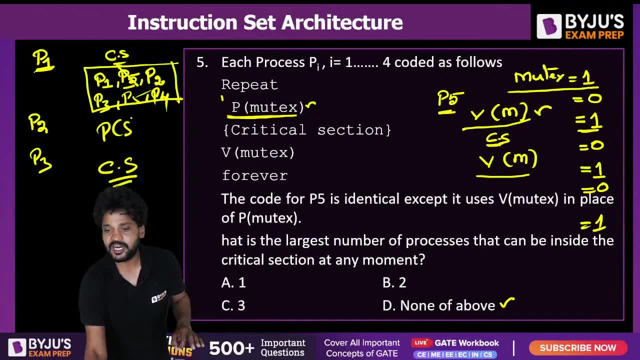 Use the semaphores, no problem. but initially you start with P of S. right after you perform the critical section, you need to end with V of S Being an application developer. your critical sections of all the processes must be protected with this order of P of S, followed by: 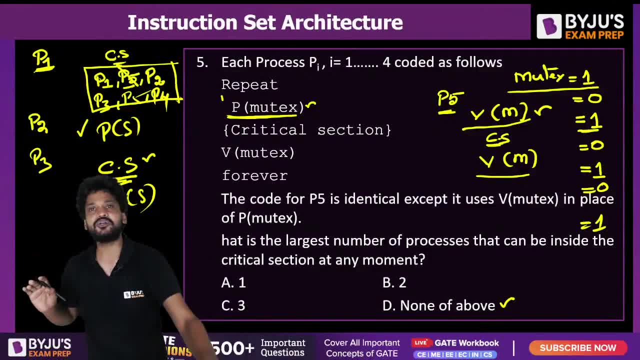 the V of S. Any change will lead to a worst consequences. The example is on your screen. A small, minor problem, because understand carefully who is an application developer. You are an application developer, I am an application developer. We people are the human beings. 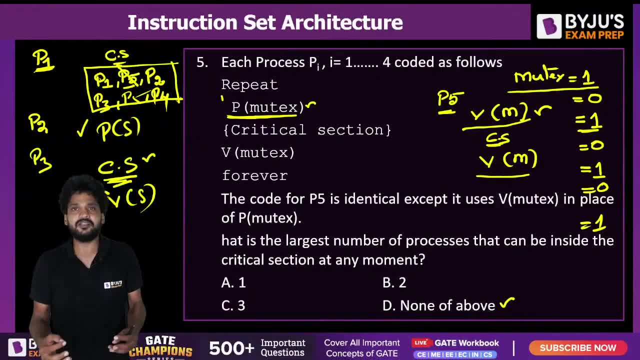 Our tendency is to commit to the mistakes, because when we overwork obviously we may not remember what we have been doing. When you are working late night at 12.30,, of course, software job is not a regular job as in the teacher, 8.30 to 4.00, no. 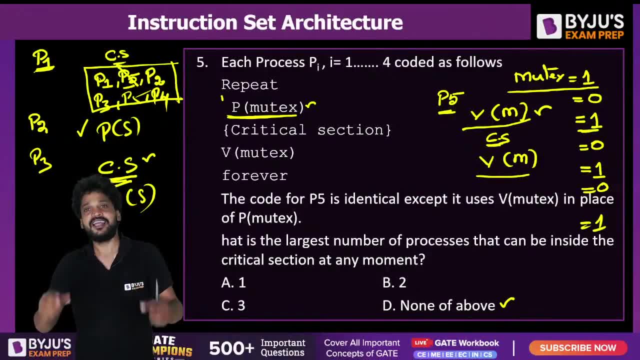 Obviously, you have to work at 11.30 or 12.30 in the night. At that time you should be able to protect your critical section. Not only five processes. trust me, when you develop an application, there will be hundreds of cooperative processes. 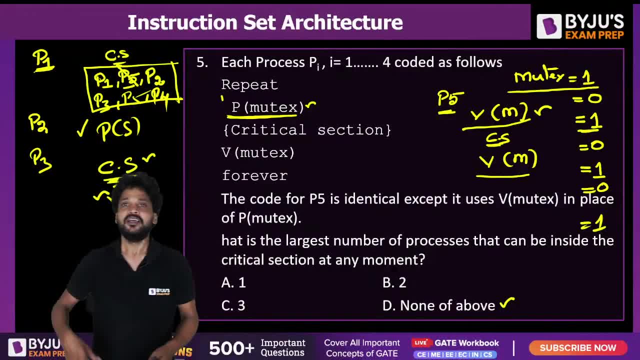 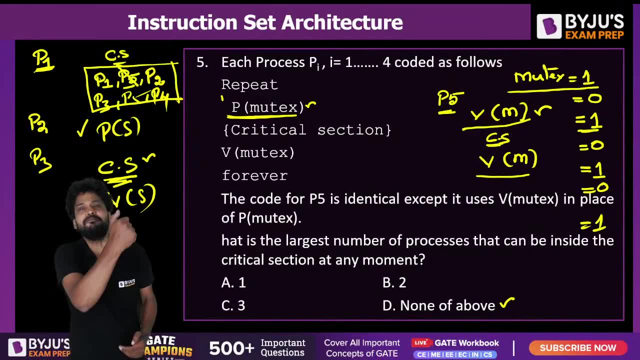 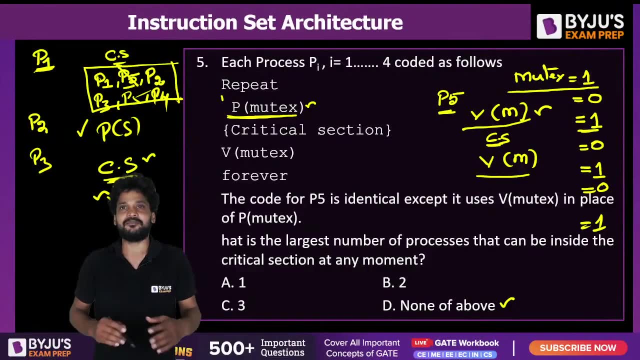 For all those hundreds of processes there will be critical section. All those critical sections must be protected by the semaphores. Obviously, we may commit to some mistakes, right But- but mistake is a mistake. I mean, this is mistake, doesn't look. I mean. 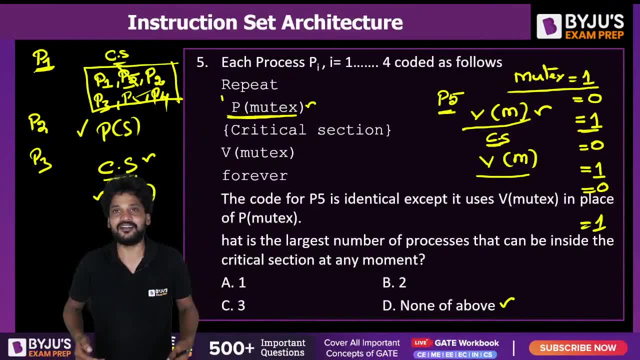 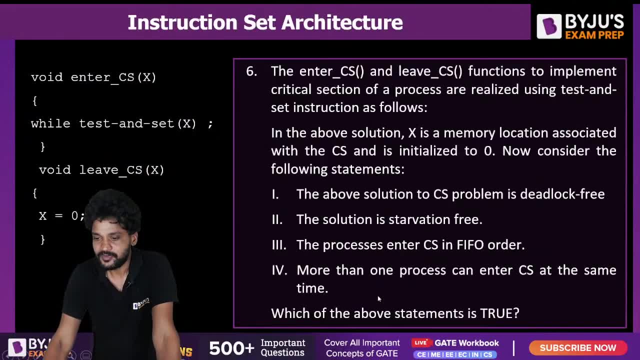 it doesn't consider the factors that led us to mistake. right Mistake is a mistake that must be corrected. Yeah, Answer will be 5 for this question. Next one is on your screen. Next question is on your screen: The enter. 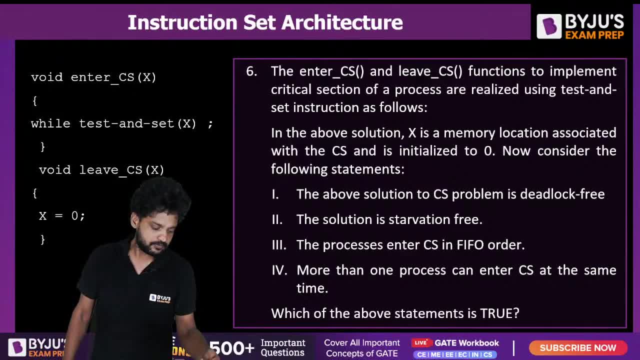 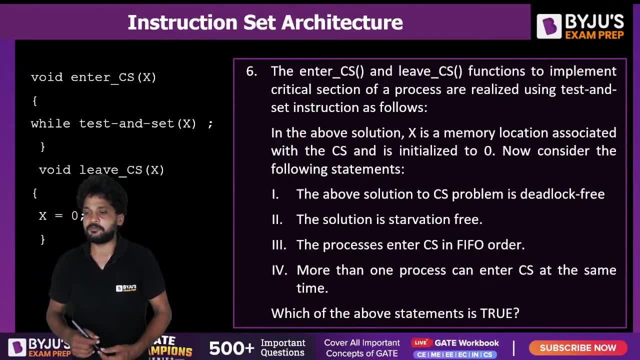 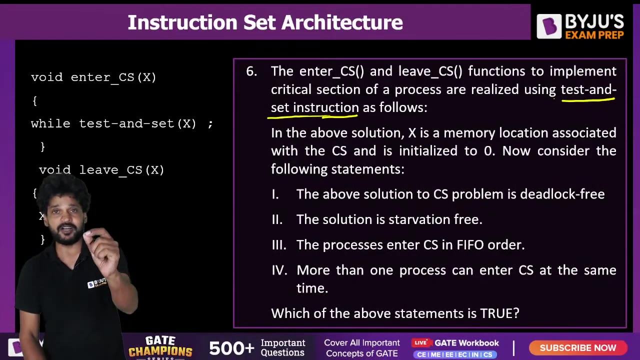 excuse me, Yeah, The enter CS and leave CS functions to implement critical section process are realized by using test and set instruction. What is test and set instruction? Recall all those people who are following my YouTube sessions and the app sessions, operating systems especially. 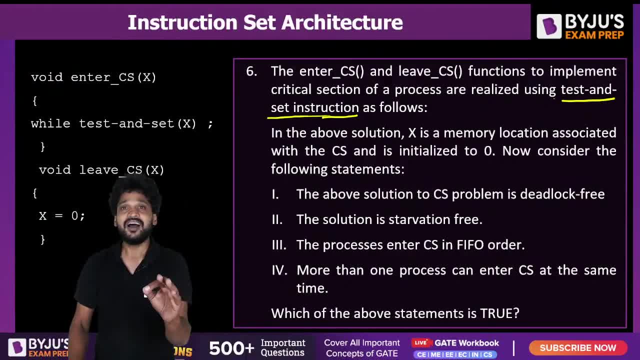 they know what is test and set lock. Test and set lock is a hardware lock to protect the critical section. Tell me what are the ways to protect the critical section? The first one is paiders and solution. right, First one is paiders and solution. 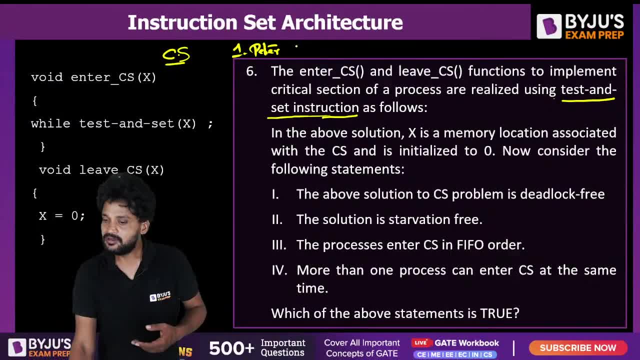 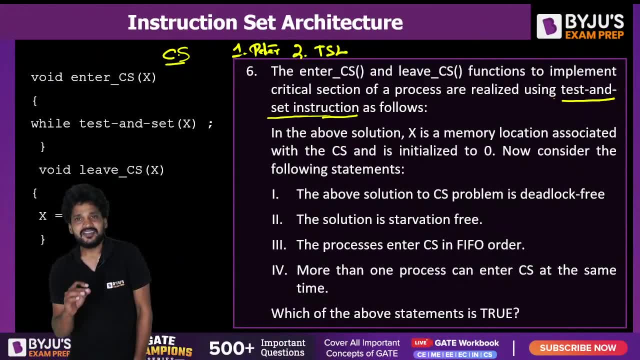 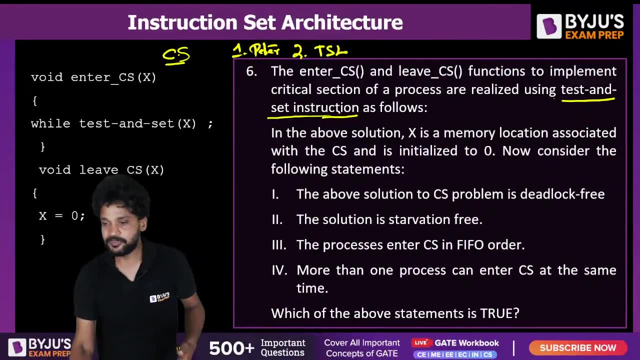 But paiders, and solution cannot be used in modern day architecture. So we can use test and set lock, which is a hardware method. But a hardware method has some shortcomings. Hardware method is not transparent to application program developers, So for that we use what you call. 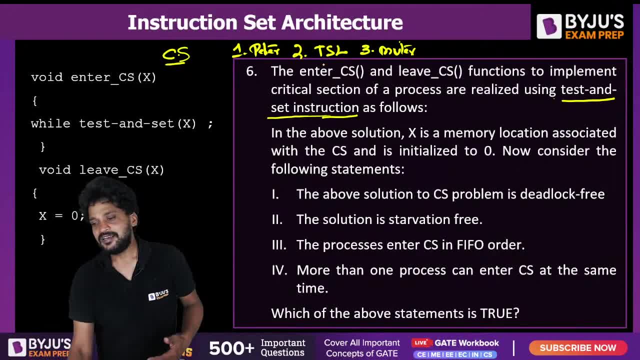 mutex locks, which is a software method, But either paiders and solution, or test and set lock, or mutex locks- whatever the lock that you are talking about- are having some shortcoming, which is called a busy waiting. To avoid the busy waiting, we introduce the semaphores. 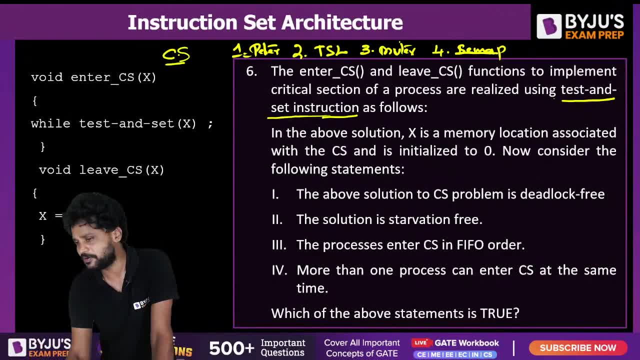 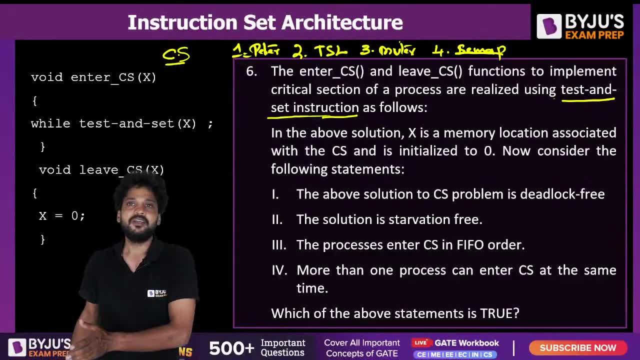 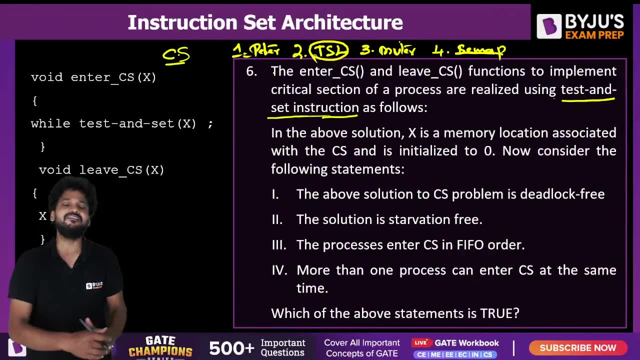 So these are the best solution. Semaphore is perhaps the best solution among any other solution, But there are shortcomings, even in the semaphore, but those can be overcome very easily. So we are talking about a test and set lock, which is a hardware lock. What is the property of a hardware lock? 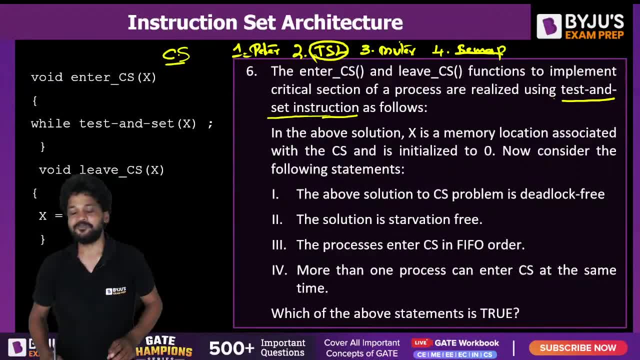 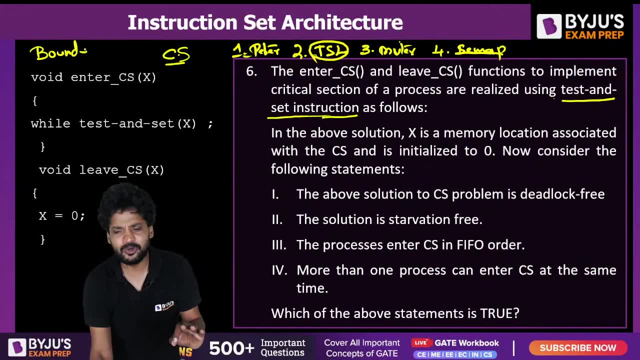 The property of a hardware lock is very simple. This test and set lock will satisfy only bounded waiting. Got me You don't need to look at any other thing. Test and set lock will only satisfy bounded waiting. Will allow only one process to enter into the critical. 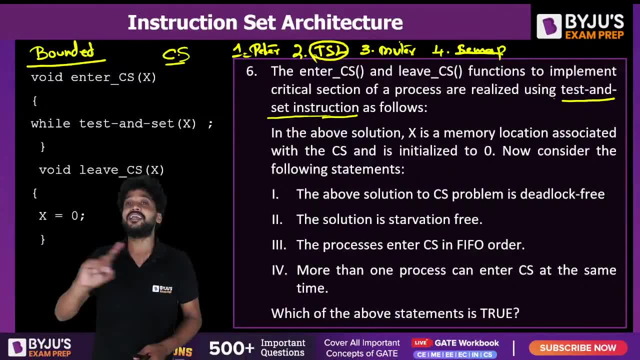 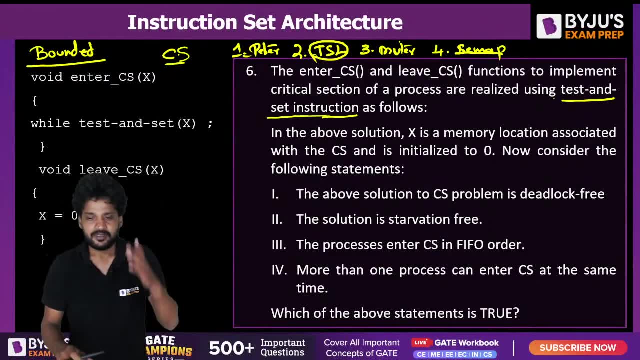 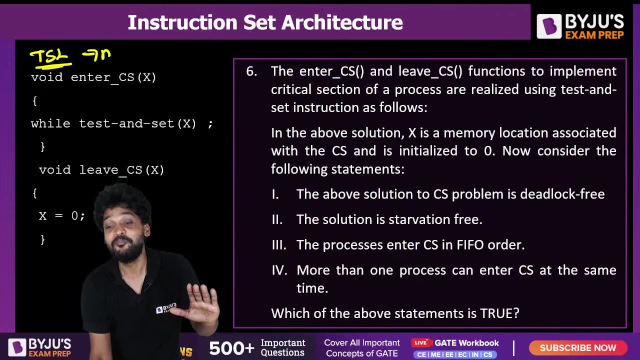 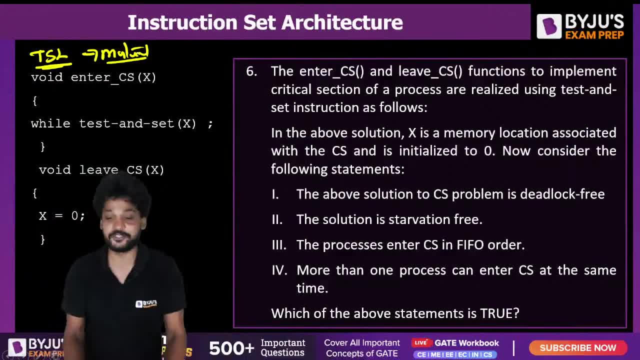 when we do our work we forget our silly little things. Test and set lock will only satisfy mutual exclusion, Okay, But it doesn't satisfy bounded waiting or progress. Progress and bounded waiting will not be satisfied by the test and set lock. Understand carefully. 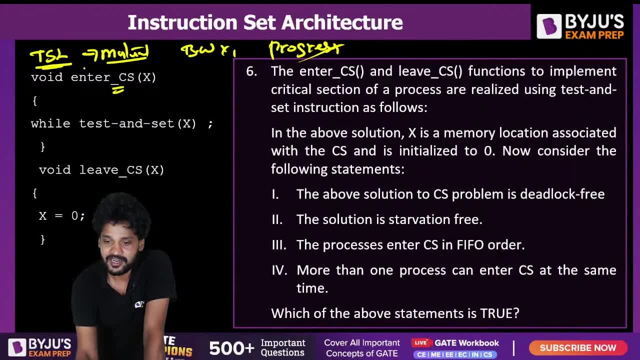 So, before entering into the critical section, it will execute, Enter, it will test and set the lock x. then, if it is successful, it will enter into the critical section. otherwise it will loop around. So, in the same light, which are the following are possible: The above solution. 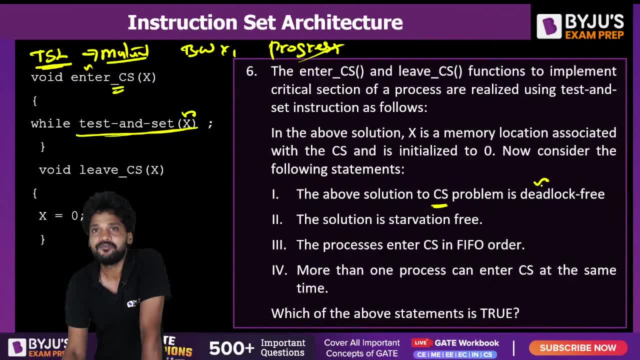 CS problem is deadlock free. Obviously, if mutual exclusion is satisfied, bounded, sorry, deadlock. there is no chance of deadlock. If the mutual exclusion is being satisfied by any solution, then we can say that it is deadlock free, But the solution cannot be treated as starvation free. 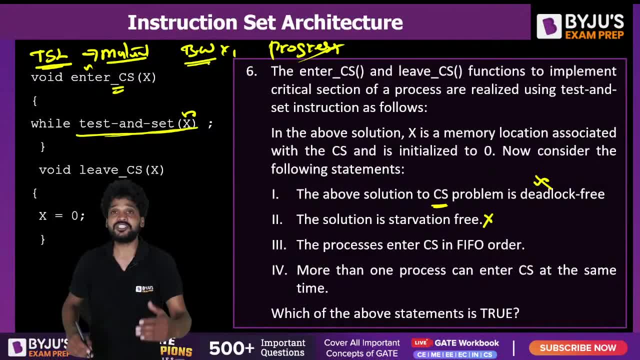 Because bounded waiting is not satisfied. a process can re-enter into the critical section as many times as it want, When, as long as the lock is available, Okay. So the solution is not starvation free. The process enters CS into the P4 order. There is no guarantee. 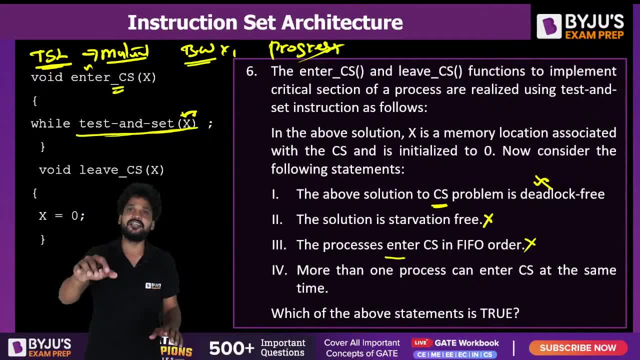 that a processes, all the process enters into the critical section in the P4 order And more than one process can enter into the critical section at the same time. No, It is also not possible Only one process By using the test and set lock. 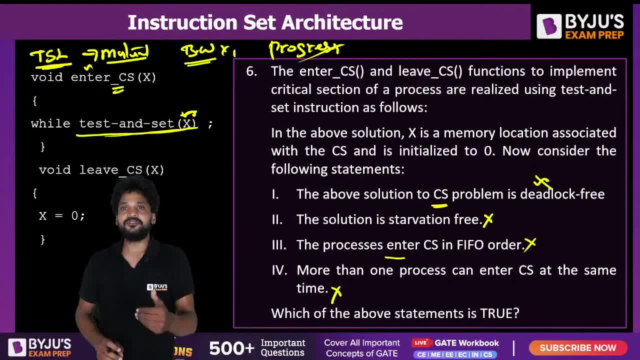 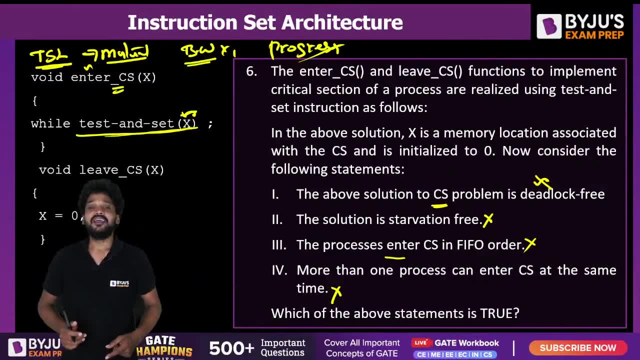 the first two criteria, which is which is mutual exclusion, can only be satisfied. When the mutual exclusion is satisfied, only one process will be in the critical section. all that time, I hope I made my point very clear. So only option one is correct. Option one is correct, right. 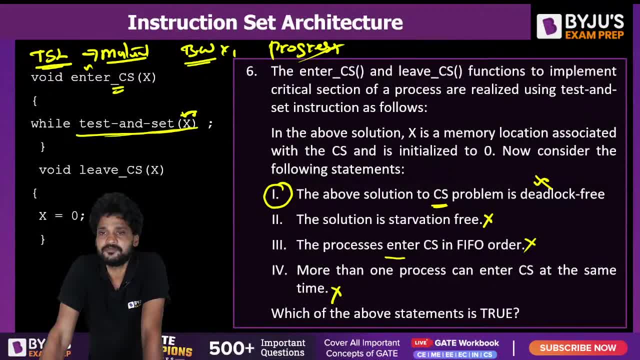 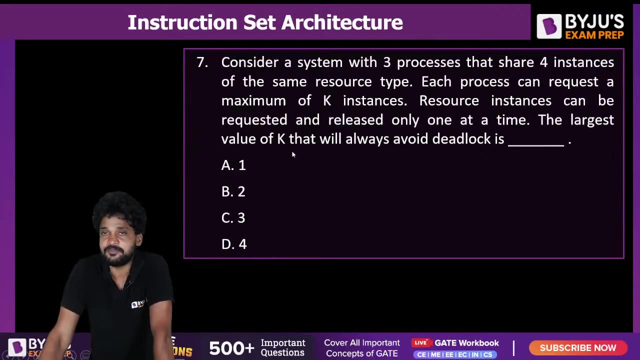 Am I right or not? Everybody believes. Am I correct or not? Can I go to the next question? Yeah, So here, only option one is correct. Consider the system with three. This is about deadlocks. This is about deadlocks. 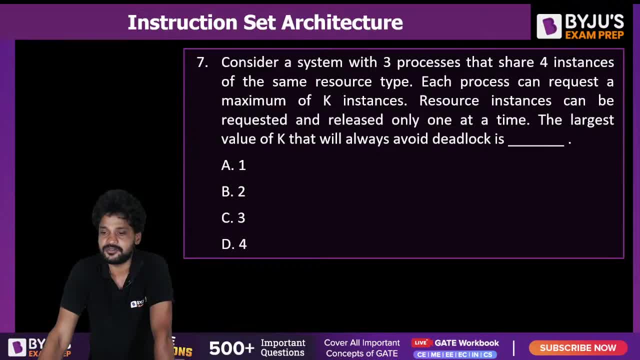 Consider a system with three processes that share four instances of same resource type. Each process can request a maximum of K instances. Resource instances can be requested and released only one at a time. The largest value of the K will always avoid a deadlock. is what? 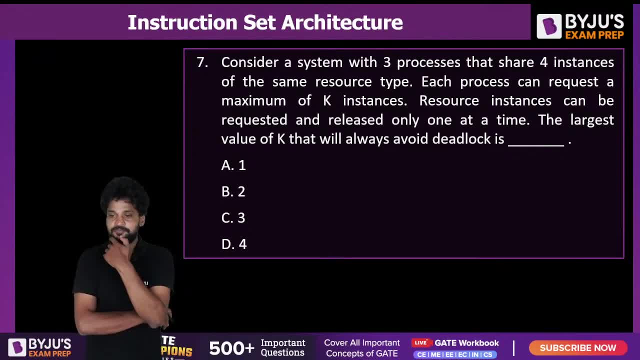 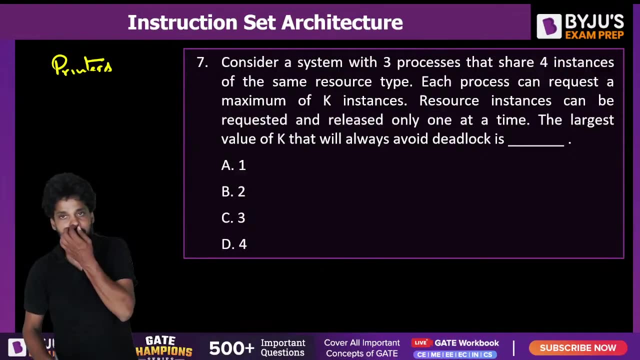 This is the question. The question is simple. System has several resources, Instance of. let us say, system has several printers. There are several printers, but the number of printers is unknown. according to the question, The number of printers- I am taking the resource type as printers. 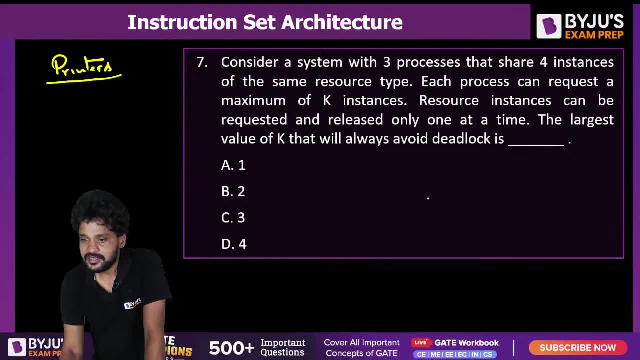 Okay, And there are three processes. Yeah, Printers also is given. There are four printers and there are three processes. Each process can request a maximum of K instances. Number of instances that are required by each process is not known as of now. 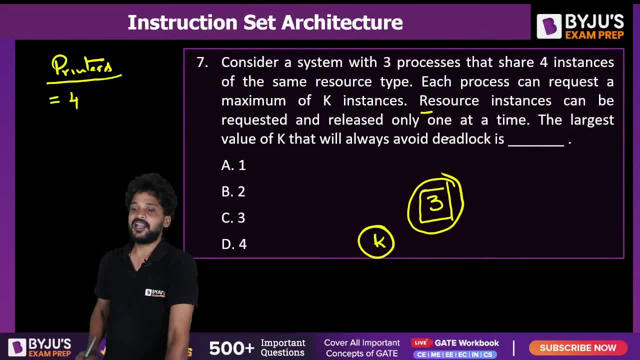 Resource instances can be requested and released only one at a time. The largest value of K will always avoid a deadlock. is Now system has. system has four printers right. Let me tell you a simple way to calculate the number of instances that can be requested by each process. 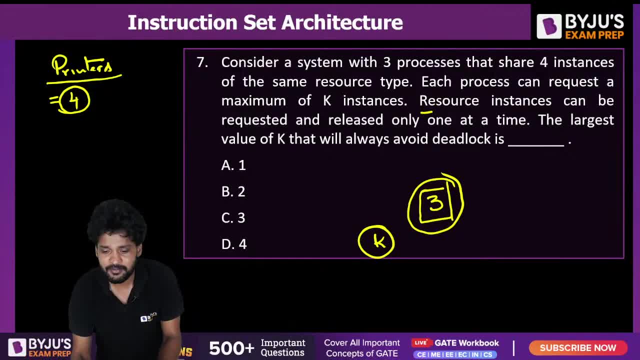 In order to avoid a deadlock. there is a fundamental rule to be followed. There is a fundamental rule to be followed. What is the fundamental rule? Any process. let us say there may be n number of processes Out of this n number of processes. 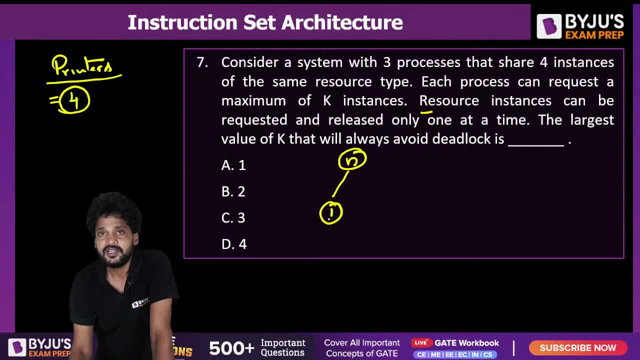 for one process, the system should be able to provide all the resources that it is requesting. For instance, in order to avoid a deadlock, system needs to have sufficient number of resources. How many? How many? For the first process, it should be able to support. 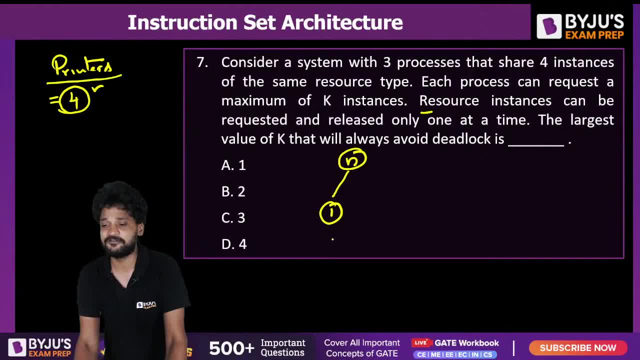 it should be able to provide all the instances that it is requesting for All But remaining n-1 processes, remaining n-1 processes. it should be able to provide the requested resource minus one. Let us say in a simple example, there are four processes. 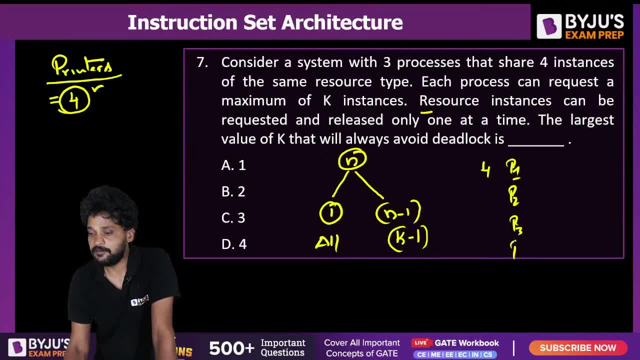 P1, P2, P3 and P4.. All are requesting for two instances of resources. In order to avoid a deadlock, system needs to have the number of resources which are equal to to satisfy the requirement of at least one process, that is, two. 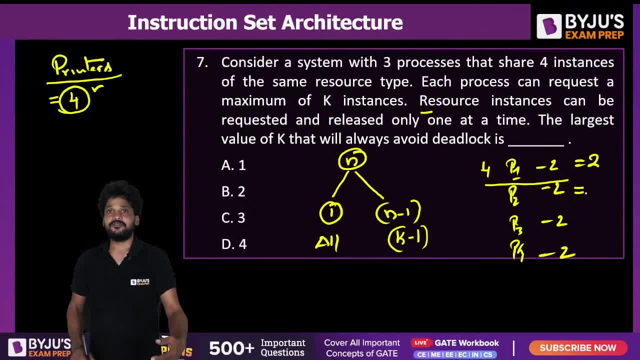 plus to satisfy the requirement of the maximum resource requirement, minus one for the other process. So it is one, it is one, it is one. If each and every process is requesting for two resources, system will require to have at least five resources to avoid. 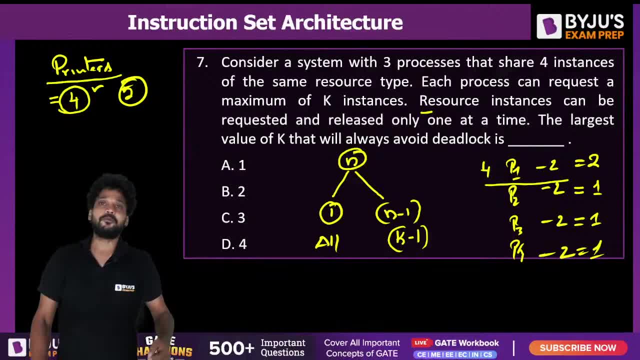 a deadlock, in case if we have four processes. Now the thing is in this same life. what is the answer for this? What is the answer for this? Okay, Let us see if each of three processes there are three processes, let me. what is the answer? 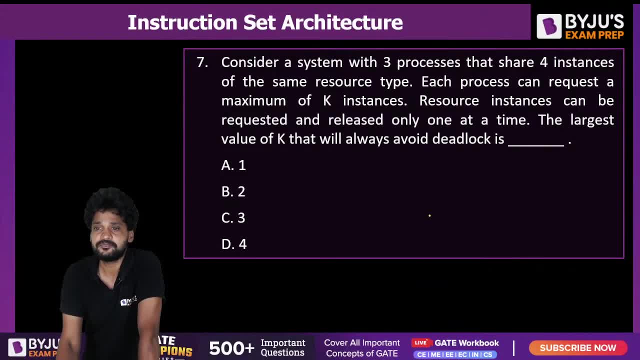 for this Abitabulous. What is the answer for this? Three processes, Let us say, each of this process requesting for one resource, But total number of printers are equal to four. Obviously, one will not lead to a deadlock, Okay, Two. 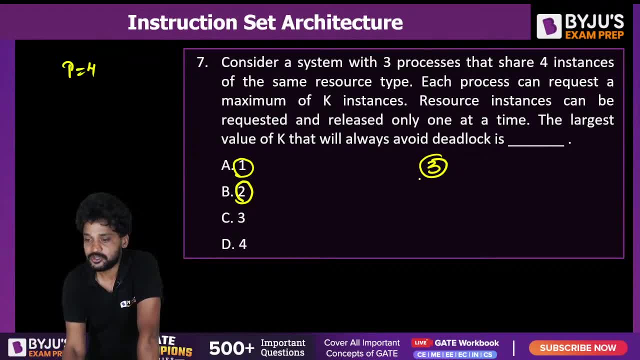 Each of the processes requesting for two resources. So first process can be given all the resources. Next, two processes will get only one resource, Okay, Next, If each of the processes is largest value of k. If each of the processes is requesting for three, 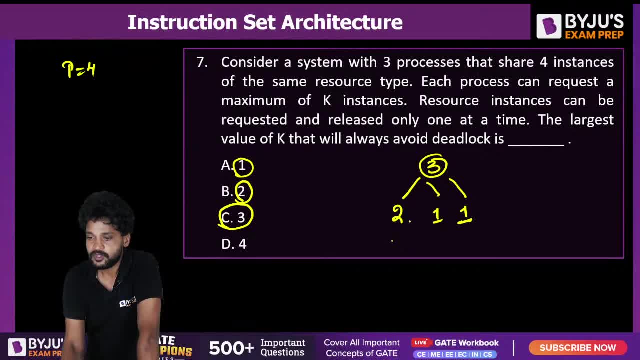 resources. first process will be given two. Yeah. Three is correct. When each of the processes is requesting for three resources, this is correct, right. One process will be given. No. Excuse me, Maximum value can only be two right. Correct me if I am wrong. 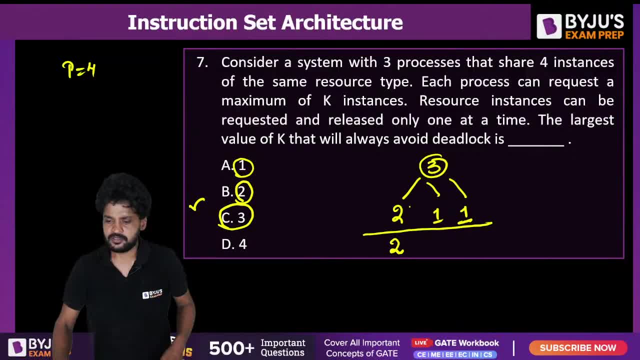 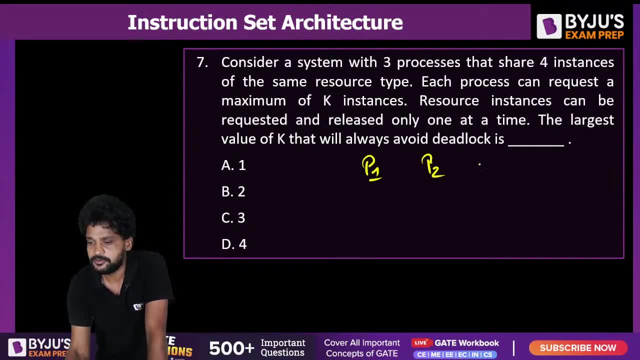 Okay, Or what is there? There is process P1, process P2, process P3.. The total number of four instance of the same resource, Total number of printers, are equal to four If, let us say, three resources are being requested. 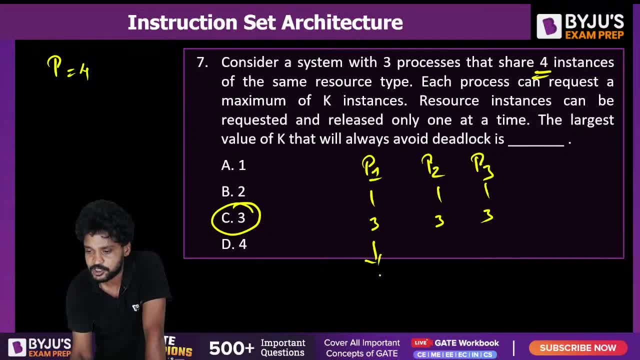 Three, three, three. At that time, first process should be provided with three. Next two processes should be provided with only two. System need to have a total of seven resources in order to satisfy all these. you know the type, right, So? 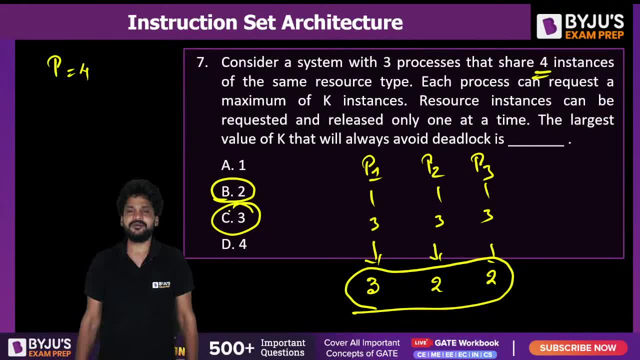 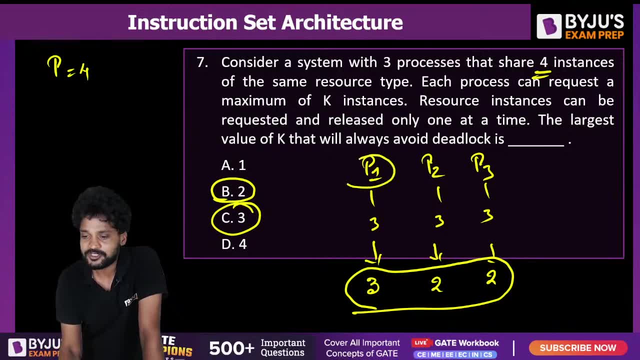 option B is correct. Am I right or not? System need to have the sufficient number of resources to provide at least one process: total request plus total request minus one for the other process. Correct me if I am wrong. Option B is correct, right. 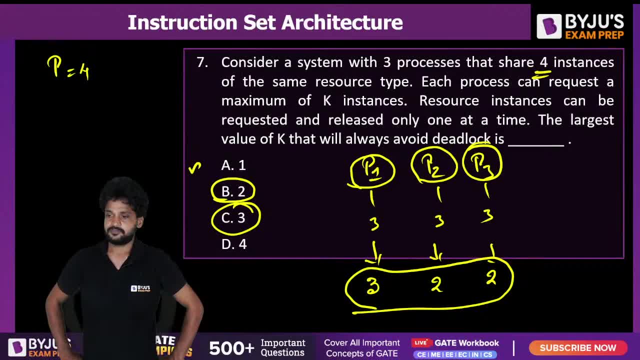 Okay, Two is correct right. Option B: two is correct. Neel Madhav, is two correct? or is C correct, Three correct? No, It is just two. More than two processes, sorry. more than two resources are requested by any process. the system. 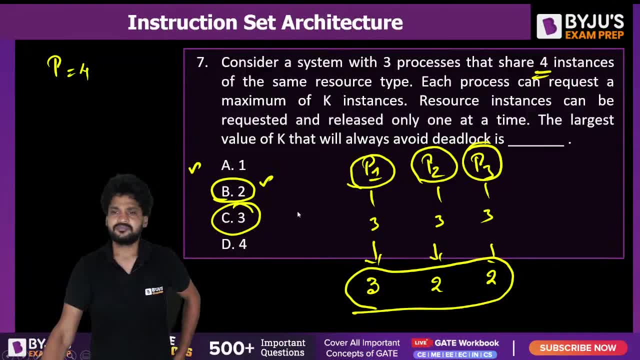 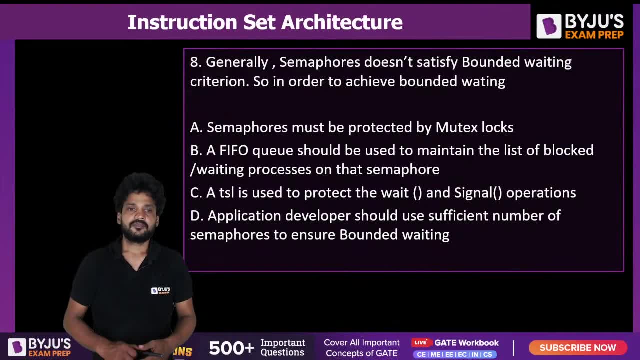 will enter into the deadlock, Yes or no? Can I go to the next question? Make it clear, or, Neel Madhav, I am waiting for your answer. Did you understand why? or you want me to repeat it again? the previous question. 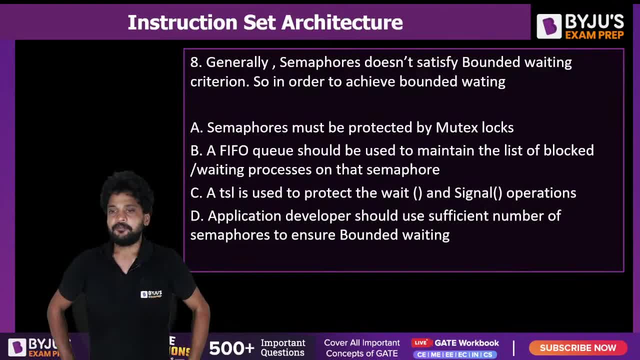 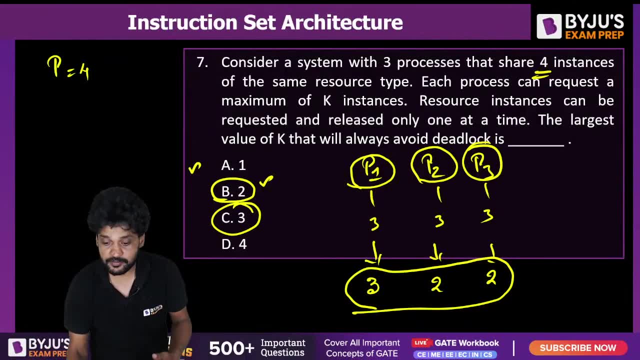 Srihita, are you there? Yeah, Next question is on your screen. which is on your screen Again. fine, That is what I want. That is what I want. Okay, Let me erase this. That is all in. 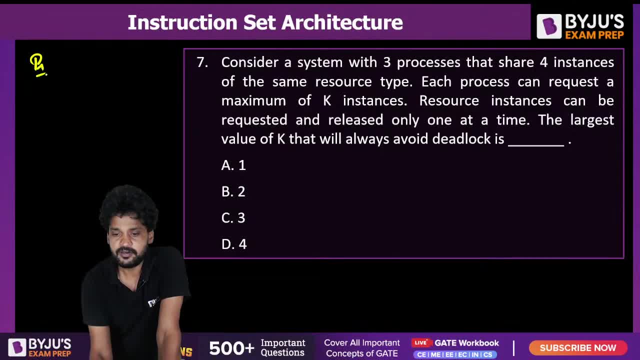 There are three processes: Process P1, Process P2, Process P3.. Okay, All the processes may request for some m number of resources. Okay, Now the thing is, in order to avoid a deadlock system, our CPU should be provided with sufficient. 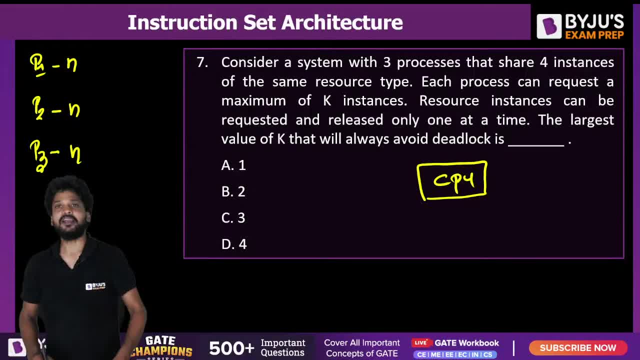 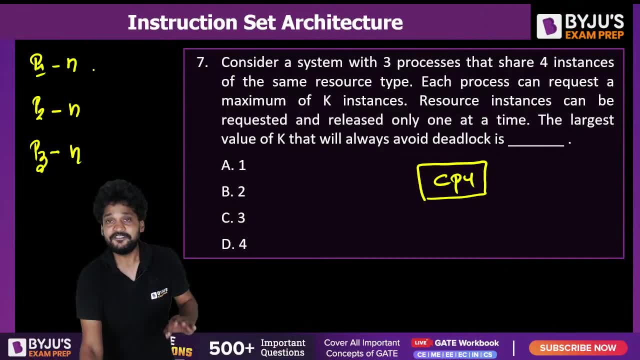 number of resources. How many are sufficient? Simple, If these are coming up with n and n, each system needs to have sufficient number of resources in such a way that it satisfies at least one process- total resource requirement. The other process- total resource requirement. 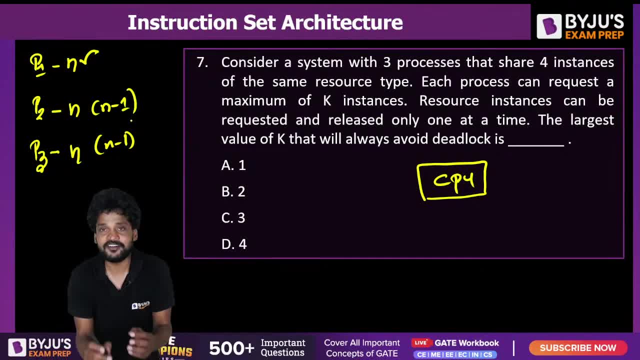 minus one. Okay, If these many number of resources are available with the system, then we won't enter into the deadlock. Otherwise, there will be a deadlock. Okay, Let us see. The total number of resources are just equal to four If these: 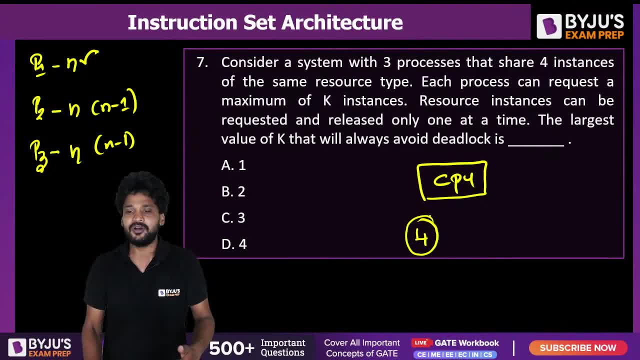 are four. the maximum possible value of n is equal to two. Each of the process can request for a maximum of two resources. Then it will be sufficient. The four will be sufficient because for first process I will give all the two resources For the next process. 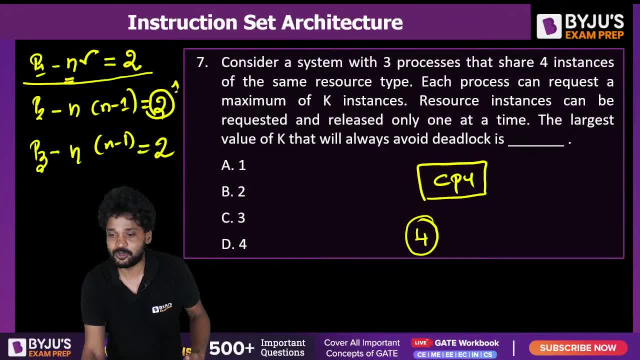 onwards: n minus one, which is two minus one, is equal to one. Which is two minus one is equal to one. Two plus one plus one is equal to four. That the system has already with us With that resource pool. But if let us say it is equal to, 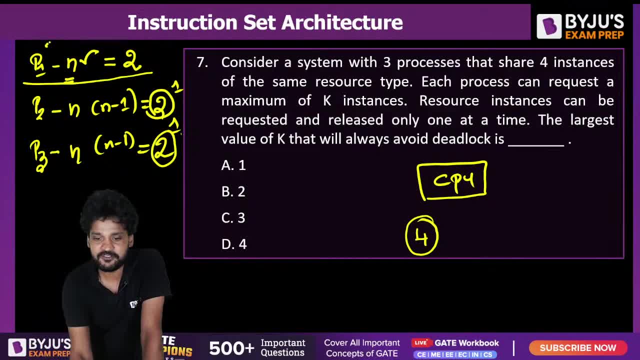 three. Each and every process requesting for three resources At that time system needs to have at least three resources to support the first process, plus two resources to support the second process and two resources to support the third process- Total seven resources If each process is requesting for. 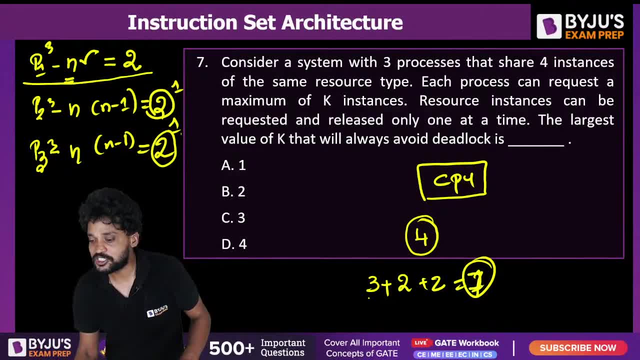 three resources. the total number of resources that the system needs to have is seven, Not less than seven. Otherwise, system will enter into the deadlock state. So did you get it? The maximum number of resources that can be requested by any process is equal to two. 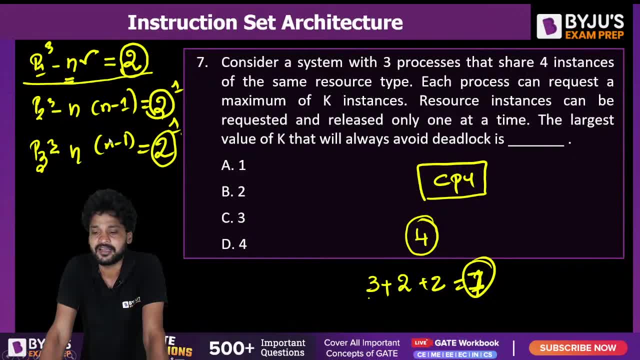 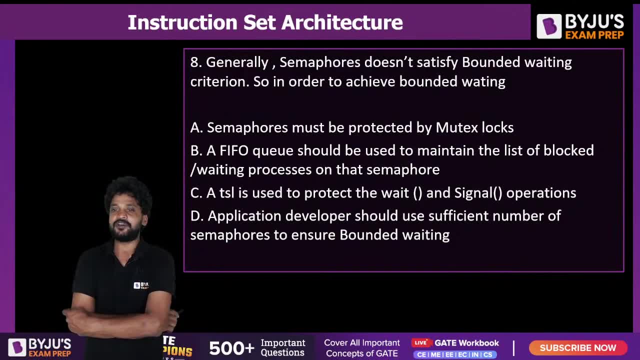 Okay, Neel Madhav, I hope I made it clear, So let me go to the next question. Next question is on your screen. Generally, semaphores doesn't satisfy bounded weighting criterion. Obviously, bounded weighting criterion will not be satisfied by the semaphores. 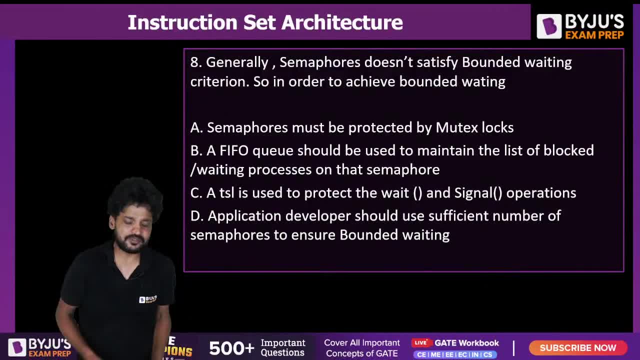 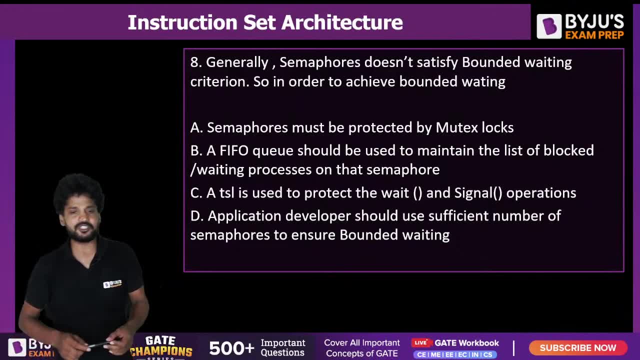 Simple. I told you for several times, no matter how many times I take the semaphore topic, you know I can't say it is a disadvantage. I would tell you that semaphores straight away, by the definition it wouldn't support bounded weighting. 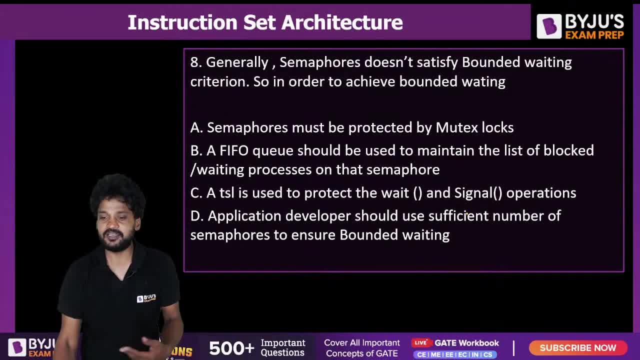 But in the same life. which of the following options are actually correct? Semaphores must be protected by the mutex locks in order to support bounded weighting. A FIFO queue should be used to maintain the list of the blocked and waiting process on the semaphore. 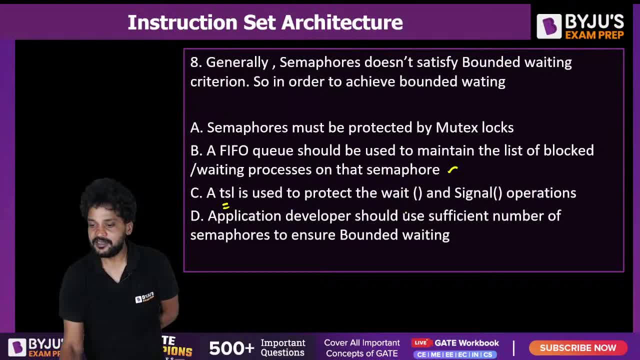 This is the second one. A test and set lock is used to protect the wait and signal operation. This is the third option or statement. Application developer should be able to use the sufficient number of the semaphores to ensure bounded weighting. So, in order to satisfy the bounded weighting, 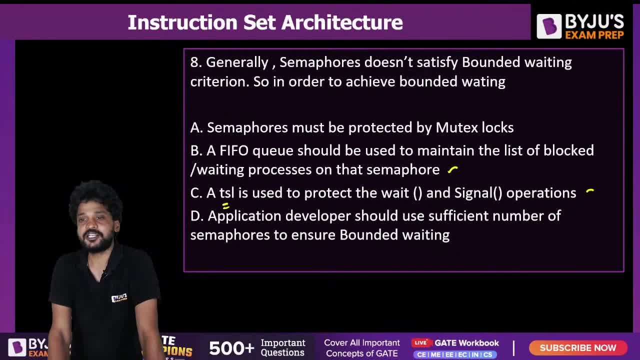 which of the following options are actually correct. Yeah, Sujan Kumar and AB Develis, You are spot on, But you are only half correct. There is one more possible option among the options that are visible. Among the options. 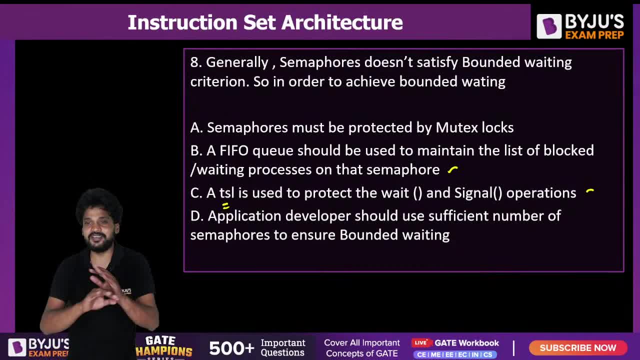 that are on the screen. Option B is, of course, it makes every sense, but there is one more option possible to have the semaphores satisfying the bounded weighting, Of course, simple: The list of the process that are waiting for a semaphore. 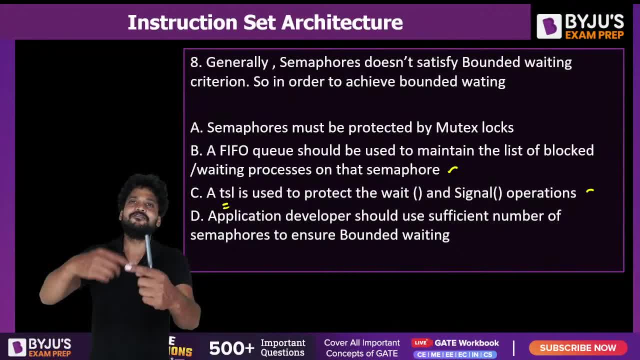 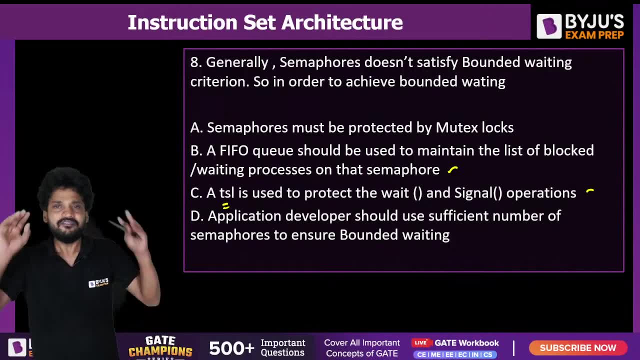 if they are maintained by using a FIFO queue, obviously, one after another, they will enter into the critical section. Obviously, bounded weighting will get satisfied. That is, of course, that every sense will tell you. the B option is correct. AB Develis, very good. 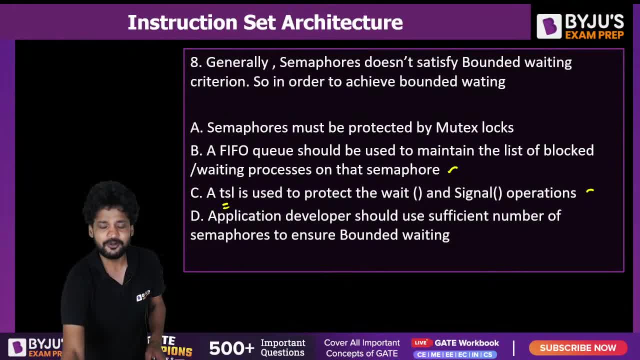 You are spot on. If you actually know how to use the semaphores, you don't even need to maintain a FIFO queue. Tell me one thing: Is there any restriction that critical section can be protected, to be protected by using only one semaphore? 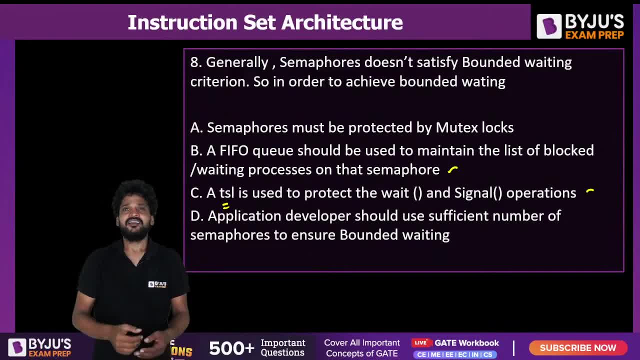 We can declare as many semaphores as we want. right, Yes or no? B and D are the correct options. If you know how to use the semaphores, you can declare many semaphores and by analyzing all the permutations and combinations, you will be able to. 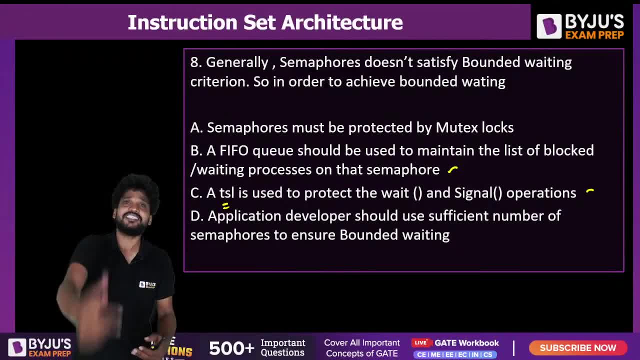 write the code, you will be able to protect the critical section in such a way that bounded weighting also gets satisfied, Yes or no? So option B: this is what I mean. this is what the mistake that we do commit to whenever we give. 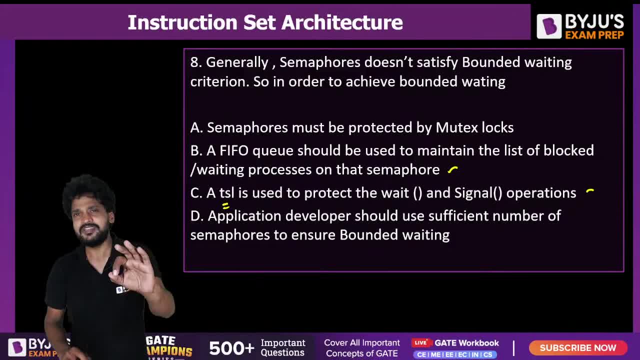 the GATE exam At that time, directly, our answer will: straight away will pull us towards B. straight away is the correct option, But there is sometimes more than one option can be correct right, So you should be able to choose the options wisely. 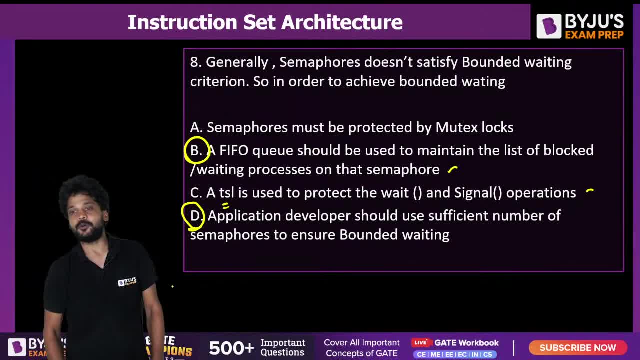 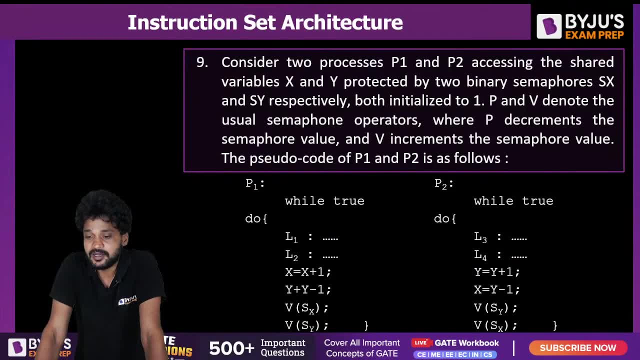 So both B and D are the correct options. Okay And yeah. the next thing is: I do have two questions for you people as homework. Take a snapshot: Question number nine: Question number nine: Yeah, MSQs, yes. 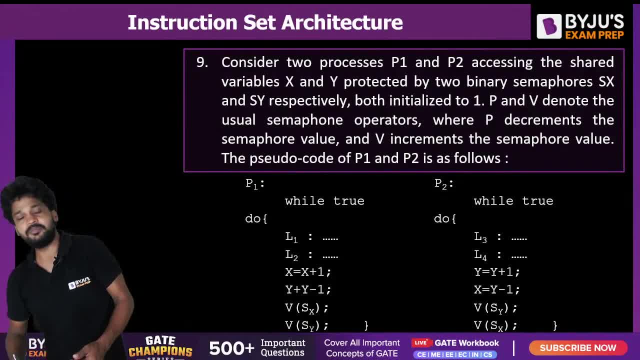 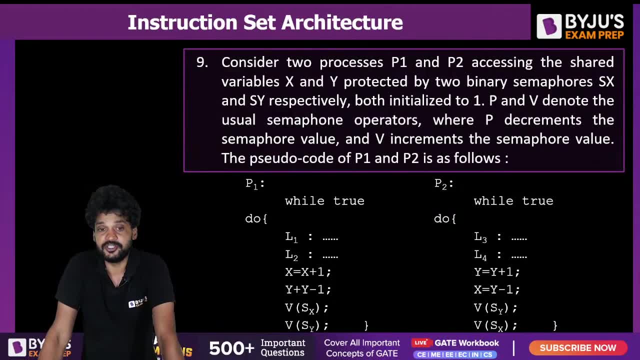 When it comes to the MSQ, more than one option is correct. We should be able to be very careful. We should be very careful while we solve MSQs- okay, Because there may be one option correct in this regard. See: 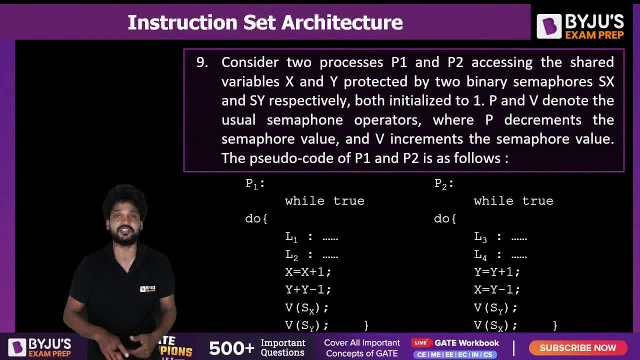 I hope it is making some sense right now how to approach the GATE exam, how to appear for the GATE exam. We do have one concept called MSQs in which more than one option can be correct. Take a snapshot, It is: 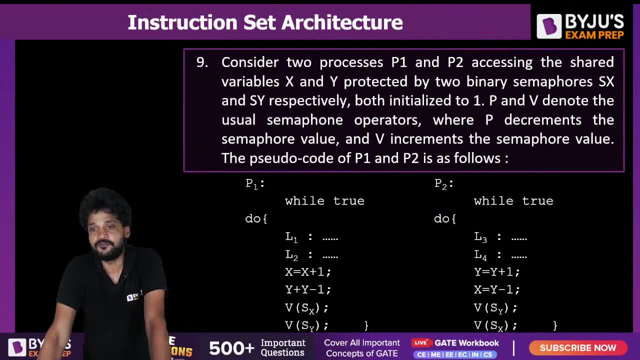 your homework Before I come to the next class. you should be able to finish it And, for those guys who are in my Telegram channel already, I want you people to post the answers within this Telegram group within no time, Right after I finish this class. take no time to. 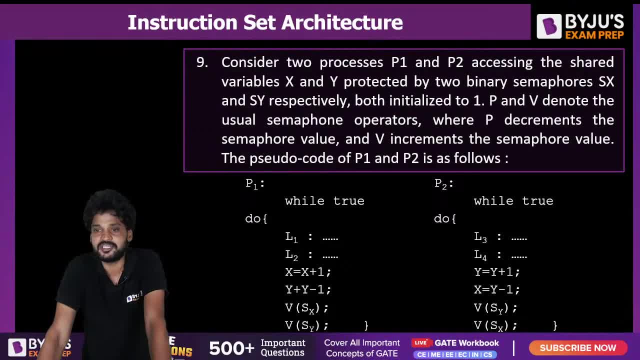 post these answers. Are you done taking the screenshot? Can I go to the next question? Can I go to the next question? What is one more answer? One more question? huh, One more question. So sorry, This is the first. 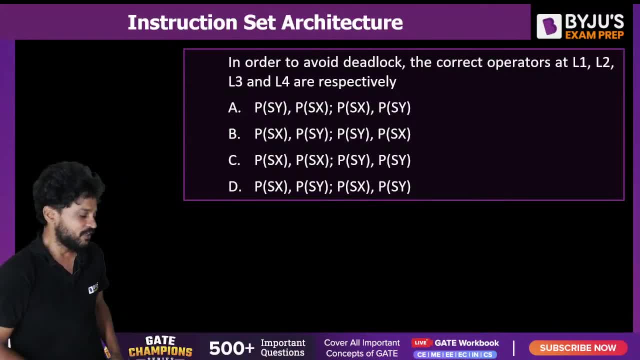 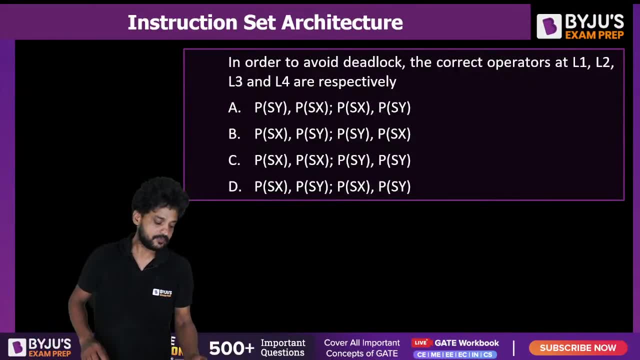 part of the question. This is the second part of the question. The question is given here in this next slide. This is the second part of the question. Actually, this is the data and this is the question on the data. Take the snapshot. 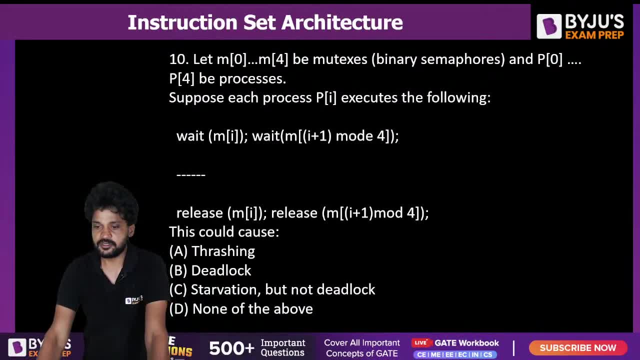 Here. The final question on your screen is the tenth question. I forgot to discuss the previous questions, I guess, so I mean please remind me when we come back. I think on Monday we have the next class. Please remind me to discuss these questions. I just want.